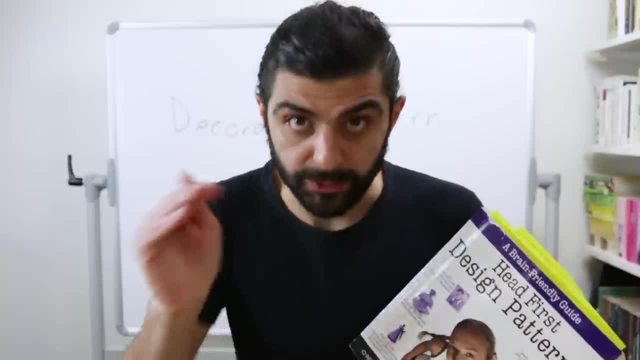 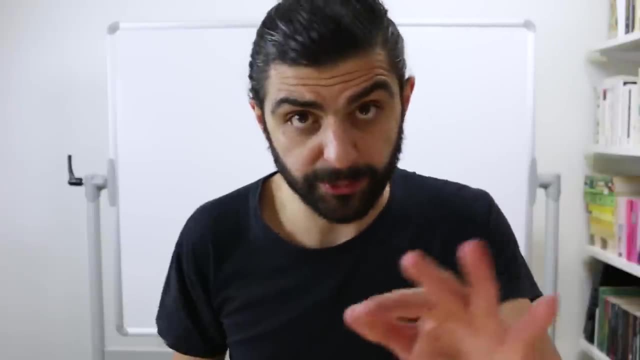 to 14 videos because we'll split some of them into multiple videos. So if you're not already subscribed to the channel, be sure to subscribe to the channel so that you won't miss the next pattern. But now the decorator pattern. So before we go any further, I just want to warn you that the 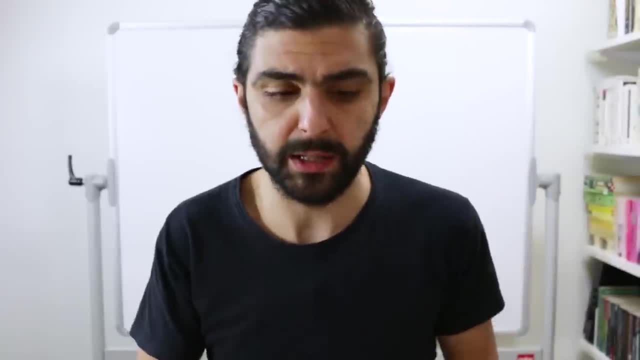 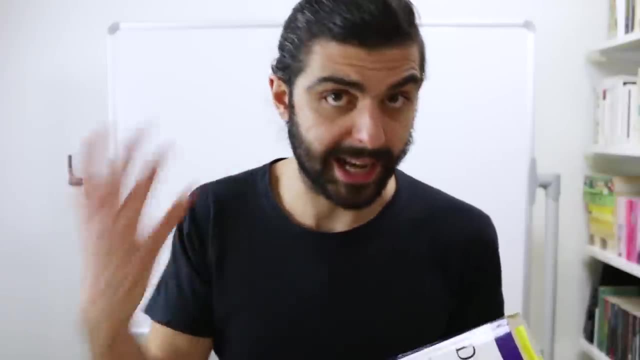 example that's found in the headfirst book is, in my opinion, not really suitable for a decorator pattern. In other words, it's a good example for illustrating how decorator pattern works and how you sort of syntactically string the pieces together. But I don't think, and people are free. 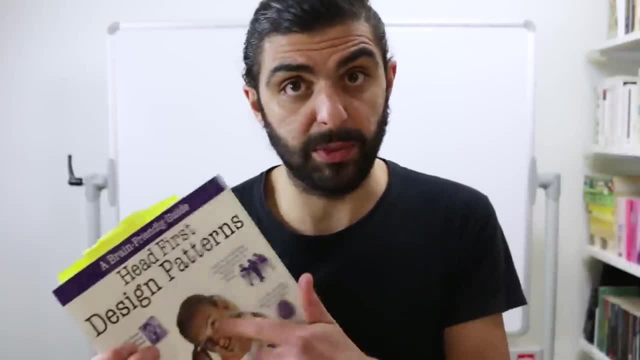 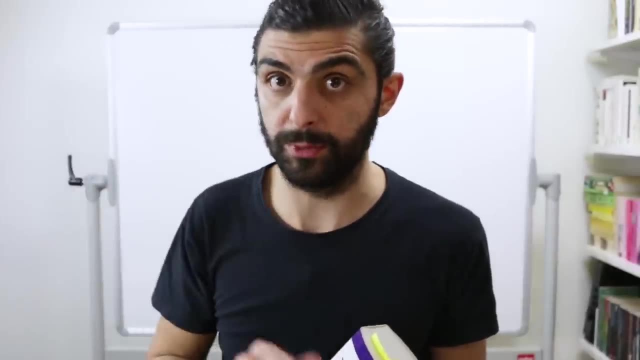 to disagree, but I don't think that it should be taken literally. I don't think that the example that they report is actually a sensible use case for using decorator pattern. We'll return to that, but I just want you to remember that as we go through the example And in the end I'll give you 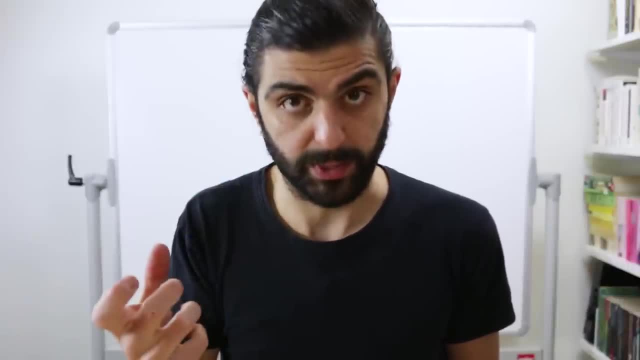 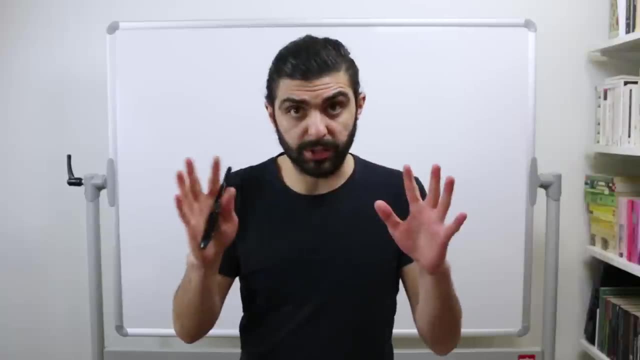 some examples of what I find to be more suitable use cases for decorator pattern and when I've actually used it in real world scenarios while coding myself. But now, what is actually decorator pattern? Let's start on a high level. I think it could be explained in multiple ways, but here are two. So the first one is decorator pattern. 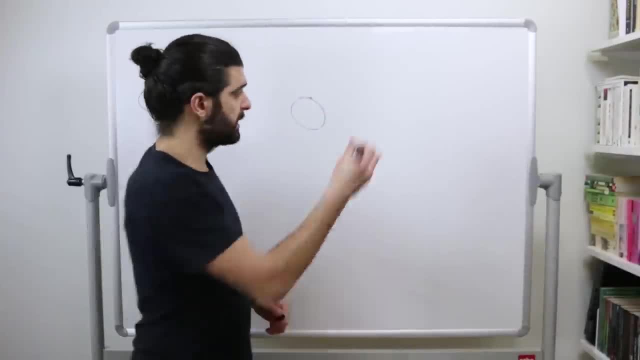 essentially is about you having an object and instead of simply sending messages to this object, this could be speak. You send the message, speak and you expect the object to return, for example, a string back. So you send the message, speak and the object returns. You send the message, speak and 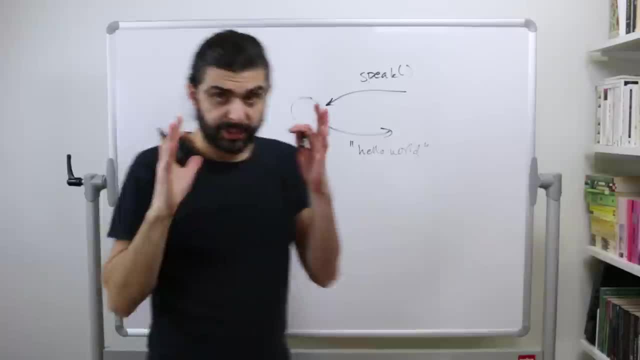 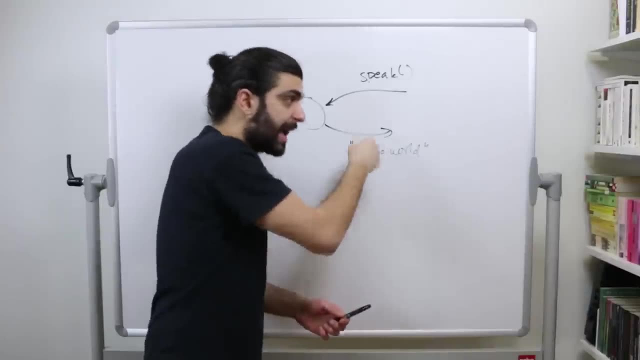 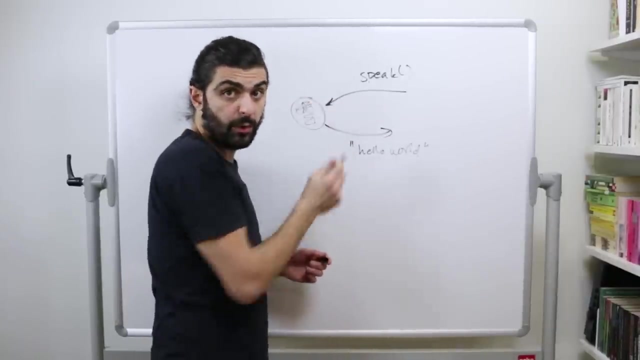 it returns, It responds with the string hello world Now. decorator pattern is a way of saying that if I want to change the thing that's returned, If I want to change the behavior of this method, I could actually do that at runtime without changing the contents of this particular object. So you 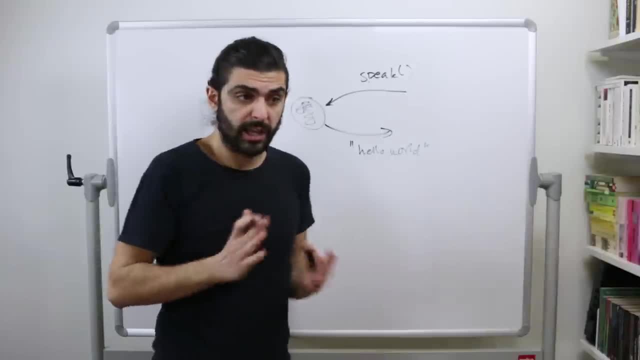 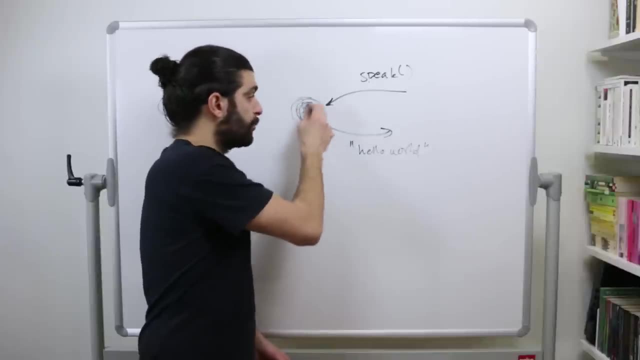 change it at runtime and not at compile time. And when we say change at runtime and not change at compile time, you can simply think of that as changing the behavior of this thing without changing the contents of this thing, without without actually opening up the class and changing the 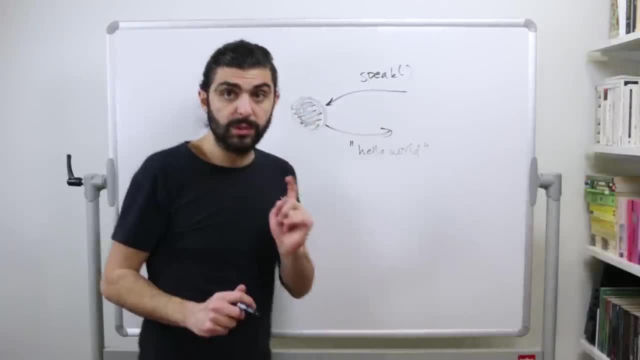 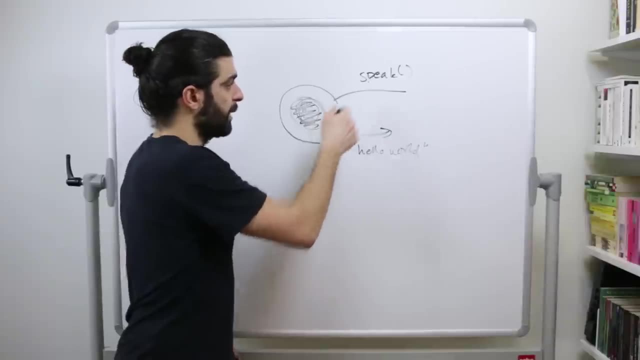 contents of that file. So with decorator pattern, what we do is instead that we say: let's actually wrap this object in another object. I'll remove these arrows and when I send the message speak, I'll send the message to the outer object. who will send the message to the inner object? who? 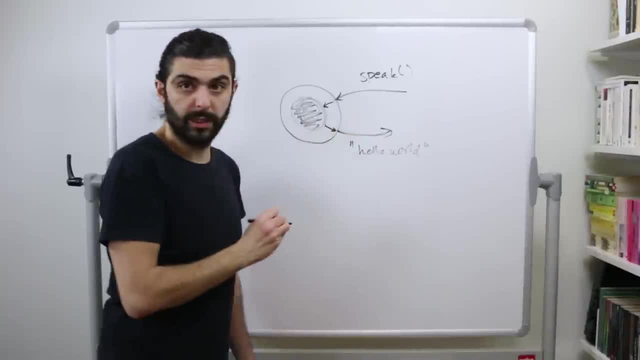 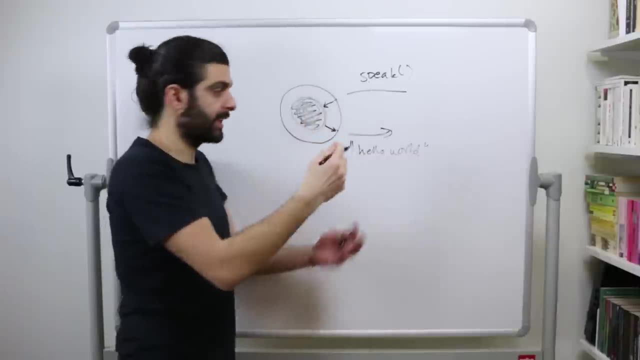 will send the message out back to the outer object, who will return it back to me, And then we can keep on doing this indefinitely. and this is the essence of the decorator pattern. You can take another object, you wrap this wrapped object, you wrap the wrapper in another wrapper, so 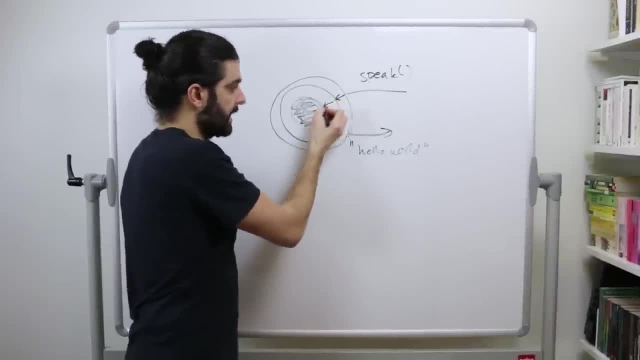 another object that sends the message to the inner wrapper. that sends the message to the inner object, that then returns to the inner wrapper, that returns to the outer wrapper and then returns back to you. So it seems kind of convoluted, but you'll see why this is actually very valuable. So you have. 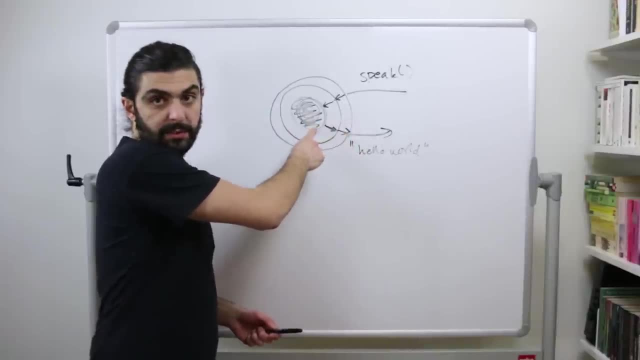 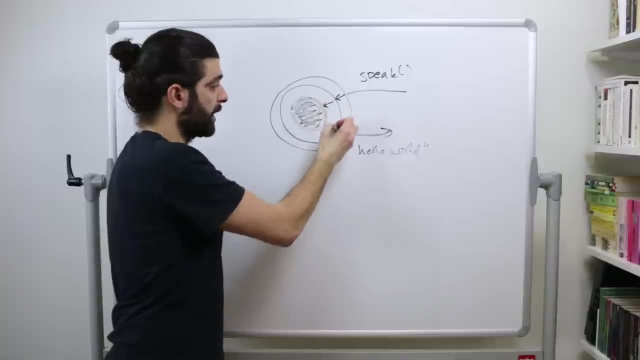 an object that wraps another object that wraps another object. And the point here- let's move to the second explanation- is that so you have the object in the middle, we'll refer to this as the component. but this one, the the one wrapping the component, is a decorator. 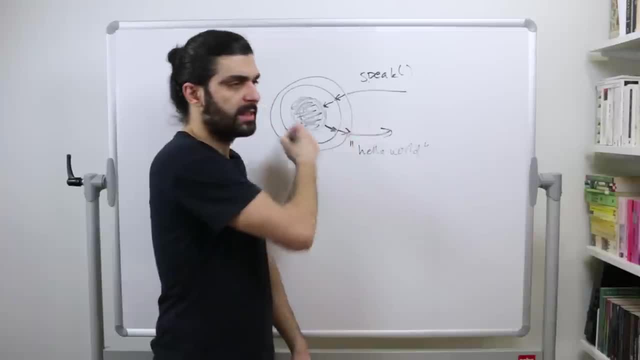 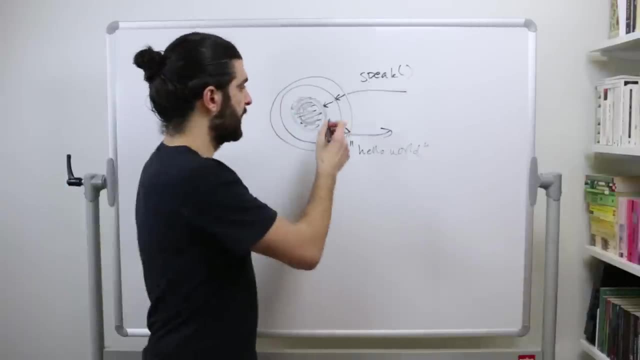 and the one wrapping the decorator is a decorator. If you just think about a single one of these decorators, the decorator has a component and is a component. We're going to get back to this, but essentially remember that from the beginning we said that I take this original object and I want 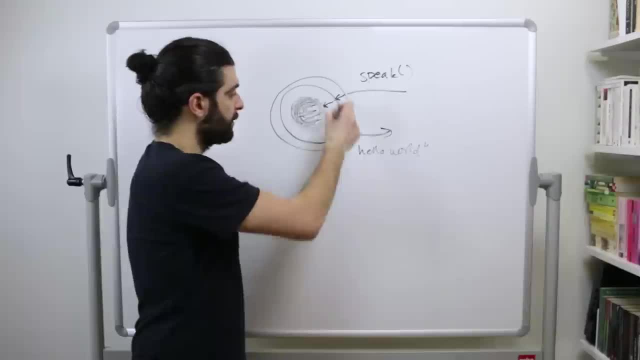 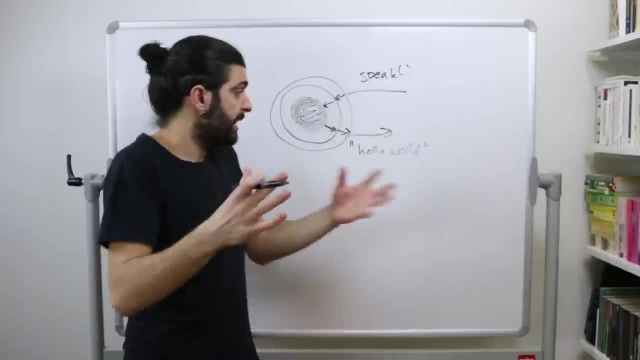 to send the message, speak, and then I'll get something back. And now that we've wrapped it in two decorators, these two decorators actually behave from the outside. from the case standpoint, they are as in isa, they are of the same type as this thing. in other words, they 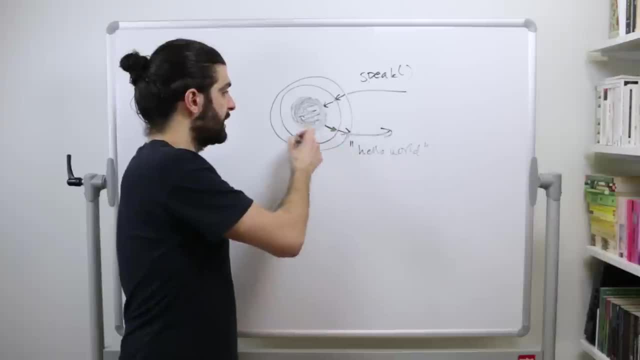 are exchangeable. so whenever you have this thing, you could use this thing instead. or you could use this thing. you wrap the original object and then you can use the wrapper and pass that around as if it was one of these original things. So the first time I heard the sentence it is a and has 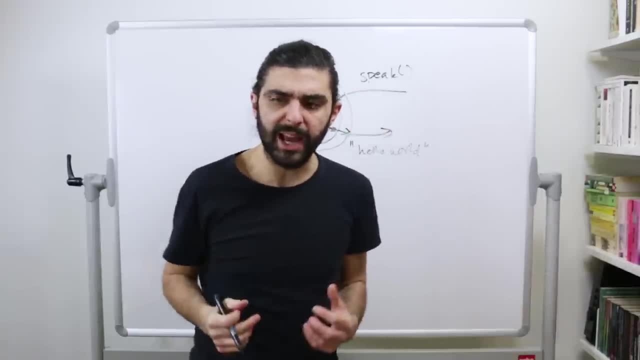 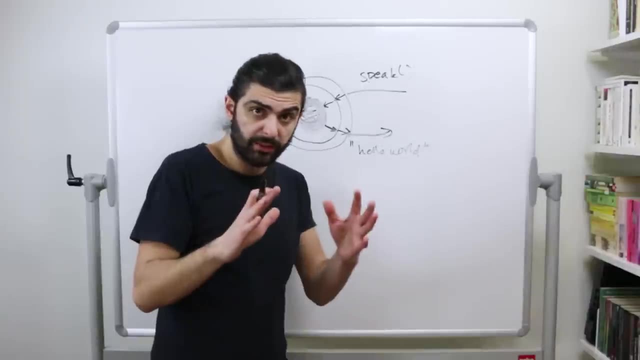 a of the same type. it kind of blew my mind. I'm like what is this crazy pattern? and actually it's kind of cool. it's very similar to composite pattern that we'll talk about later, but composite is significantly more complicated. but you can think of it this way. the decorator is of. 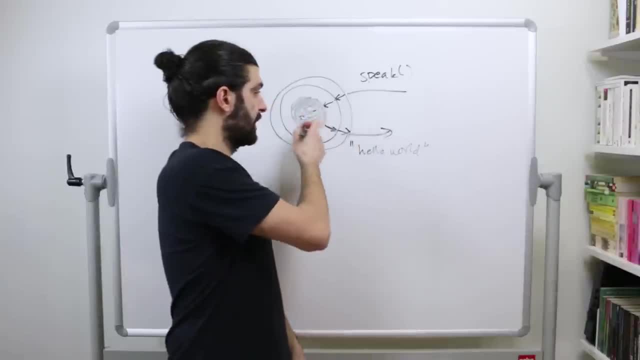 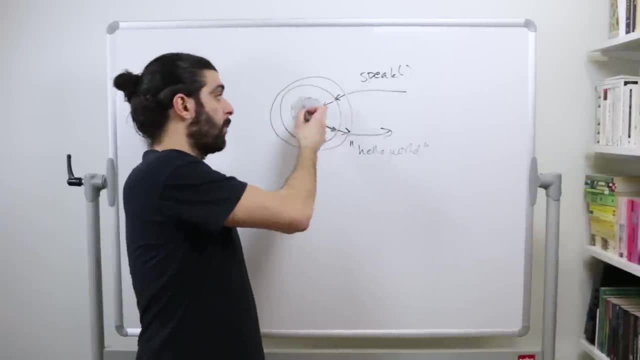 the same type as this because you want to be able to treat it as if it was one of these things that's similar to proxy pattern- that we'll talk about later- and and the has a portion. the fact that it has one of these types is because you want to be able to send the message downwards and then back. 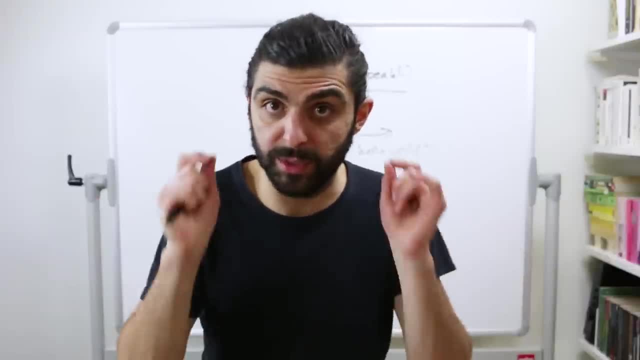 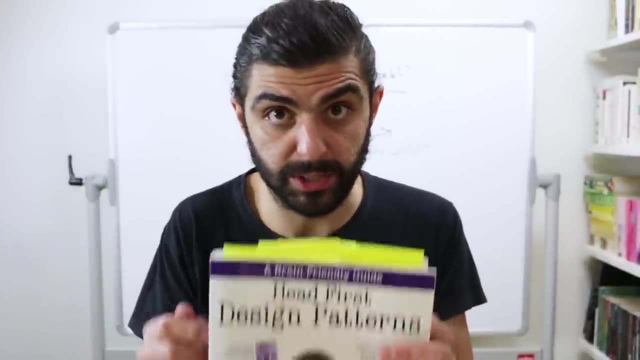 up. that's why it has a but: enough with the abstract nonsense, let's get into something more concrete. so let's look at the definition from the headfirst book. by the way, if you're new to design patterns, I highly recommend you to get this book. the link is in the description. it's an affiliate link, so if you use that link, I'll 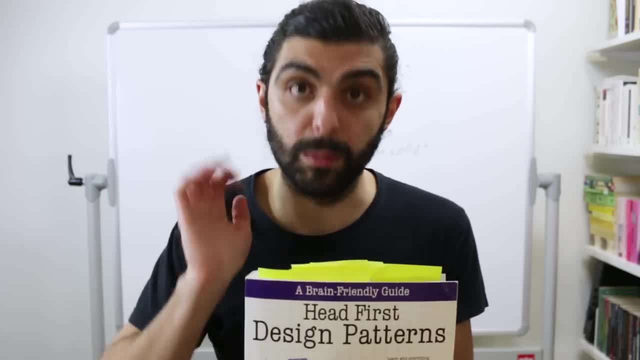 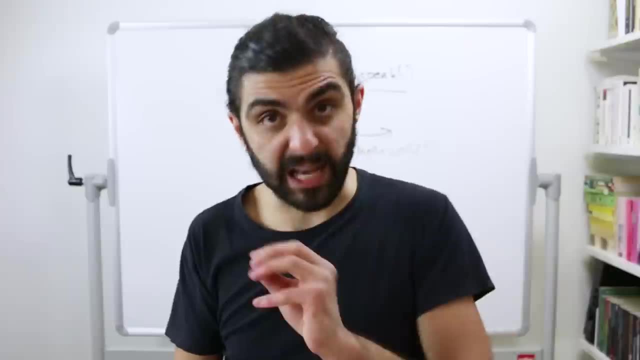 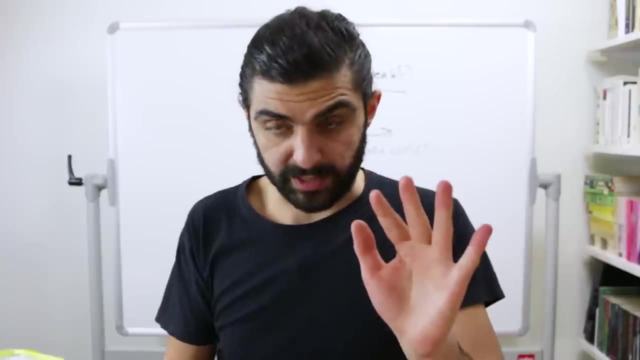 get a kickback and if you do, thank you. that helps massively. but now moving on. so here's what they say. the decorator pattern attaches additional responsibilities to an object dynamically. decorators provide a flexible alternative to subclassing for extending functionality. let's break this down. the decorator pattern attaches additional responsibilities to an object. okay. 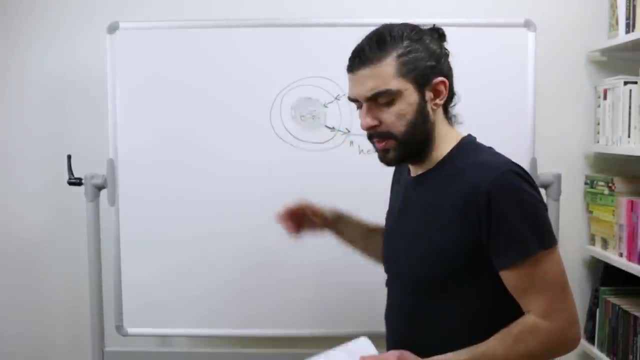 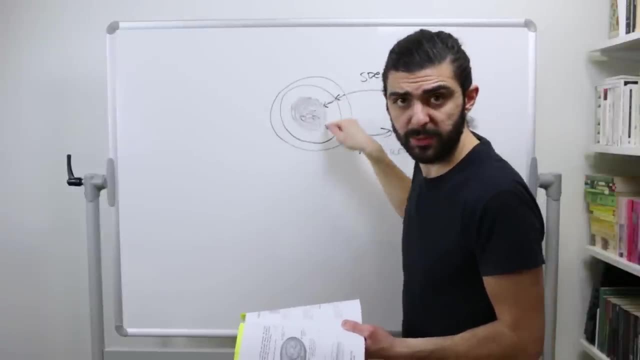 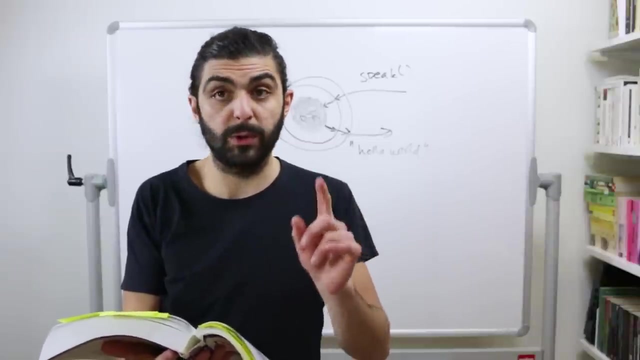 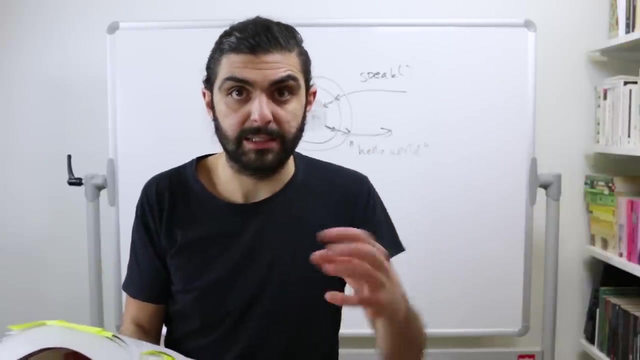 so that means this object was originally doing something, but now, using decorator pattern, we attach additional responsibilities. this outer circle attaches some set of responsibilities and this even outer circle attaches some other responsibilities and, remember, attaches additional responsibilities to an object dynamically, and that's what we're talking about. at runtime or at compile time, you can attach different responsibilities at runtime. 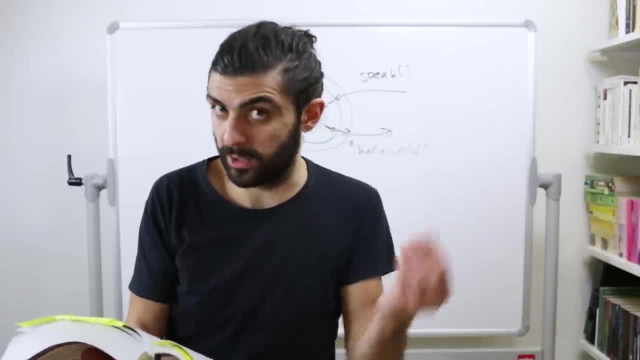 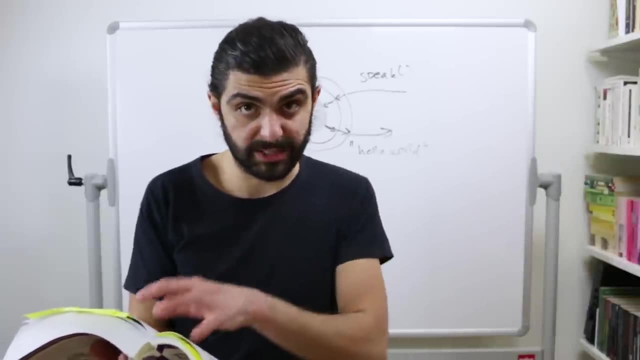 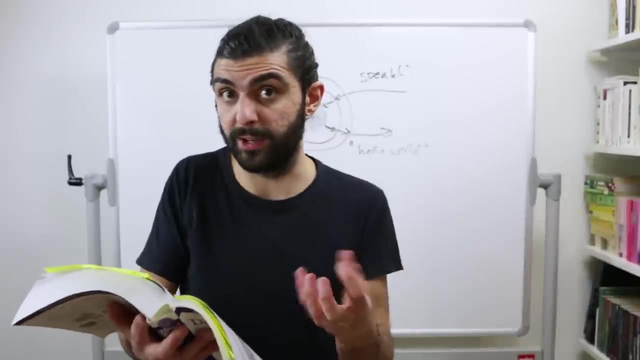 you don't have to set your mind to a particular set of responsibilities at compile time. that's what they mean when they say dynamically. next sentence: decorators provide a flexible alternative to subclassing. we'll actually specifically look at this, because the example that they have of a situation where you might feel that you possibly need something like decorator. 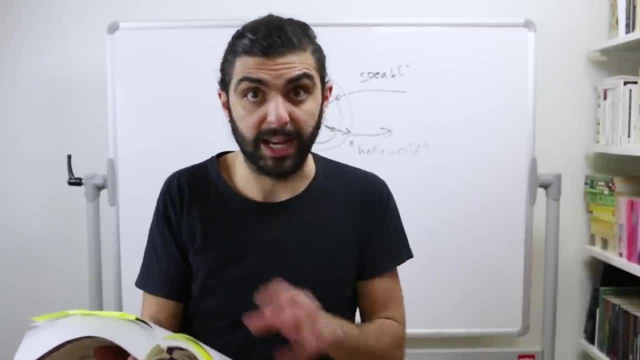 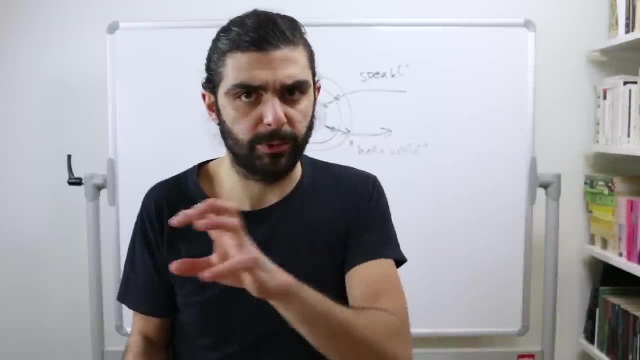 pattern is a class explosion scenario where you have too many subclasses. so you can think of it this way. think about that classical saying: inheritance is not for code reuse, inheritance is not for sharing behavior. so it's a way of using composition rather than inheritance in order to 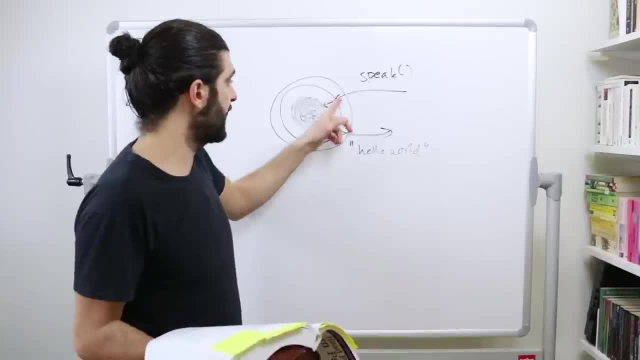 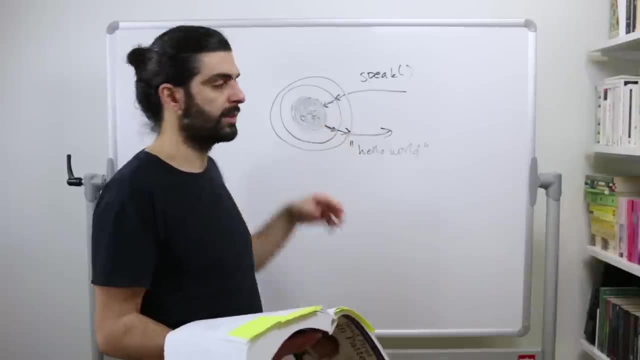 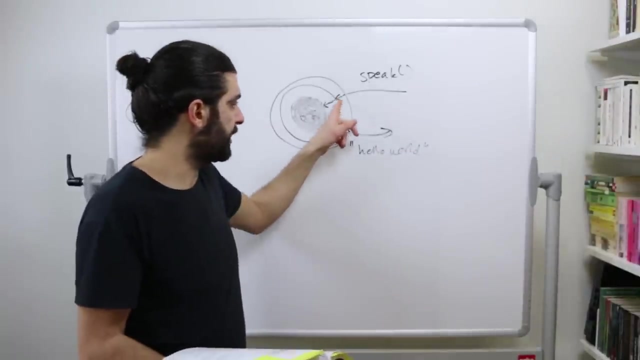 share behavior. remember that what we said before: we use inheritance, we will use isa, but only to to make this thing behave as if it was one of these things. right, we're not using inheritance to share behavior. we're using composition to share behavior. we'll get into this, but we're going to use inheritance to make sure that this thing behaves. 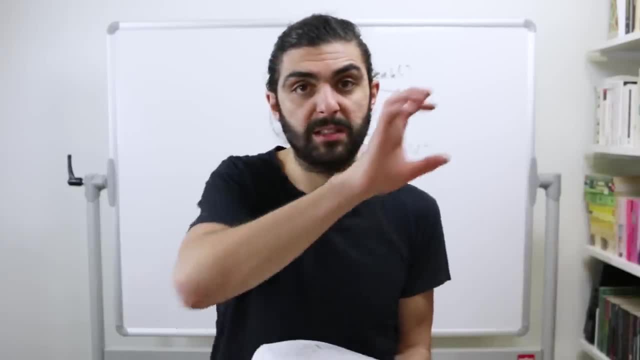 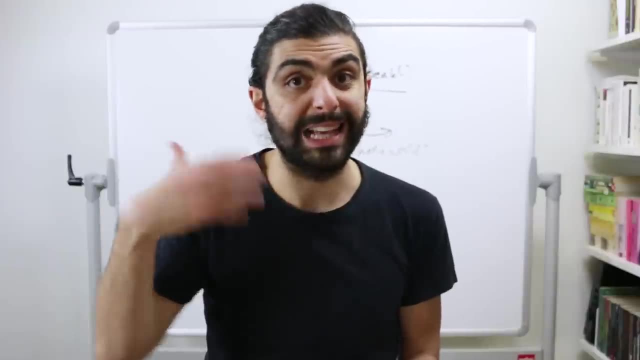 as if it was this inner thing. you can also think of it this way: if you define subclass a, subclass B, subclass C, then you only have ABC. you can't somehow compose a new class at runtime. that's a composition of A and B or B and C. 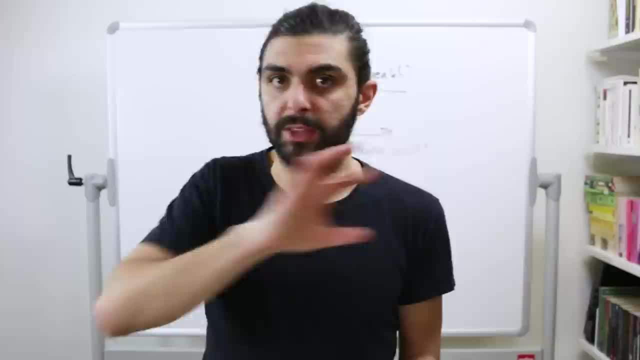 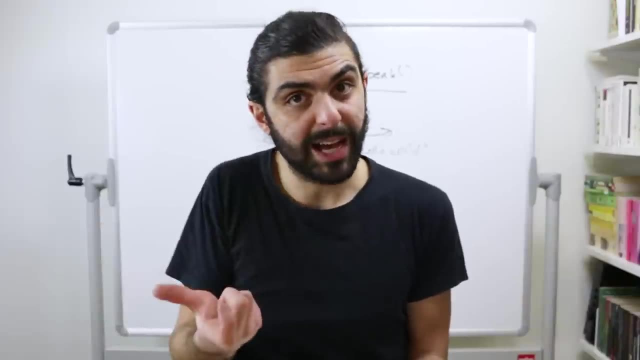 but with decorators, that's actually what we're doing. we're defining the decorator A, the decorator B and the decorator C and then you can actually compose. you can use both decorator A and decorator B at the same time. so it's more flexible, but we'll get into this. so decorators provide a flexible. 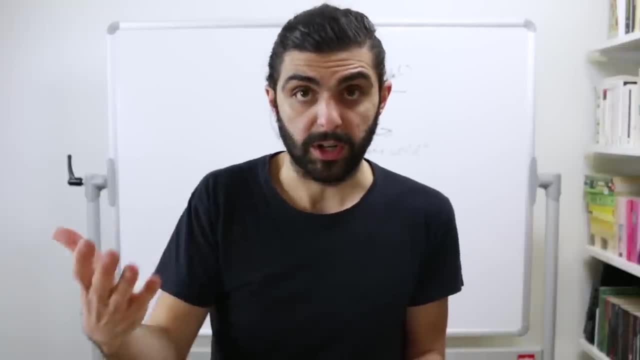 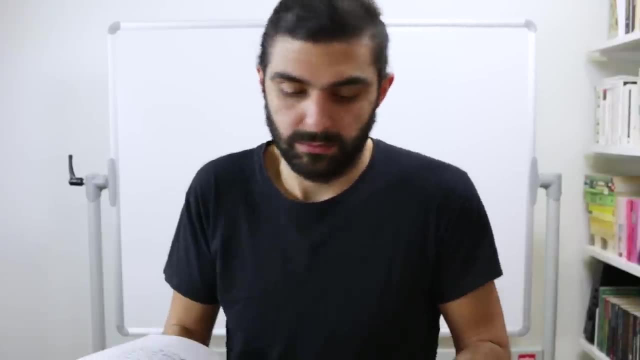 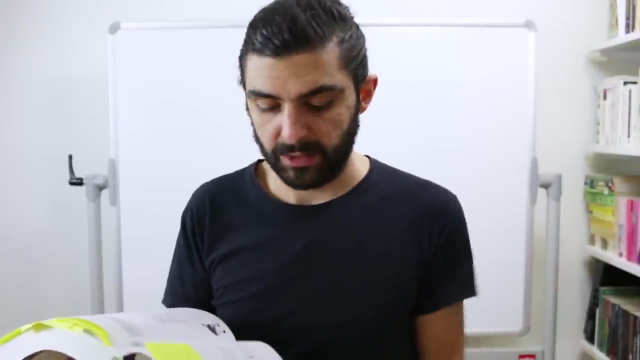 alternative to subclassing for extending functionality, and that's what we were talking about. so that's the definition. in the book they use an example of a coffee house called starbuzz coffee, so essentially it's about constructing a menu of products that can be ordered at the coffee house. so it's a bunch of different coffee types. 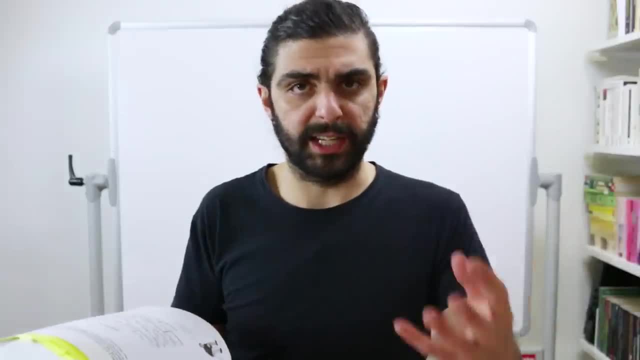 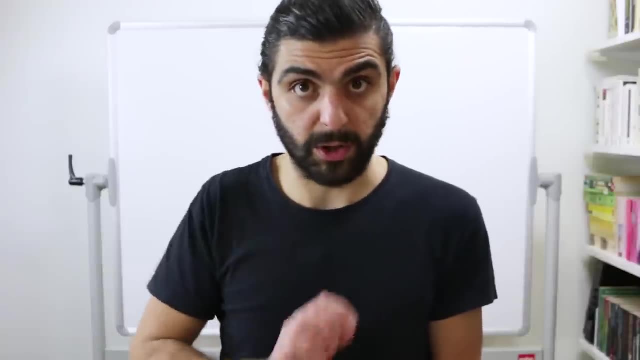 I guess. so a customer comes in and asks for a particular type of coffee, and they have tons and tons of variations of coffee. so here's what they start with. remember that now we're talking about a bad example, so this is not a suggestion of what you should do. this is an illustration of 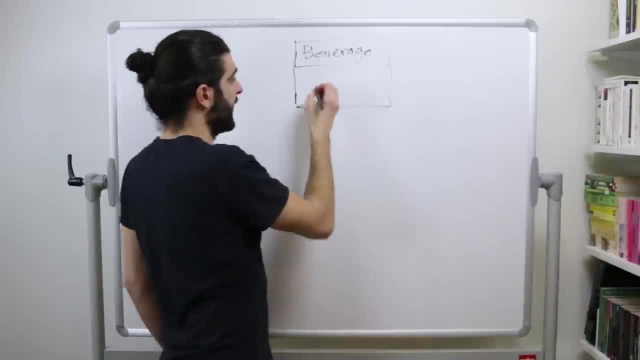 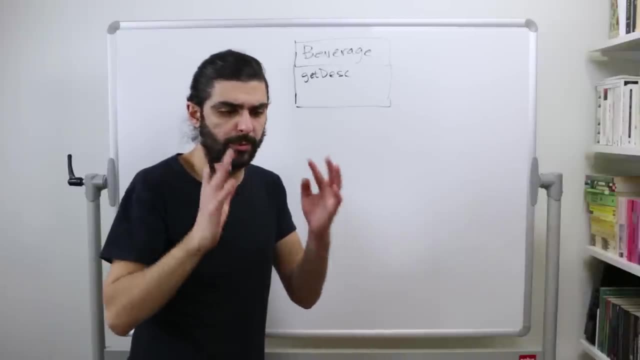 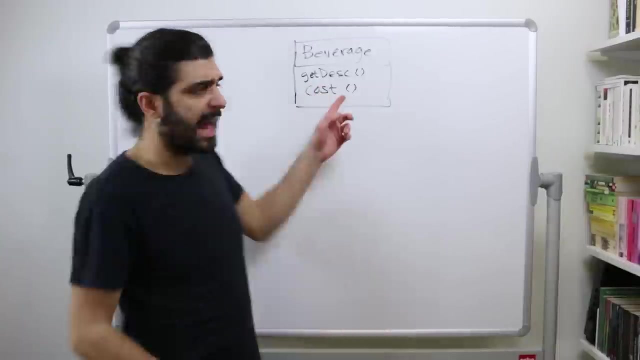 something that's problematic. so they have a class called beverage that has two methods: get description. I'll just write get desk in order to save myself the space. again, remember to always use proper method names and variable names, but just to save space. so get desk for get description. and it has another method called cost and this beverage class is an abstract. 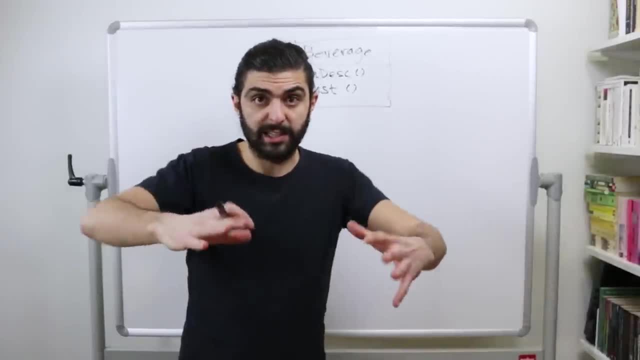 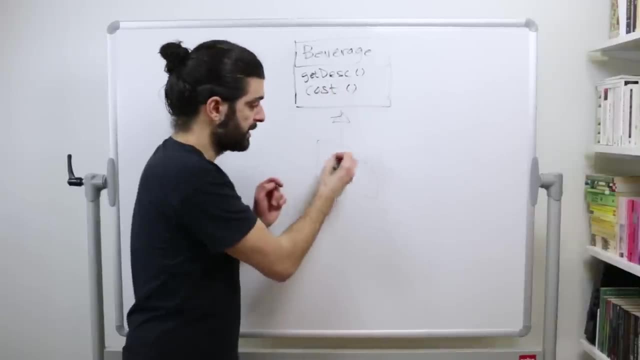 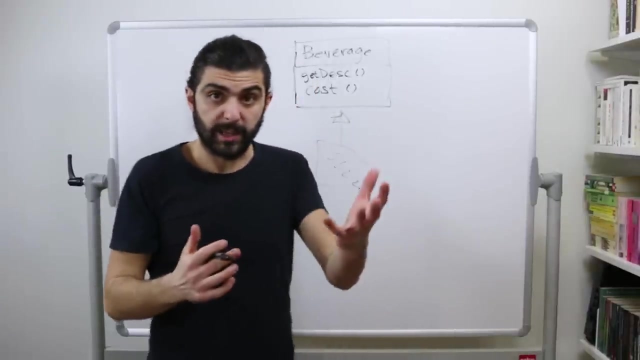 class if you're not familiar with abstract classes. abstract classes are essentially classes that cannot be instantiated. so something has to inherit from beverage and then you can instantiate this thing, but you can never instantiate this thing. the reason for using an abstract class instead of an interface is that an interface cannot have an implementation. 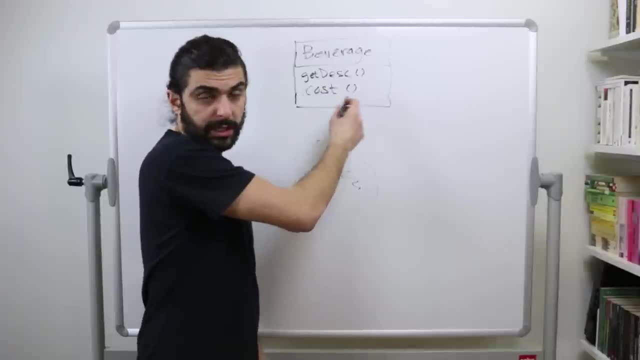 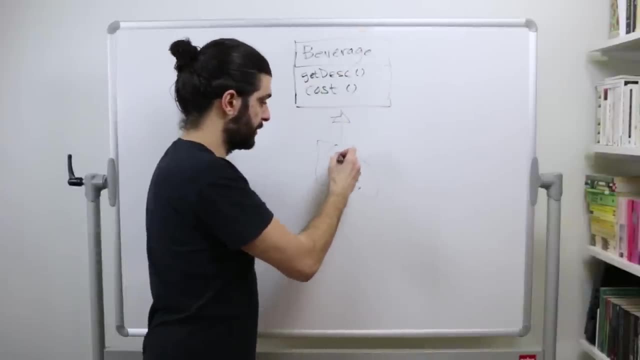 right, you cannot put implementation details in, for example, the cost method. but if you have an abstract class you can actually put a default implementation here in the cost method. but you can't instantiate the beverage. but, however, if you have so here, if you have coffee, for example, then 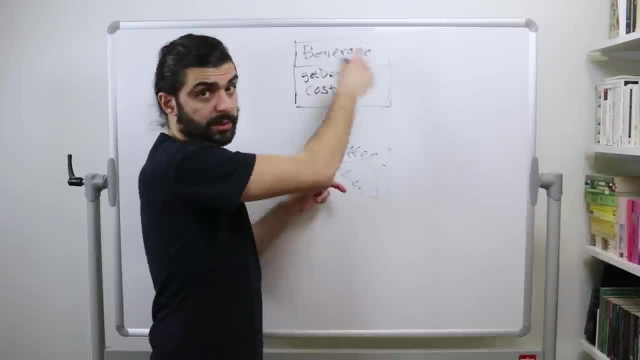 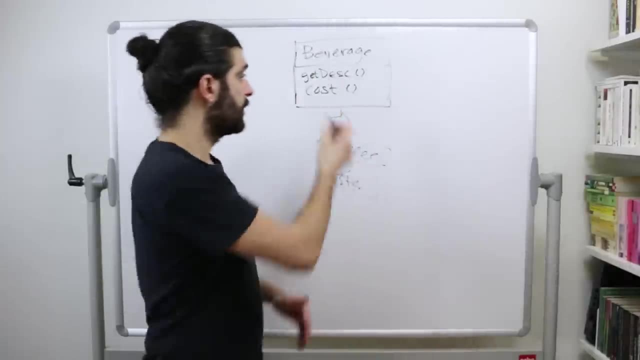 you could instantiate a coffee and if cost has an implementation here in the abstract class, then coffee will get that implementation. for the cost method that wouldn't be possible if you have an interface, because then you would define the existence of a method called cost but you would 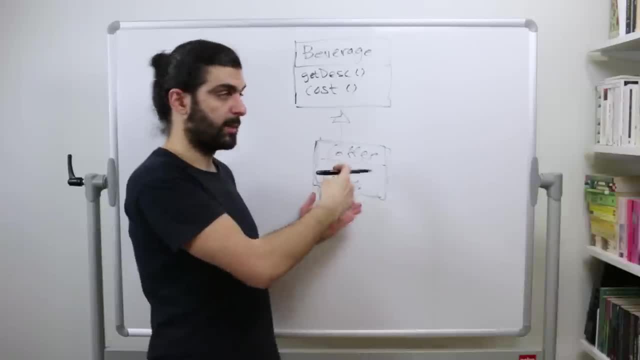 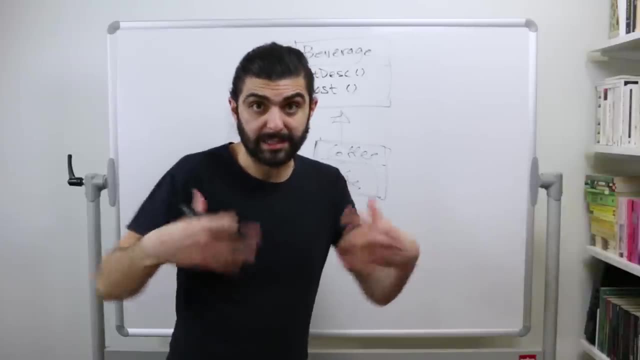 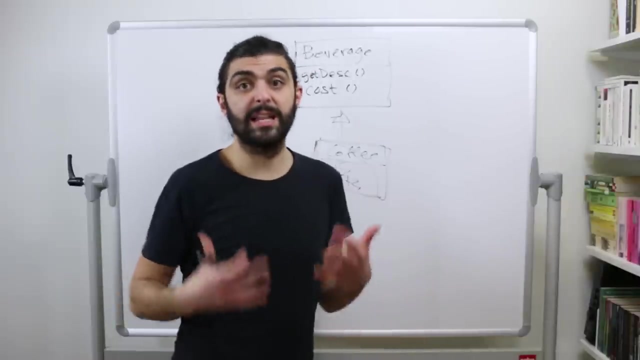 have to define an implementation in the coffee class, so the coffee class is responsible for implementing cost and it can't inherit it from something. so an abstract class is a way of defining a class that defines some baseline implementation or some default behavior that other classes can inherit. but the abstract class is not instantiateable. you can't. 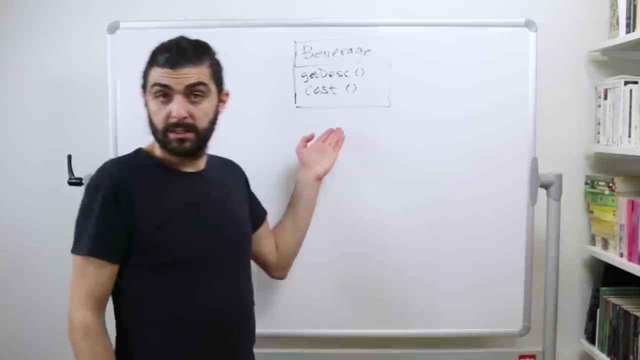 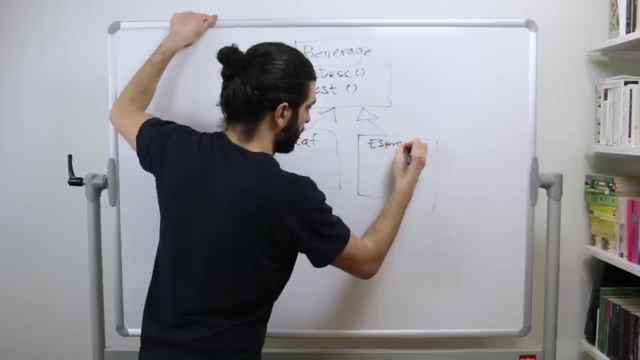 instantiate an instance of the abstract class moving on. so that's the abstract class, and then they have a few basic types of coffee, so they have, for example, decaf and they have espresso, and then they have a few more types, but I mean in order to see if they're going to be able to do a lot of things. 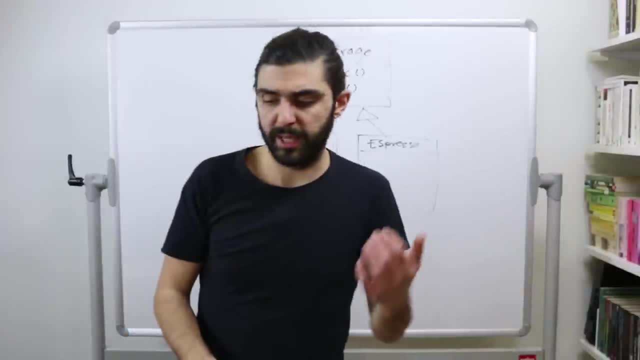 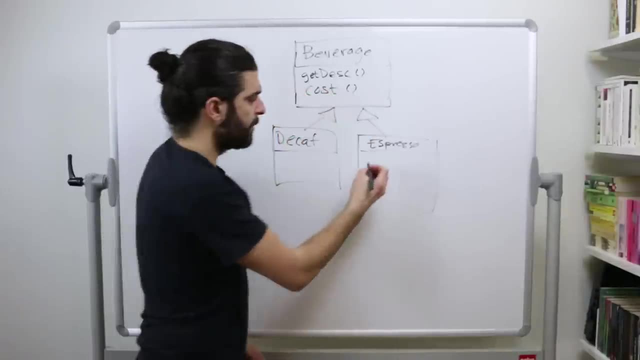 to save space, let's just not consider them. but the other types that they have are house blend and dark roast. but I mean you get the point. you could have a multiple types of coffee that inherits from the, the beverage abstract class and the method that we that they define is cost because the 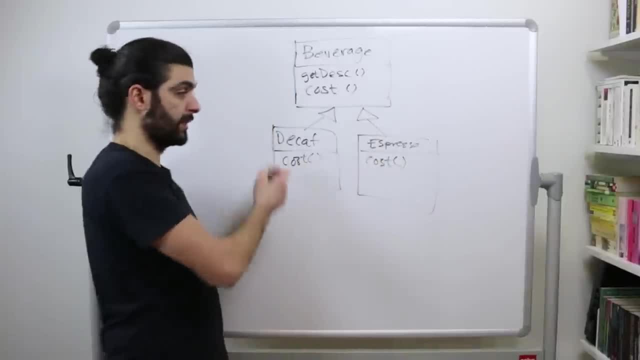 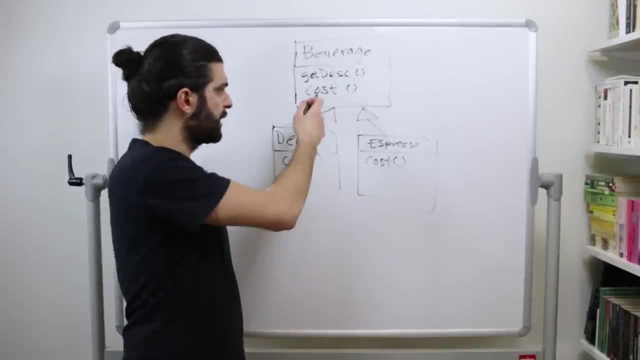 baseline cost of an espresso is different from the baseline cost of a decaf coffee, given the scenario that we're looking at right now. right, so, when I talked about the abstract class before sharing behavior, I think I used the cost method as an example, but what actually happens here is that 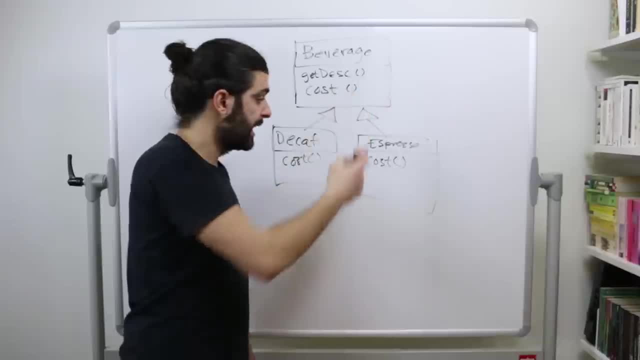 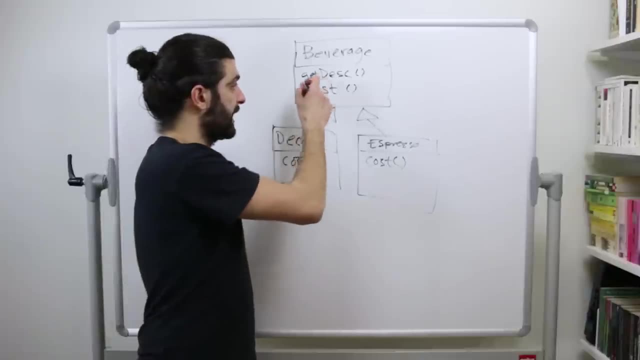 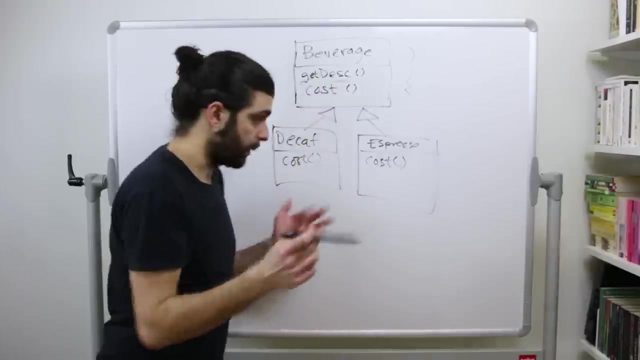 description. that method has a default implementation that is not overridden here or is not implemented here in espresso nor in decaf, which means that the get description method is defined in this class and thus these subclasses will use this implementation. however, cost is probably not defined here, or you? 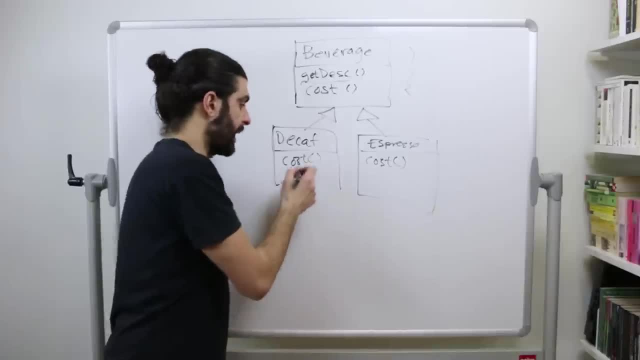 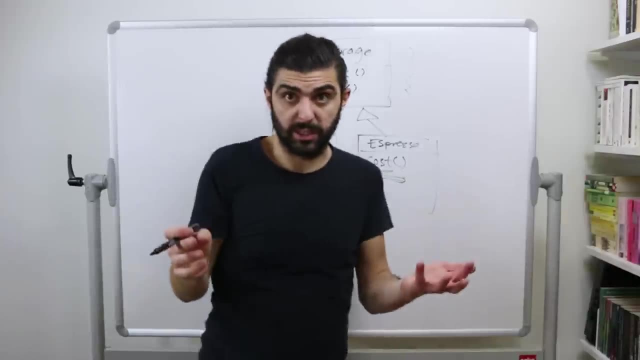 could have a default implementation here. but regardless it's possible to override here in decaf and here in espresso. so decaf has some cost and espresso has some other cost which could potentially be the same or potentially not, but, given the example, probably not the same. so the 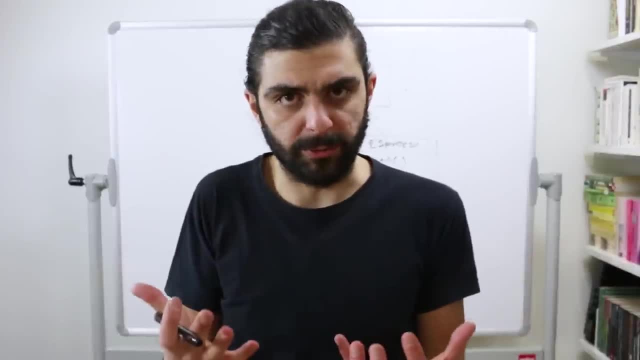 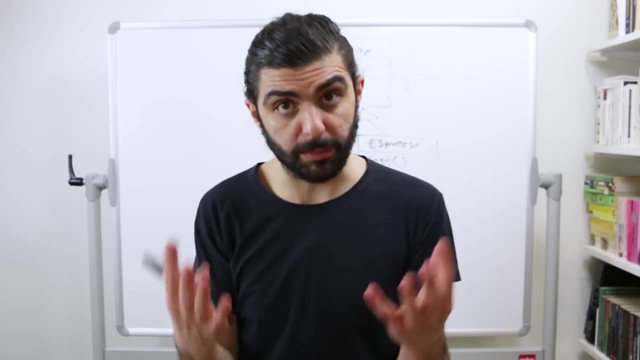 point here is that they have these sort of base kinds of coffee, but then the crux is that they have a bunch of extras that you can get with your coffee or in your coffee, which they in the book later call condiments. but you can think of them as extras or as flavors or as toppings or as spicings. 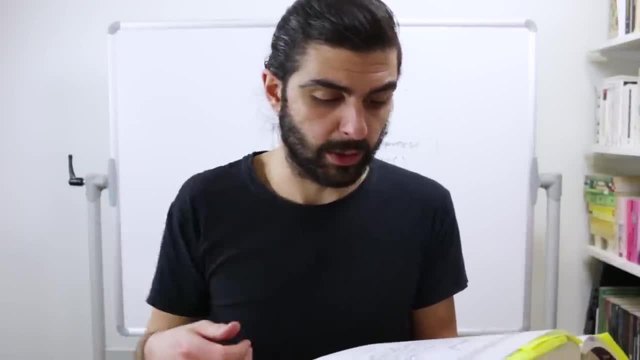 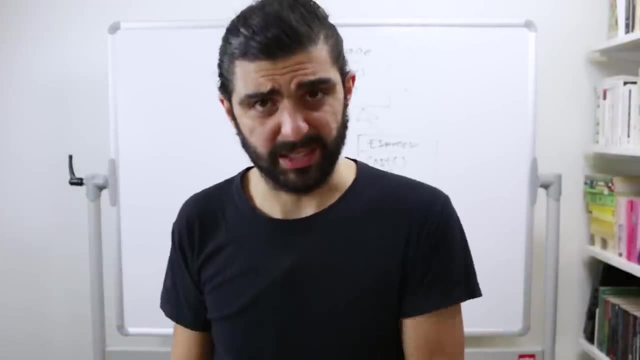 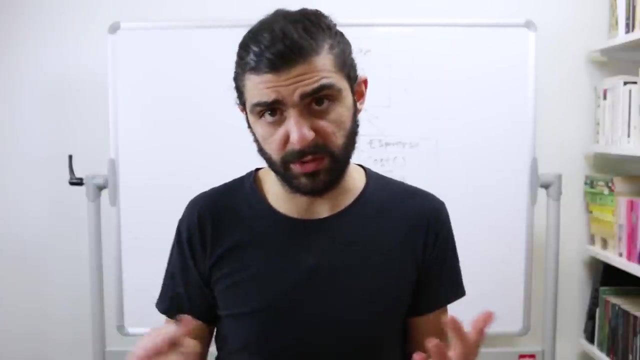 so, to be more specific, these are things such as steamed milk, whipped milk, mocha, soy milk, Etc. Etc, Etc. this is also the first point where I feel that their example is- apologies, but kind of stupid, because who would ever then think that it's a reasonable idea to start to introduce a single? 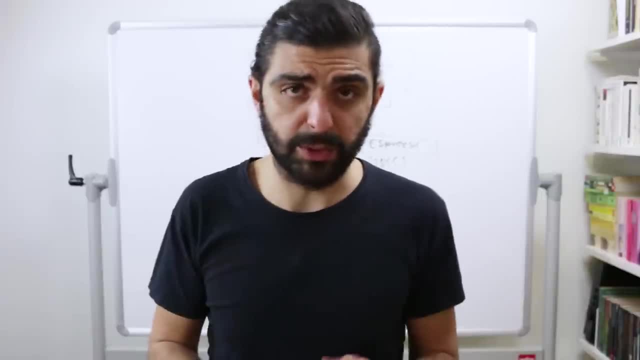 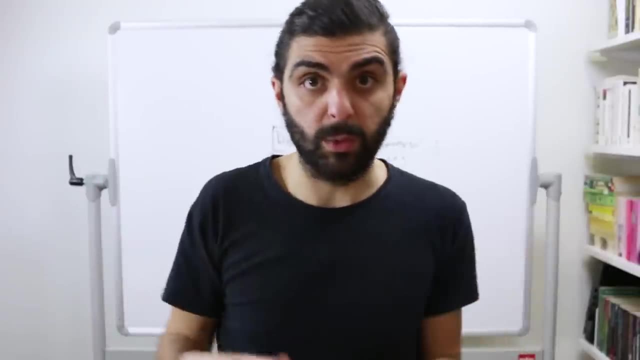 class for each combination of these different things, because the problem that they're pointing towards is, of course, that you could have both a mocha coffee with steamed milk, but you could also have a mocha coffee with whipped milk, or you could have a mocha coffee with soy milk, or, if you think, 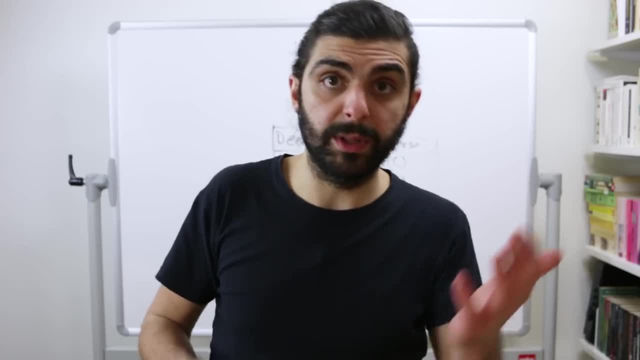 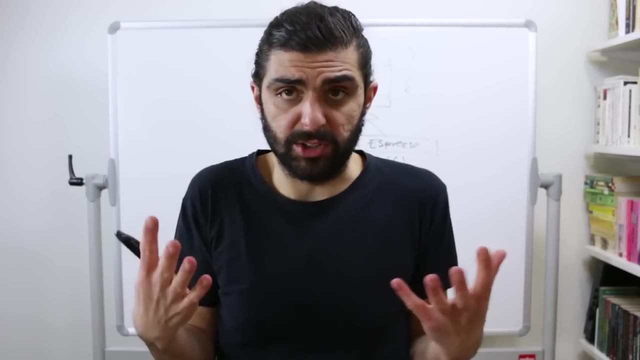 about the flavor caramel. then you can have a soy milk with caramel or whipped milk and caramel, Etc, Etc, Etc. like if you define a few of these different flavors and then just imagine that any flavor could be combined with any other flavor, because why not? I mean, people could come up with the. 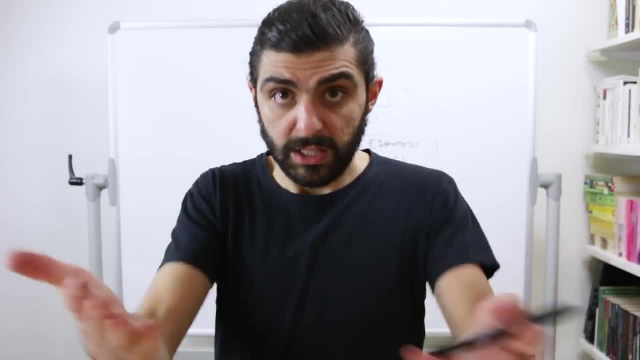 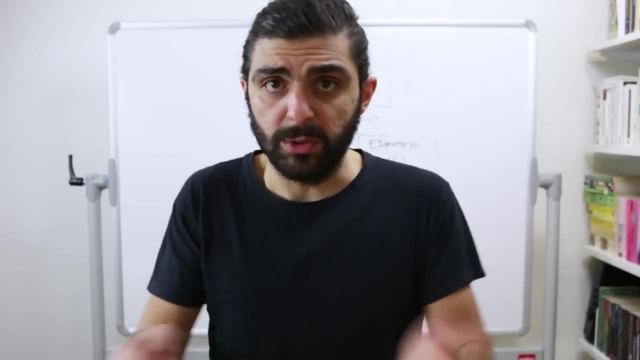 strangest orders, which makes sense. if you're a coffee house, right, you want to actually serve the people who want you to mix different things. just think about if you've ever been to Starbucks or espresso house or any of these places. I mean, of course you can get crazy combinations of the. 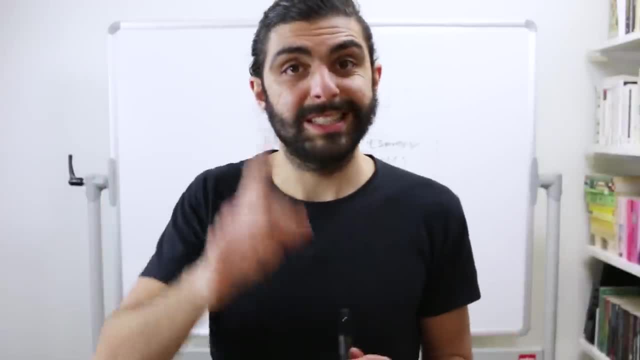 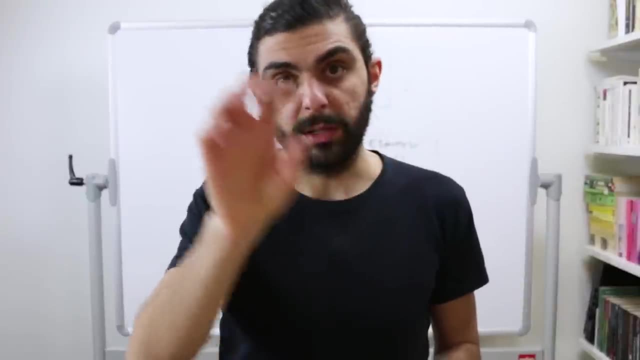 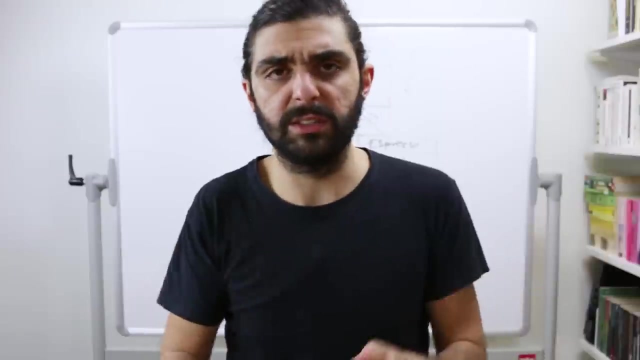 toppings or the extras that they have. and if you introduce a single class for each combination of these different flavors, what you get is this: a mocha coffee with steamed milk, caramel, whipped milk, caramel, Etc, Etc, Etc. If the first one is a class, the second one is a class, the third one is a class each and 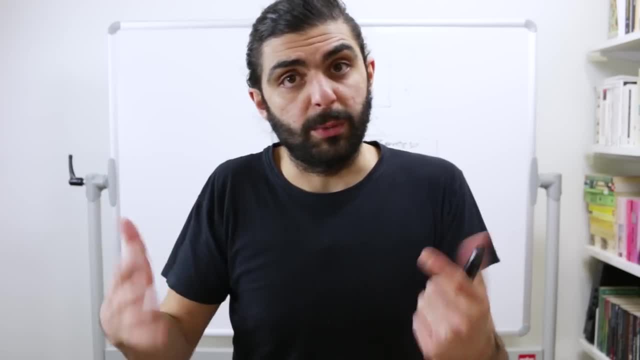 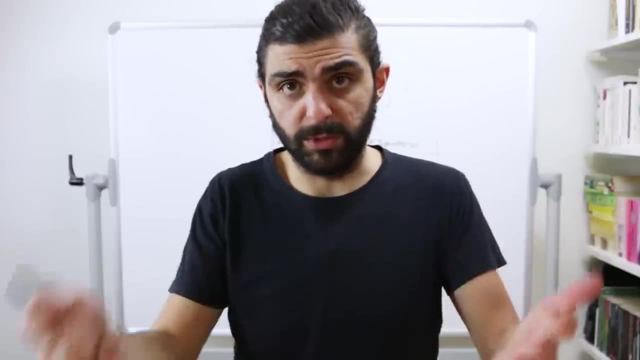 all of these are different classes, then you'll have what is commonly referred to as a class explosion. you'll very quickly find yourself in a scenario where you have tons and tons of classes and they all do very, very small things right. so, from single responsibility, principles, point of 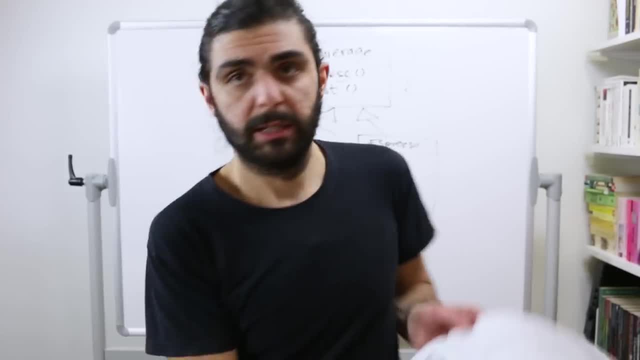 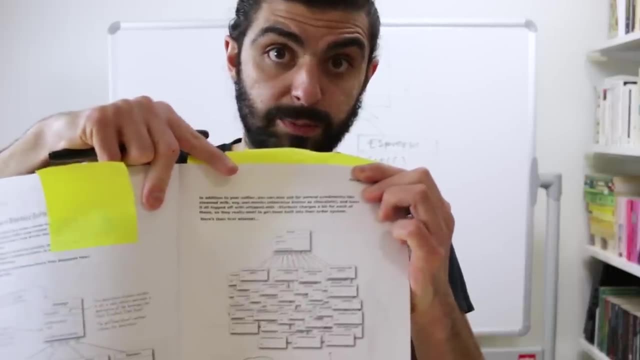 view. maybe that's a good thing, because they do only a very small thing, but it's completely unmanageable me actually drawing this here. Let me just show you this picture and I think you'll understand what I'm saying. So a serious class explosion. So that's an example of a poor way of approaching 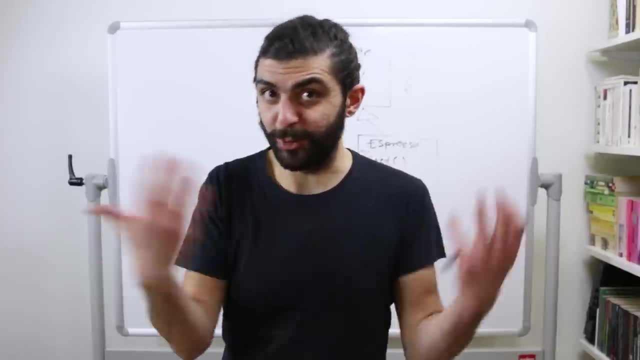 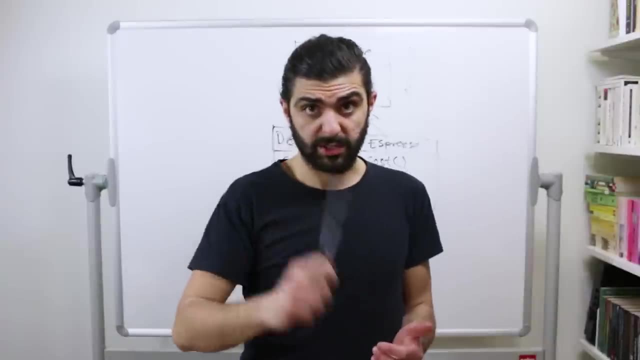 this problem. So then they suggest another poor way of approaching this problem that might also actually be intuitive to a lot of people, especially when you're new to programming. So the second suggestion that they have is to say that all of these different things 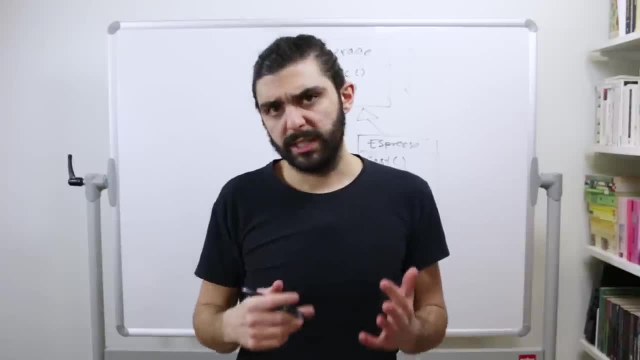 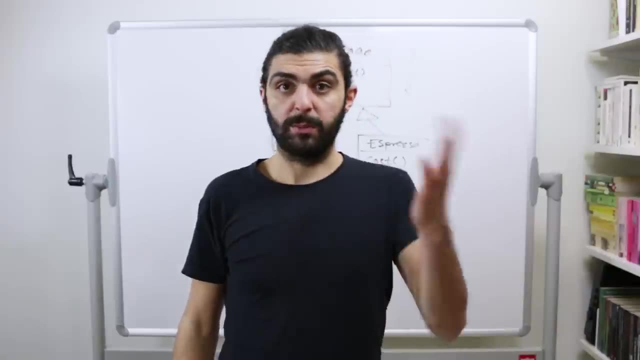 like whipped milk, soy milk, caramel, et cetera, could be treated as booleans, could be treated as true or false values. So the concept of having steamed milk could be treated as a boolean where if you put steamed milk into the coffee, how steamed the milk is true. 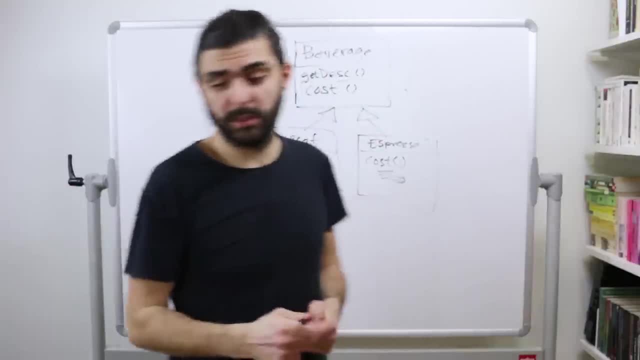 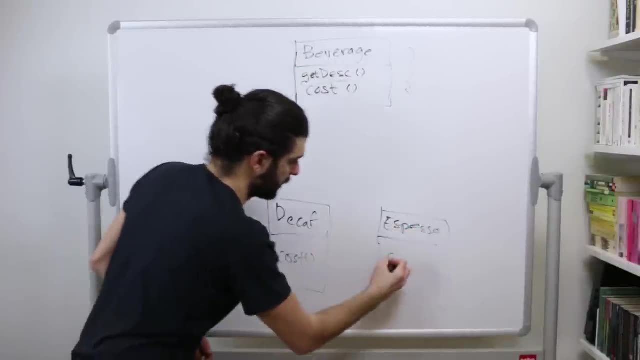 If you don't, then it's false. That's kind of simple right. So you just enumerate all of the different things So, which means that we need some more space here. So we had decaf and espresso, both having the cost method and both inheriting from beverage, And then 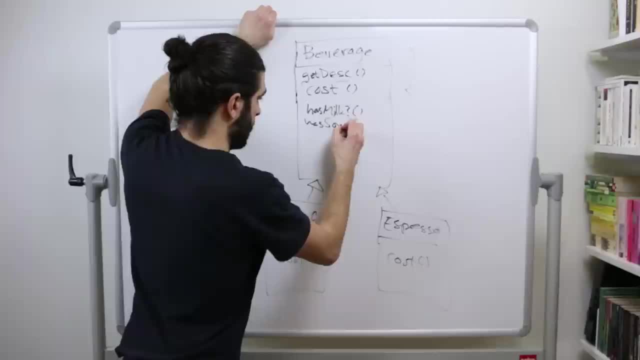 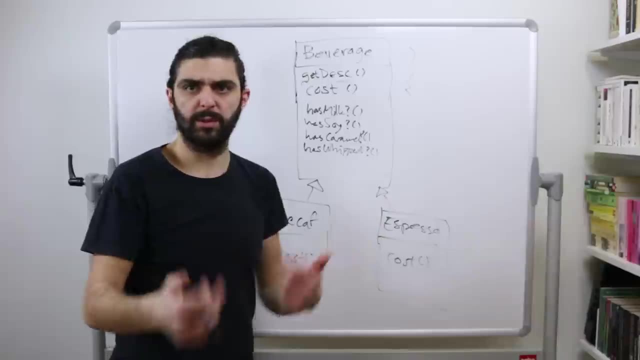 in beverage. we put all of these booleans So has milk, has soy, has caramel, has water, whipped and so forth and so forth and so forth, And actually whipped was probably whipped cream rather than whipped milk, but whatever. And actually because of the examples in the 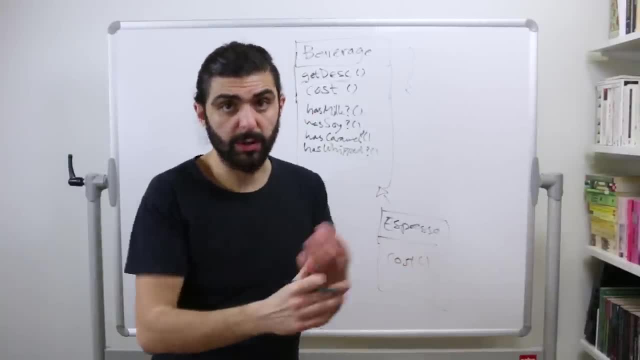 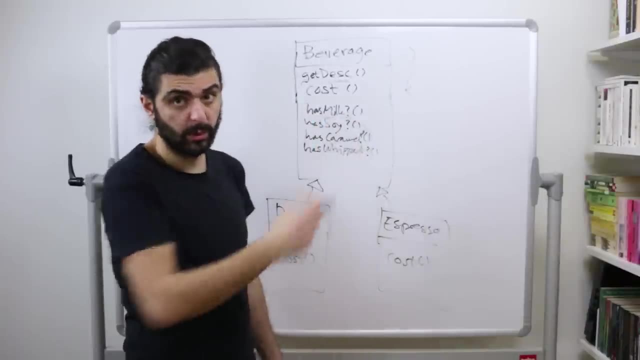 book are in Java. they're not using getters and setters that you have in C sharp. So these would correspond to getters, but they also in the book define setters. So you don't only have has milk, you also have set milk. So you say set milk which sets milk to true. 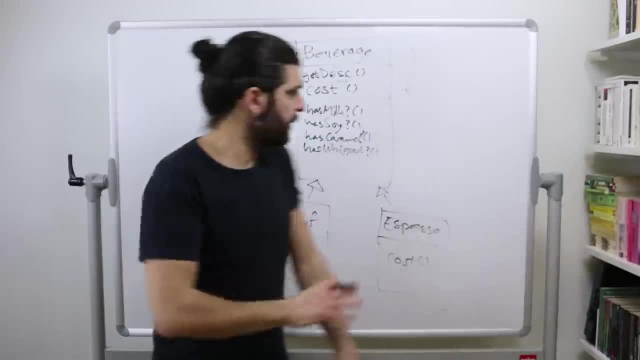 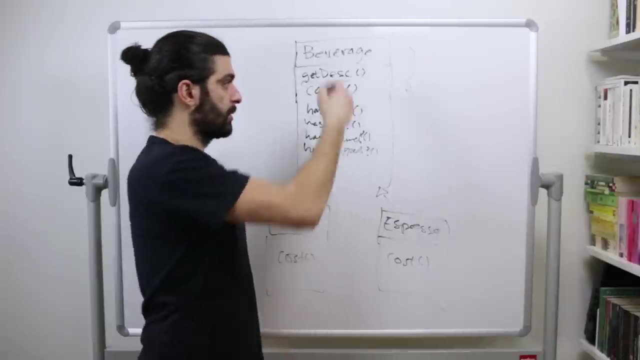 or you say: set milk and pass a boolean, so setting it to true or false. But I mean that's irrelevant to this example. Of course you could also pass these through the constructor, for example right. So on creation of a beverage, you supply 1,, 2,, 3, 4 booleans. So true for milk, false. 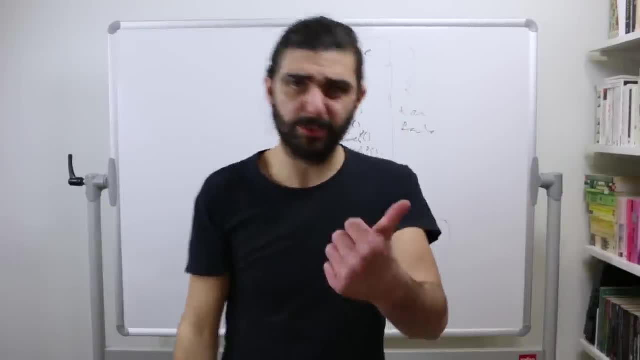 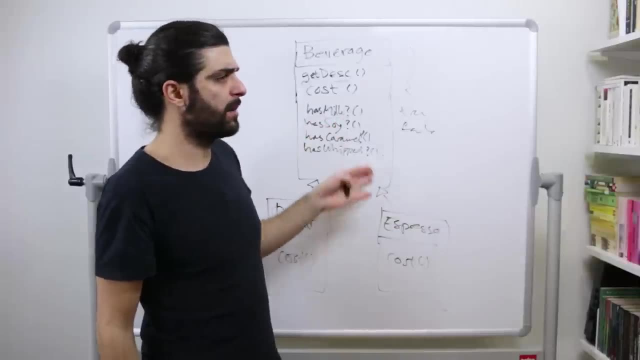 for soy, et cetera, et cetera, et cetera. And I mean you can see that for one this is extremely unexpressive. to pass all of those in And even setting these as parameters feels very odd. I think Sandy Metz has a great saying when she says that conditionals breed. So 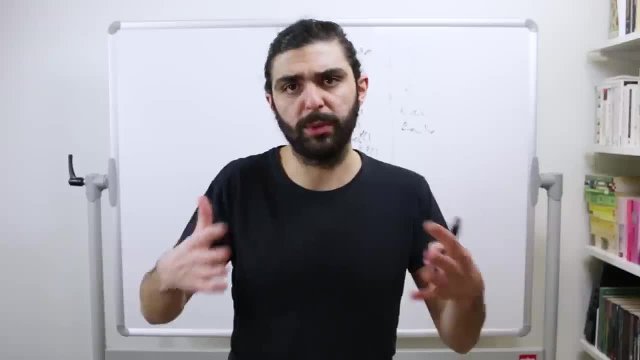 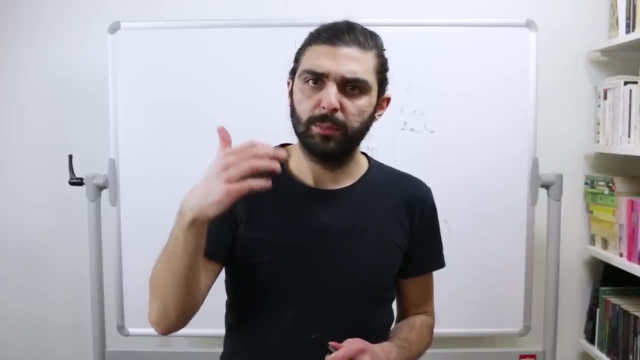 if you have one conditional, that will likely put you in a place where eventually you'll put even more conditionals in your program. And I can't remember who said this. Please put that in the comments, if you remember, But somebody said that returning booleans. 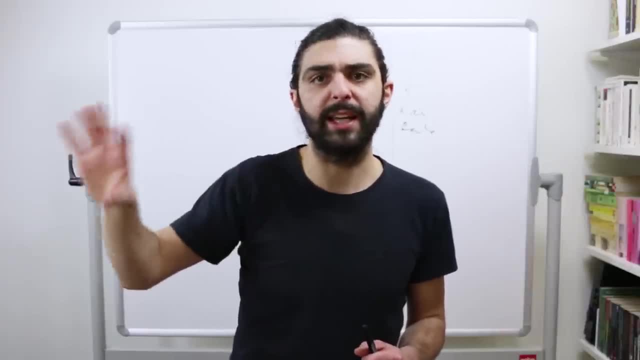 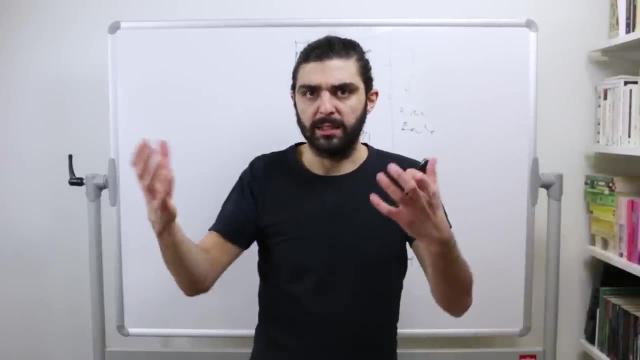 usually provokes conditionals elsewhere in your system. So the fact that we're returning a boolean will provoke the need to, at some other place, switch over that conditional, In other words, include that conditional in some kind of switch statement or if statement. 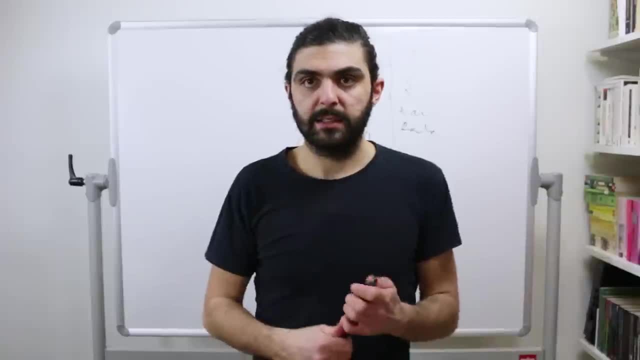 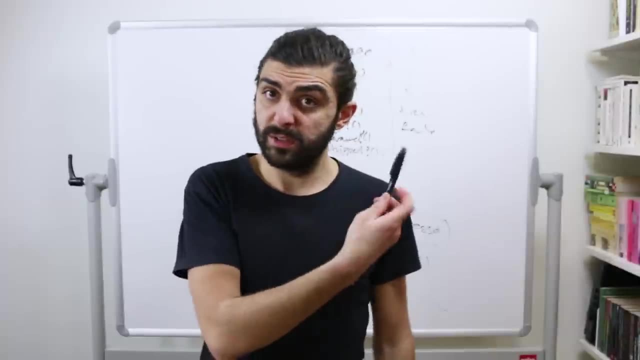 or something like this, essentially in some kind of condition, And the idea that you should stay away from conditionals is a topic for another discussion. Let me know when we can have that discussion. But beyond these problems, there are some other problems that they highlight in the 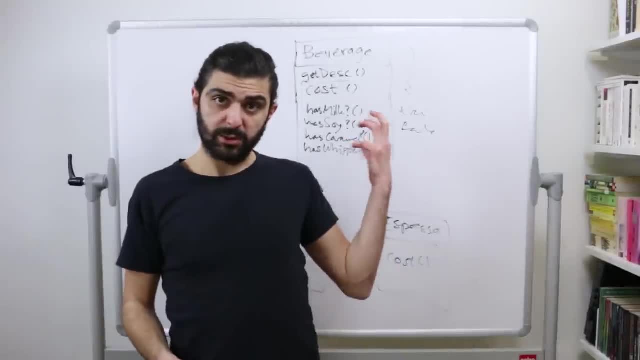 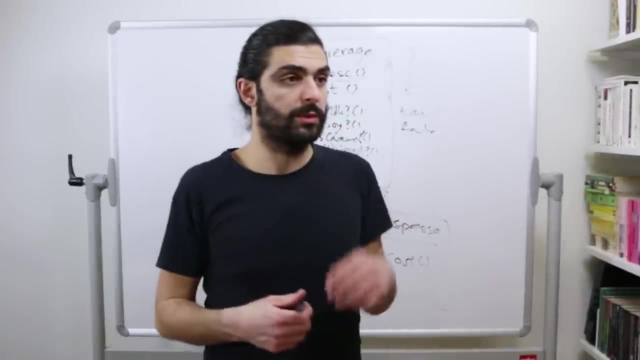 headfirst book. One of them is that you have to change existing source code when you want to add a new condiment or when you want to add a new extra, a new flavor. So if you want to introduce chocolate, for example, so maybe you want to put chocolate in your coffee. 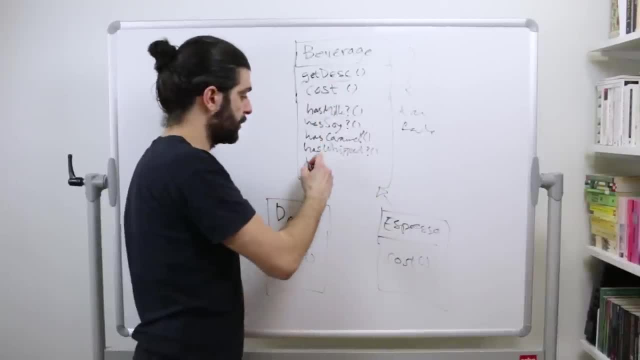 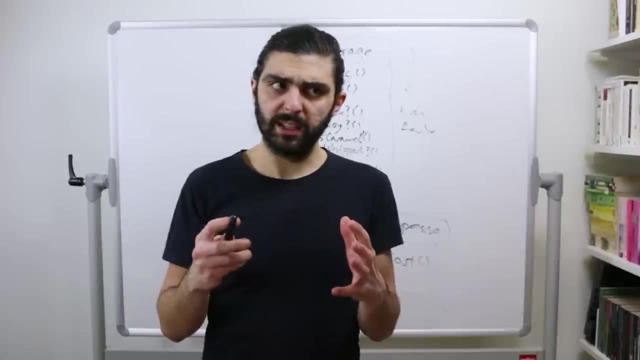 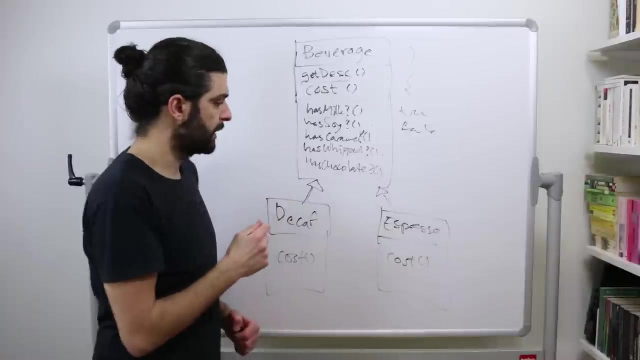 then you have to actually change the contents of this class by introducing has chocolate, And this violates the open-closed principle. So that's why they're suggesting that's a bad idea. But I think perhaps even a more severe problem that they're also highlighting is the fact that, because these are inheriting from beverage, 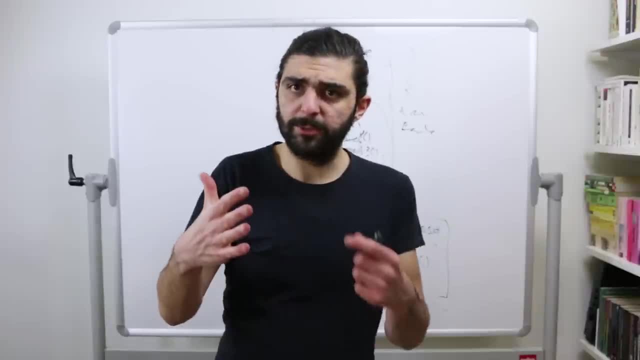 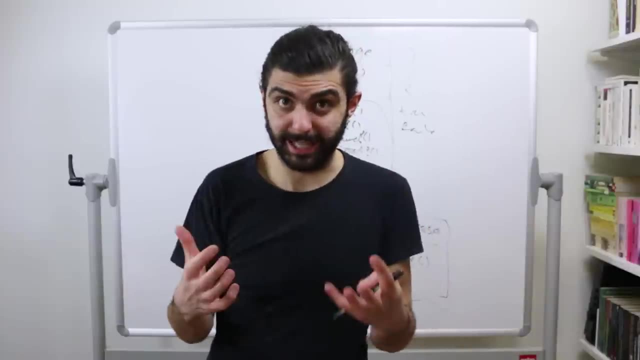 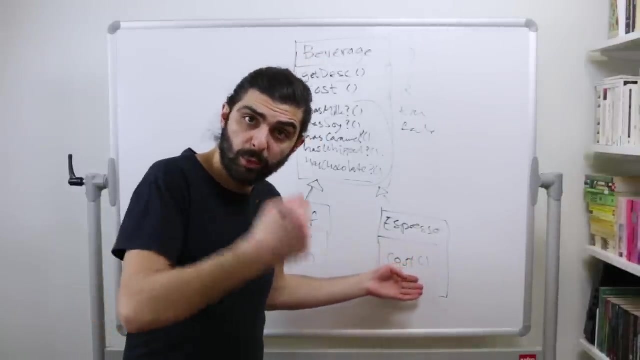 they'll also inherit all of the methods here. So perhaps you're already familiar with the interface segregation principle and Liskov substitution principle. These are two of the principles from the solid design principles of object-oriented programming, And the interface segregation principle states that a subclass should not be forced to depend on methods. 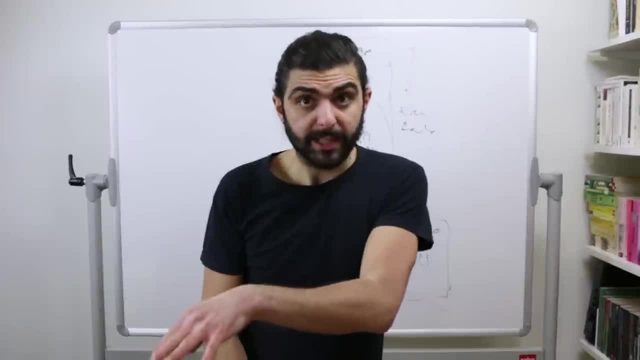 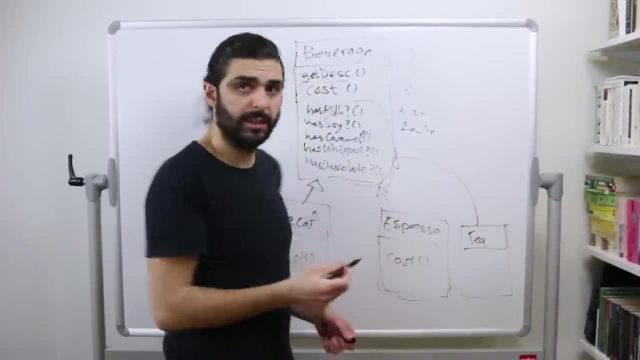 that it does not use. So, for example, they actually have a very great example in this book. The example is that what if you introduce tea and make tea inherit from beverage, Because it is a beverage and you want to be able to treat all of the beverages, all of the menu? 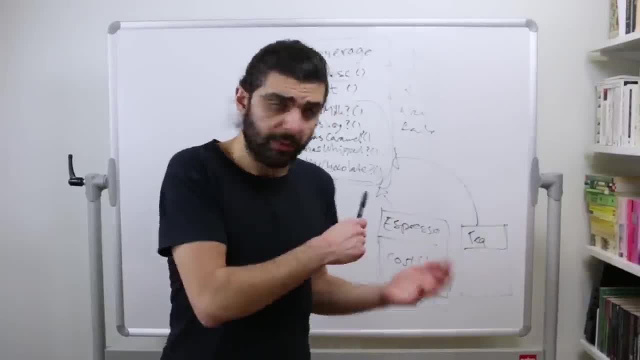 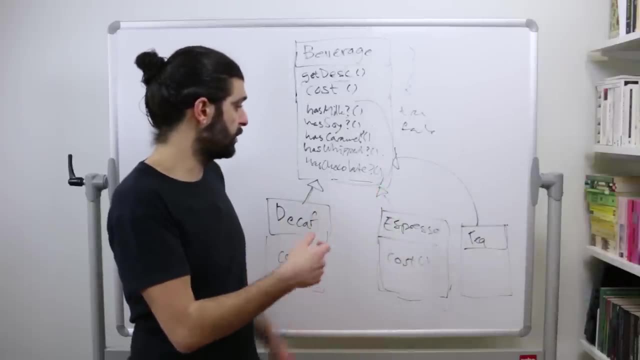 items the same, so you can print them to the menu. But what if some of the methods that we've put here actually don't apply to tea? So, hypothetically, I mean, maybe these do. I apologize if these do, but maybe chocolate simply doesn't apply to tea Like it's, so 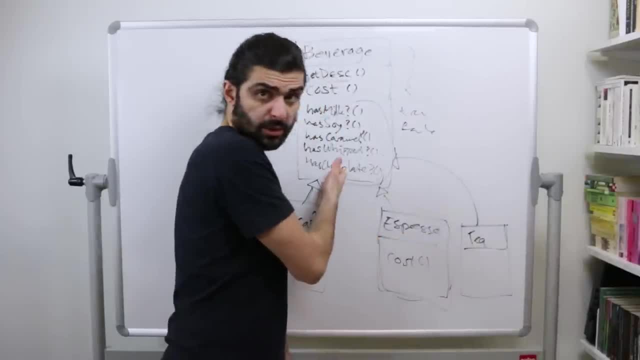 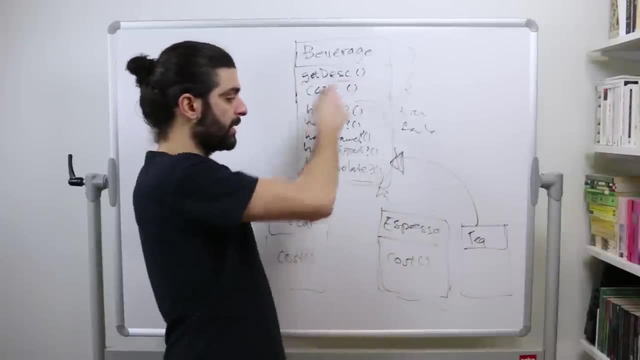 absurd that you can't order it. You can't order tea with has chocolate. Then maybe you are explicitly breaking the interface segregation principle because we're forcing, because tea is inheriting from beverage and we're forcing tea to actually have the default implementation. 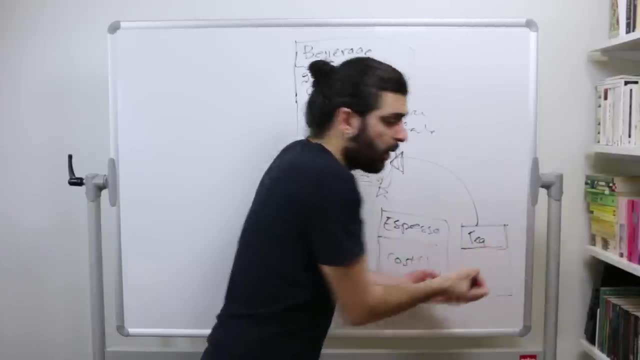 the implementation in the abstract class of has chocolate, even though it doesn't want to use it. So if you're interested in the interface segregation principle, I've talked about that previously in another video, So if you're interested I'll link that in the. 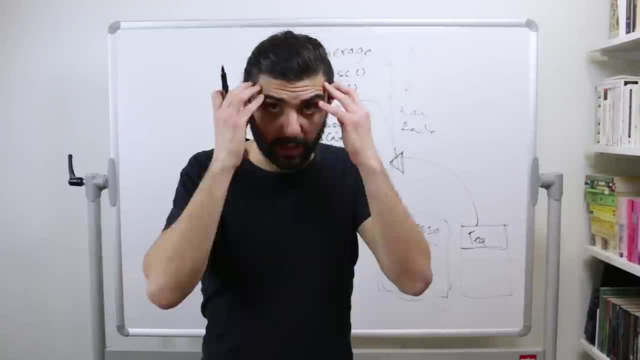 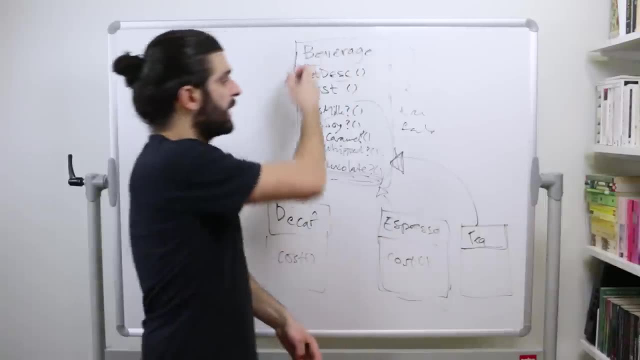 show notes. check it out, But shortly. the problem is that if you just think of an example where you have an instance of the tea class, you could have an instance of a tea class knowing that it's a tea class because you're treating it as a beverage. right. That's the. 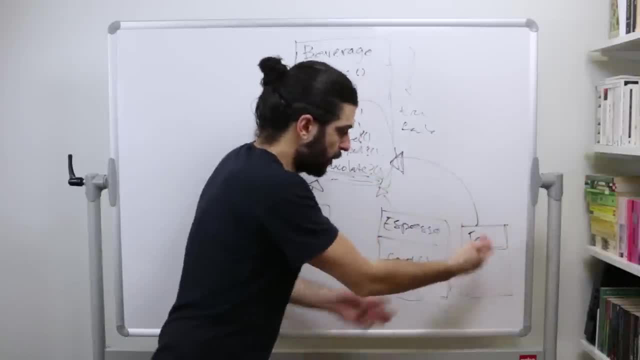 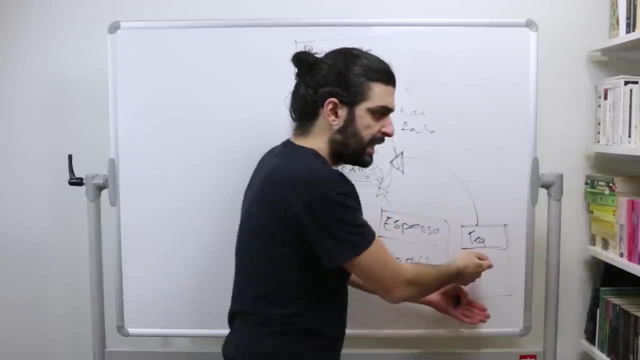 point of having inheritance. So you have an instance of a tea class. you have an object that's of type tea but you're treating it as a beverage And because you only know that it's a beverage you could call has chocolate. but tea surely doesn't have chocolate. And 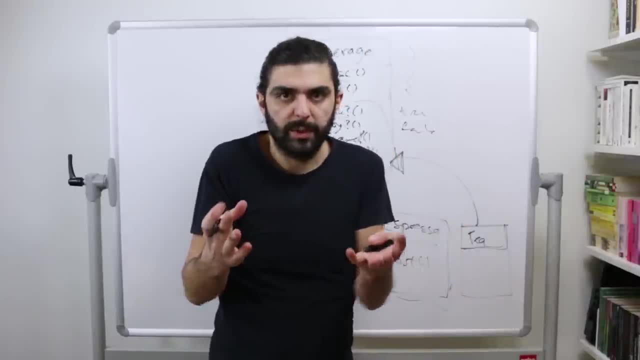 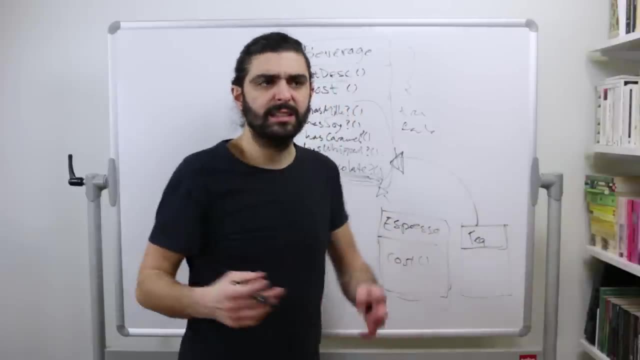 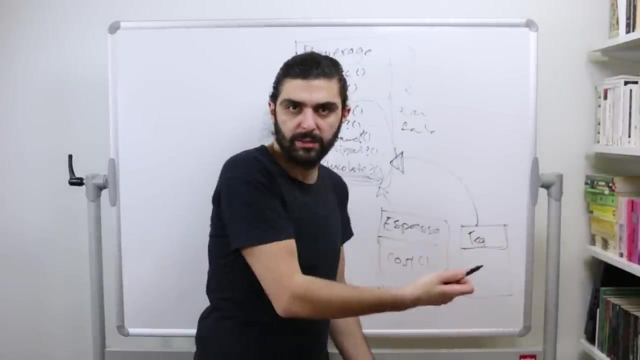 now, in this particular scenario that's not necessarily too dangerous, but on the general plane that's a crazy idea, because this method simply doesn't apply to this class. It's not that it's not doing anything, It's like it's completely undefined. It just doesn't make any sense within the context. 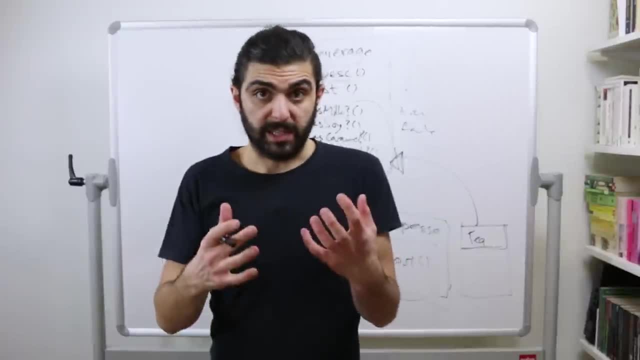 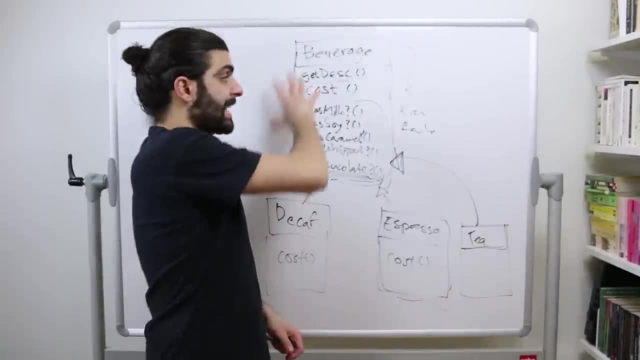 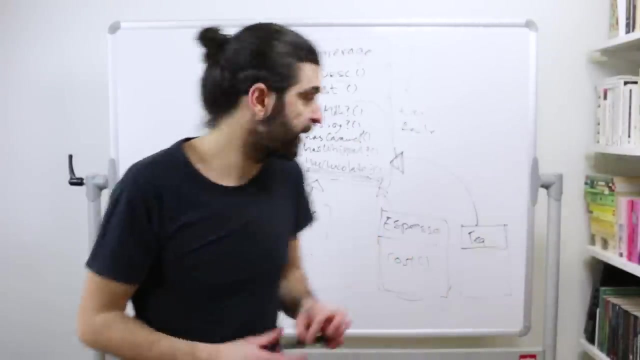 of tea, And that's why we should separate these. So the interface segregation principle essentially says that it's better to have multiple smaller interfaces than one single large one, which is exactly what we have here: a single large interface. Another problem with this design that they raise in this book is that they say what if a customer wants? 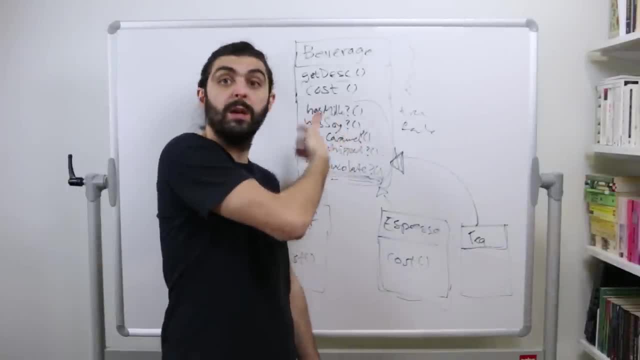 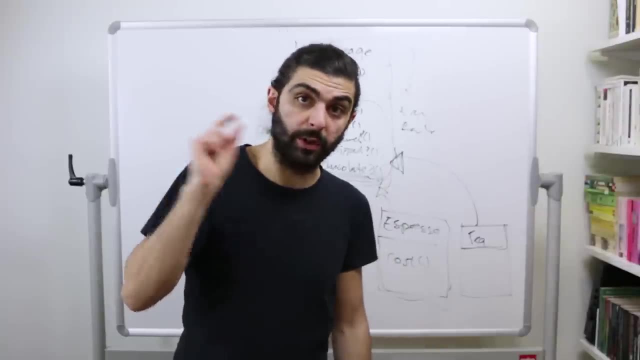 now, I didn't put mocha here, but their example is what if the customer wants a double mocha? I mean, most coffee houses have it so that you can get your coffee, and then you can get a shot of espresso in your coffee and whatever coffee you had. And then, if you just think, 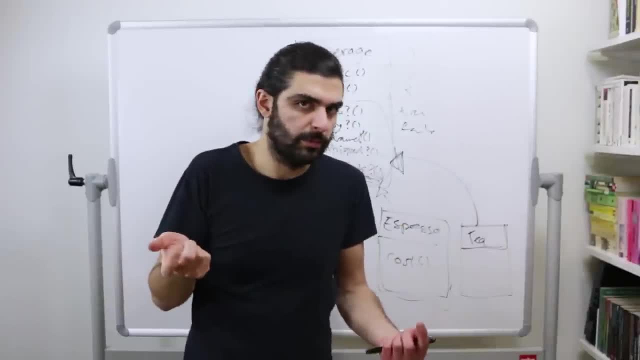 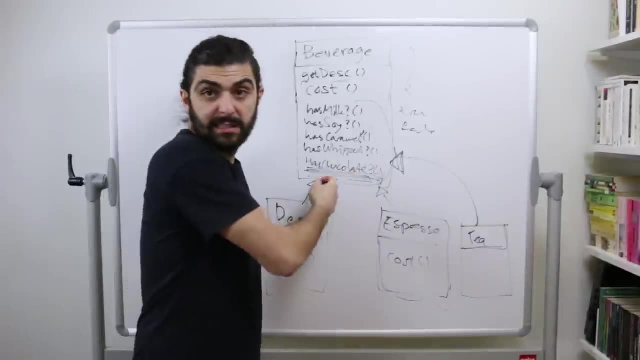 about the concept of one shot of espresso. if you can have one, of course you could have two. And if you could have two, then why not have three? hypothetically right, And that means that you would have has espresso shot, but then you would also need to have has double. 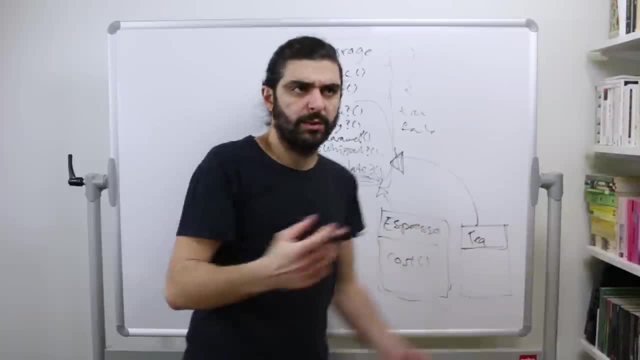 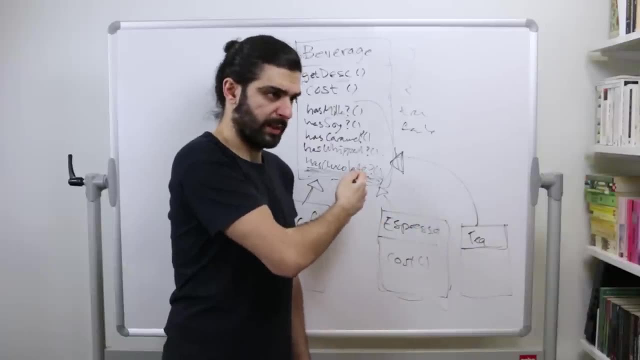 espresso shot and then has triple espresso shot. And then you're also in a sticky situation where you have to say, okay, if I have a triple espresso shot, I shouldn't also set Has double espresso shot to true. So that's kind of tricky to manage but also kind of stupid. 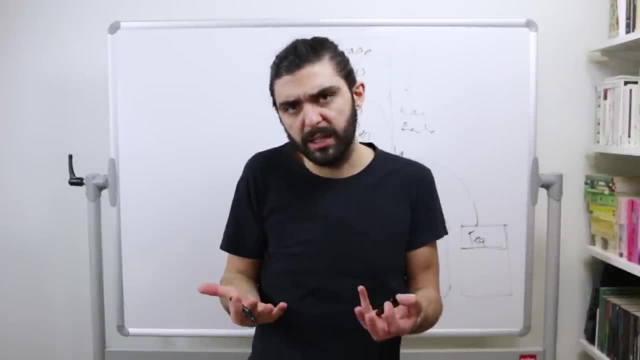 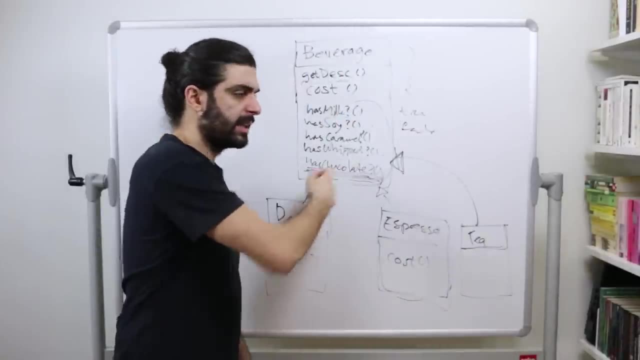 because the second espresso shot is just another one of the same thing, So why would that have to be a second one? But of course, then you could also think about strange designs, such as saying that: okay, instead of making that a Boolean, you would make that an integer. 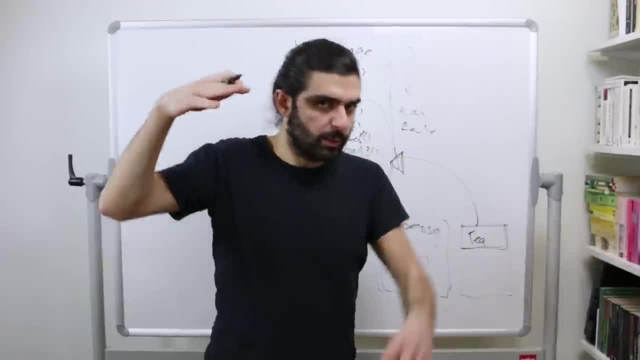 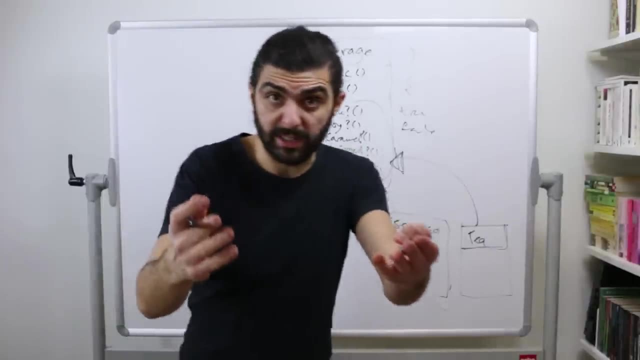 and then you count the number of times that you have. But I mean, hopefully you're feeling that we're sort of treading down a slippery path where it's just going to get more complicated and then you would have to calculate the cost. I mean, obviously, maybe I didn't mention 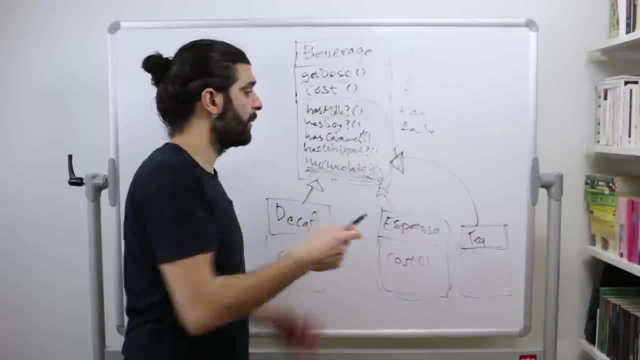 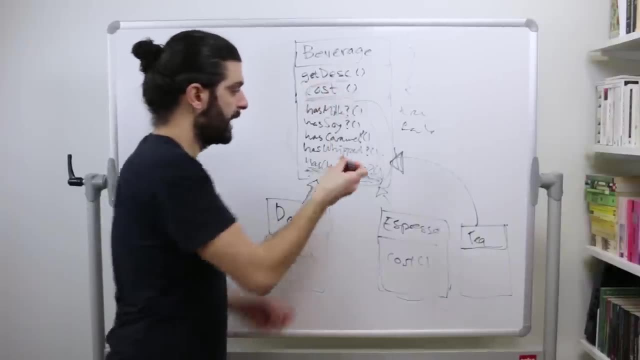 that before. But the point of keeping track of all these things is that the cost varies based on what kind of condiments you're actually putting into your coffee. So then the calculation of the cost method- how to actually calculate the cost of this particular beverage- becomes. 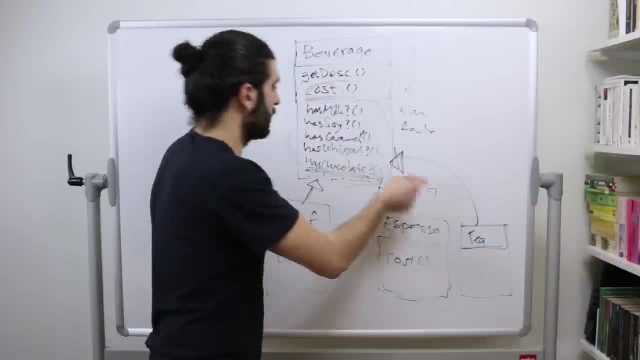 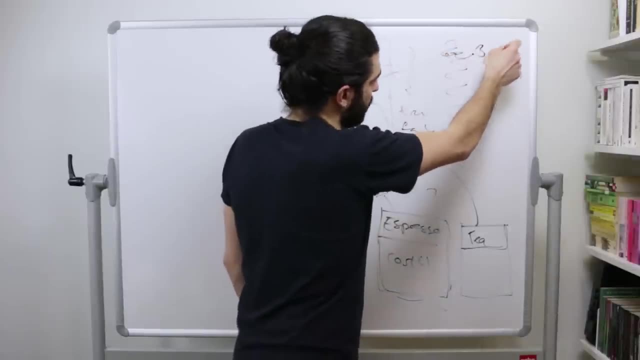 very complicated when you think about has espresso shot being an integer and has soy being a Boolean. So you'd have to have some nasty logic for the cost method where you would say, okay, if it has three, four espresso shots, then it's this price, If it's two of. 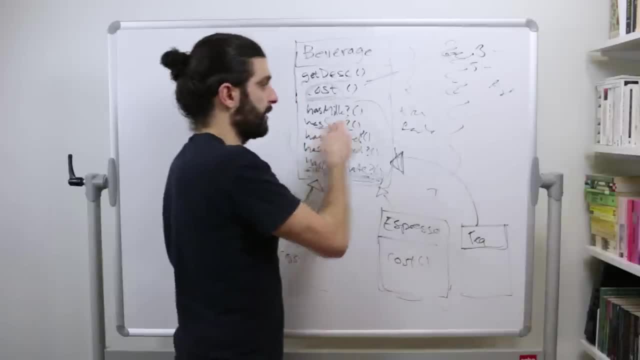 espresso shots, then it's this price, But then plus the fact that you have salt, soy, which makes it this, So if has soy, et cetera, et cetera. et cetera, I mean hairy. 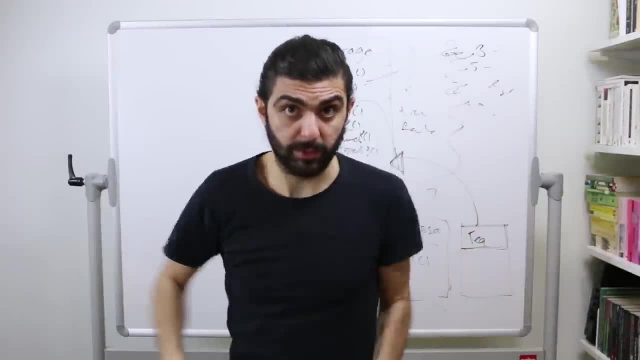 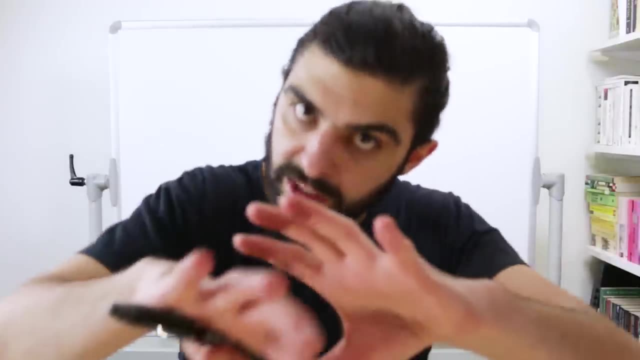 very hairy. So not a good idea, right? What can we do? And this is when the decorator pattern comes in. So let's start off by looking at the decorator pattern applied to this particular example, And then after that we'll look at sort of the generalized UML diagram and talk about. 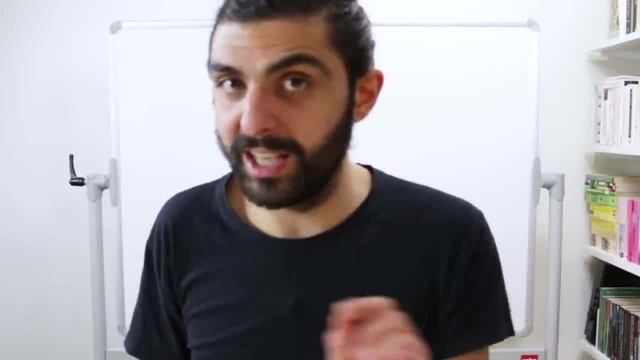 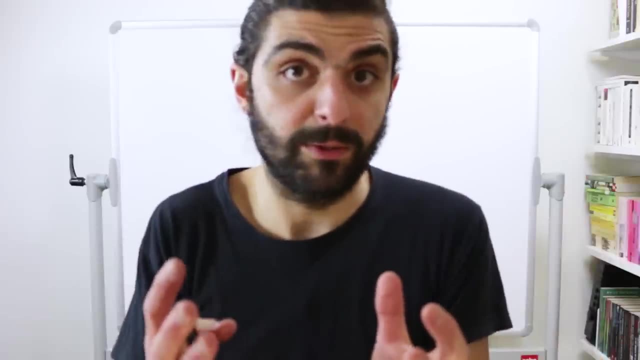 the decorator pattern in general And again, remember that I'm not saying that decorator patterns are actually suitable for this example that they've chosen. This illustrates the way you use decorator pattern very well, But I don't actually think that this particular use case is suitable for decorator pattern. 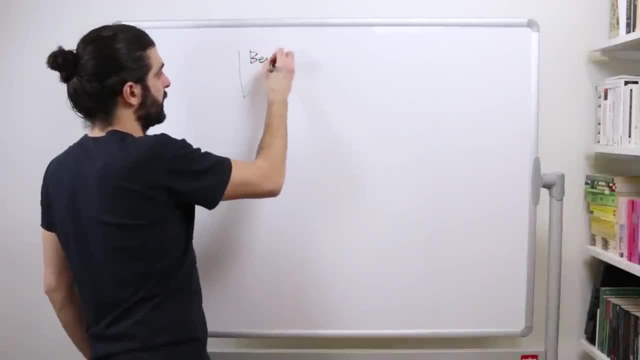 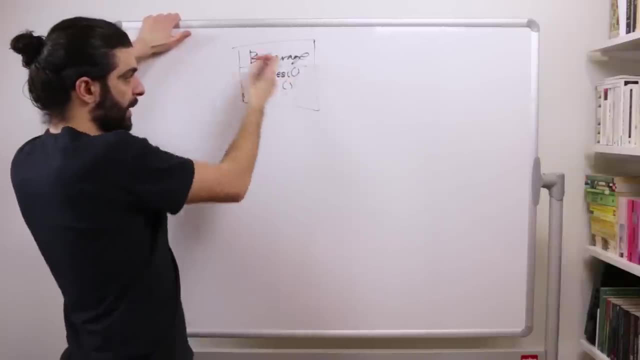 Moving on, let's check it out. So we start off with a class beverage. Again, the beverage has get description and it has price and it has cost. So cost returns to the price of this particular beverage and get description returns some kind of string representation. 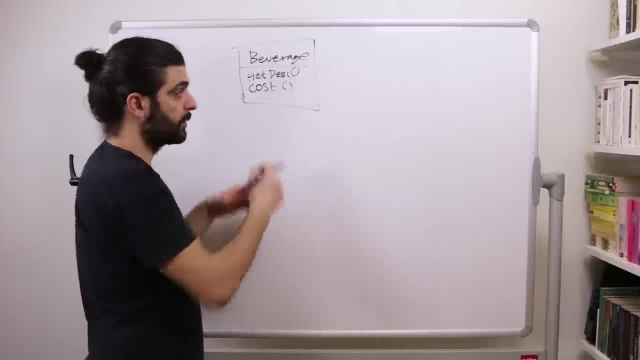 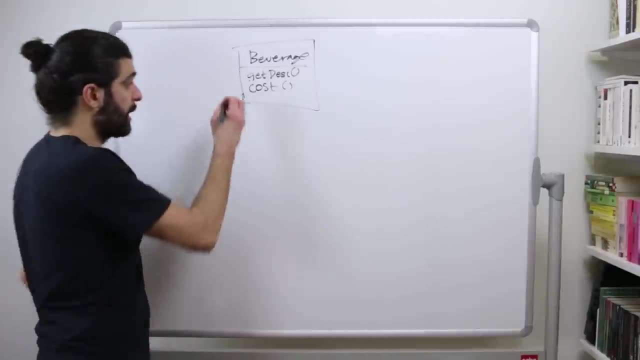 of the contents of this particular beverage. Again, remember, that could get complicated, because you can have all of these different condiments, all of these different extras, all of these different add-ons, And then we have those two basic types that we had before. 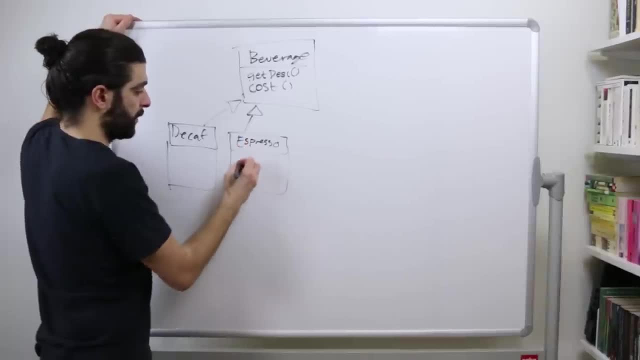 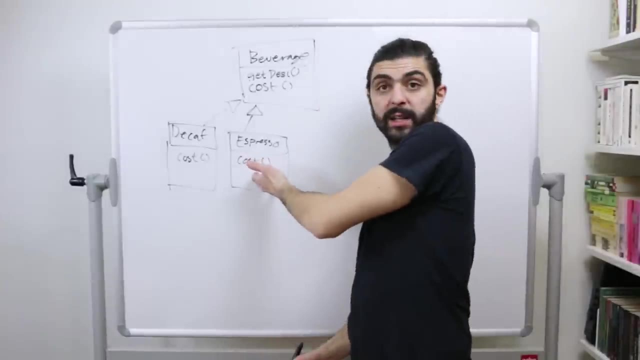 We have decaf and we have espresso, And both of these have their own implementation of the cost method because, again, they have different baseline costs. So the price of an espresso is different from the price of a decaf, assuming you put either no other condiments or you. 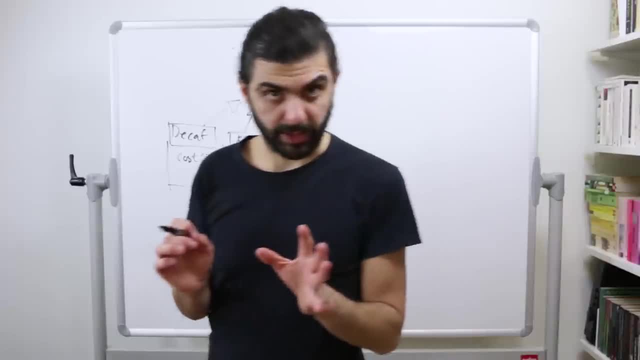 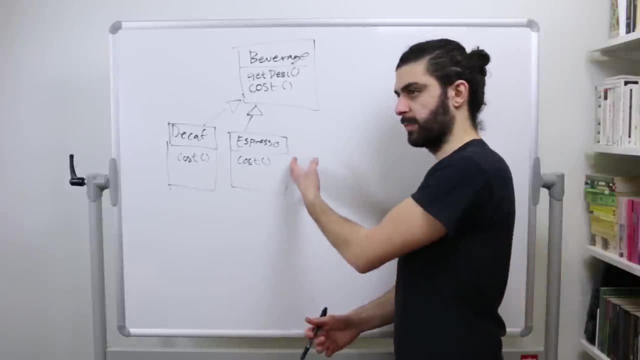 put the same condiments in them. Now, how do we make use of decorator pattern Instead of introducing multiple classes that represent all of the different combinations of the condiments? you have? espresso with mocha, espresso with caramel, and so forth and so forth. 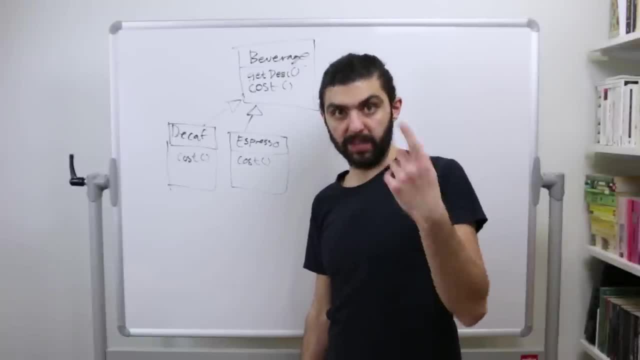 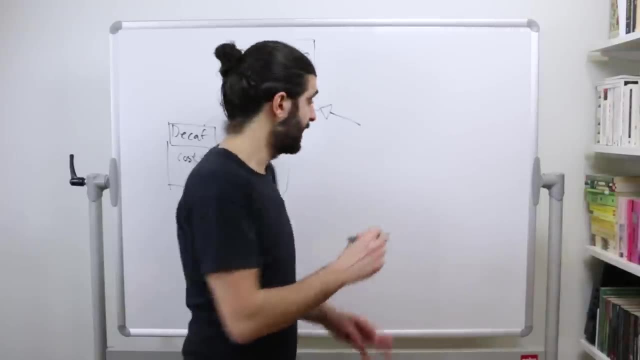 Instead of that, what we'll do is that we'll introduce a condiment decorator, But because of the length of the word condiment, I'll just use the word add-on instead. I'm meaning the same thing, It's just to make this simple. So it's an add-on to your sort of baseline. 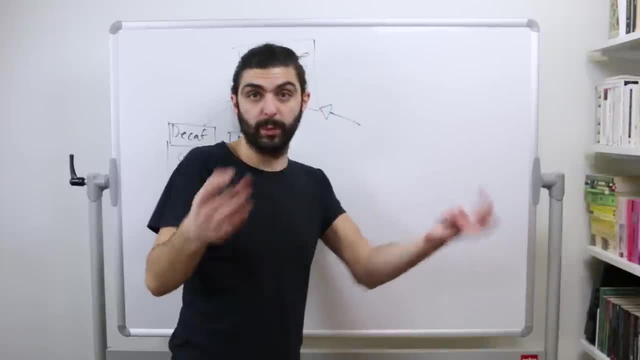 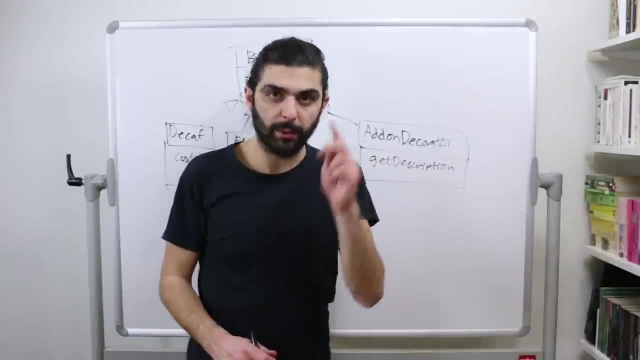 coffee, So you have a baseline coffee and then you add on something else, such as whipped cream. So we'll call this add-on, So add-on decorator, which implements the method get description. But remember what we said in the beginning about decorator pattern, The 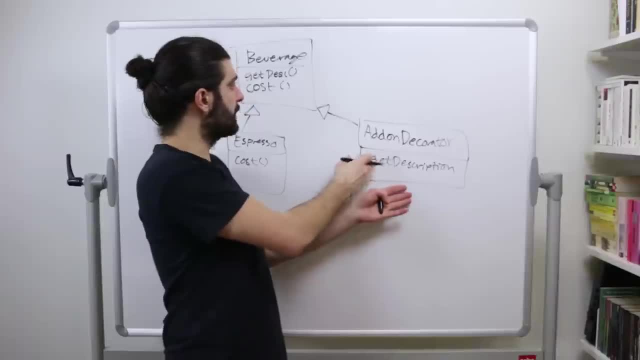 essence of the decorator pattern is that the decorator is a component of the method get description. So we're going to call this add-on decorator, which implements the method get description. So this add-on decorator is a component and has a component. So this arrow. 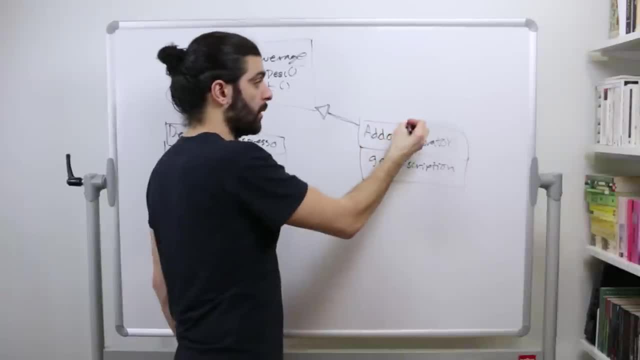 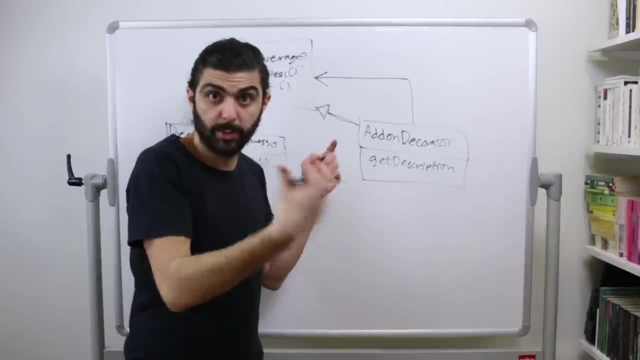 denotes that it is a beverage, but it also has a beverage, So the add-on decorator is a beverage. It behaves as if it were a beverage. So you can call get description, just like you can call get description here. Sorry, I should use the same name because we mean. 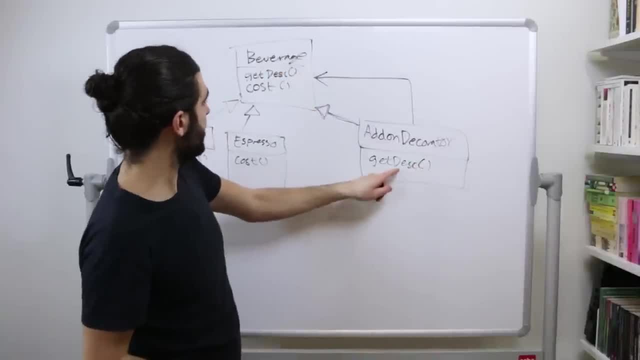 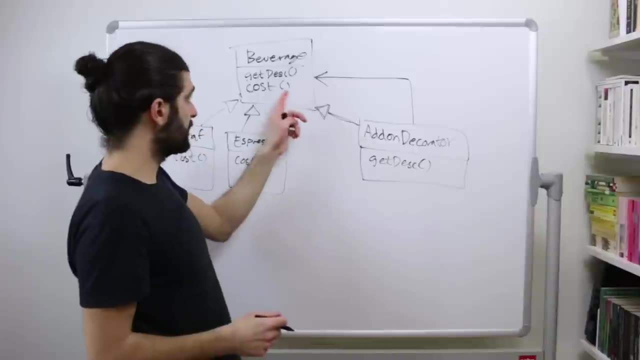 the same method. I use the short notation get desk. You can call get desk on an add-on decorator because it is a beverage, and you can call cost, even though we don't define cost here, Because all beverages have costs, and if the cost has a baseline implementation here, then 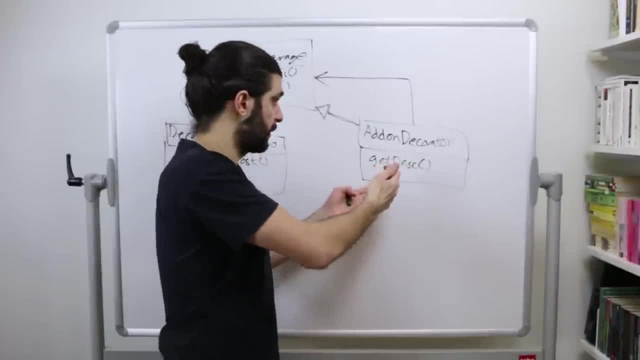 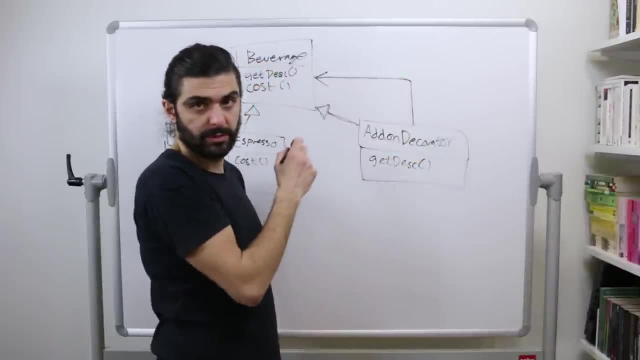 you have an implementation for cost and you can, then you can call cost in the add-on decorator. So then it behaves as if it were a beverage, because it is a beverage, but it also has a beverage. We'll get into more about why this is and what this means, But what we then? 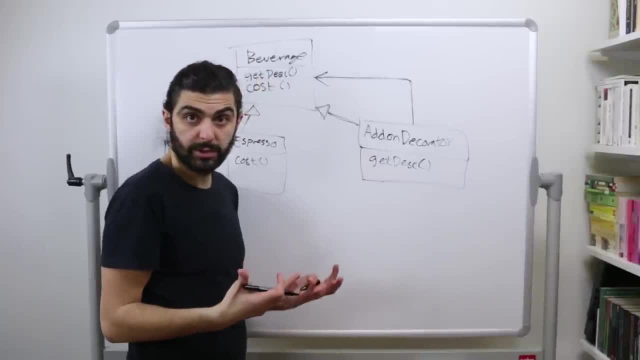 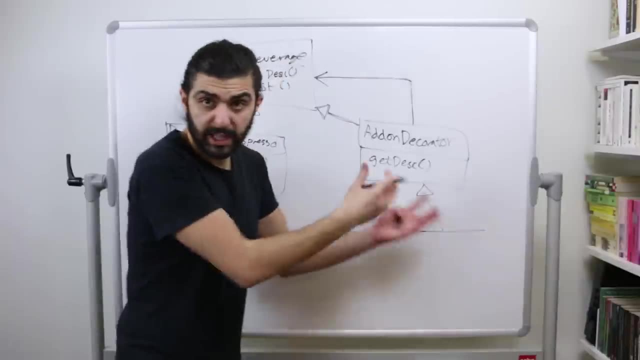 do is that we say that the add-on decorator has a number of implementations. A number of different classes are add-on decorators, So I'll just do two. but you have to realize that you can have as many as you want, and that's the point. We were talking about different. 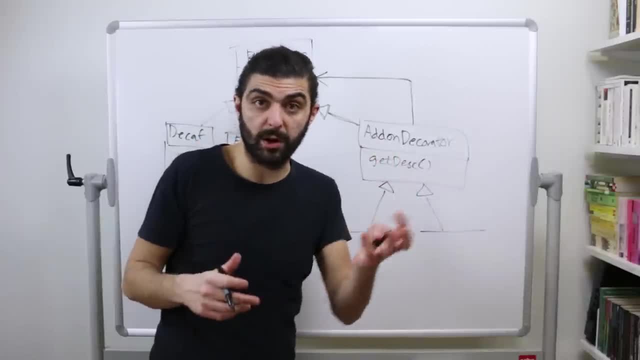 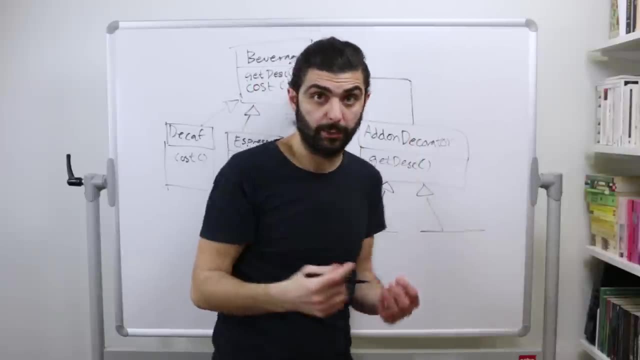 condiments before different add-ons like soy and whipped cream and caramel and chocolate and so forth and so forth and so forth, And all of these could be different add-on decorators or, in the book, condiment decorators. So let's do one. Let's say caramel, So car-a-mel. Now 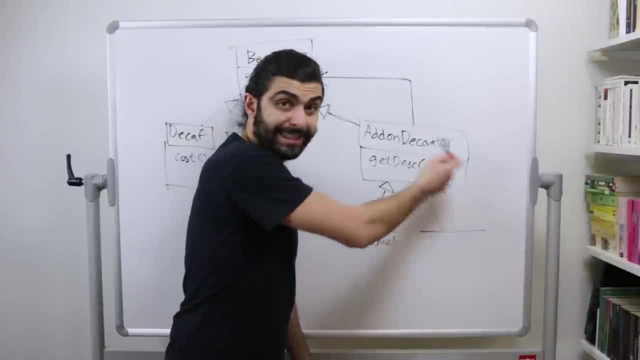 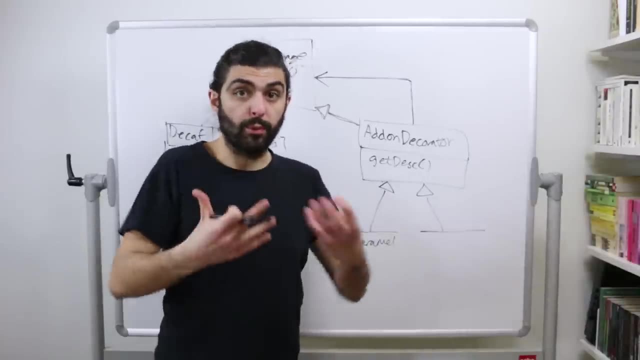 if I would put this in code, I would probably actually call this caramel decorator, just to make it very clear to the person that this is a decorator. Remember the power of using semantic naming. I'm using proper naming so that other people can understand what you're actually. 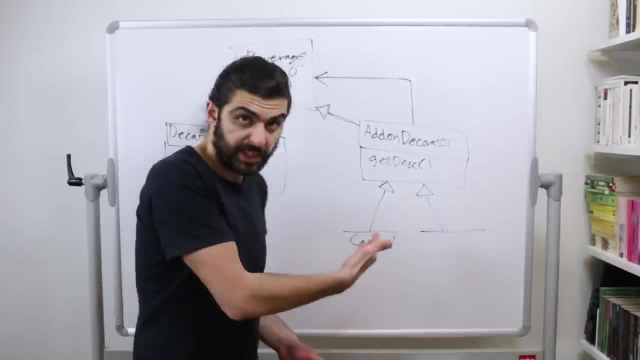 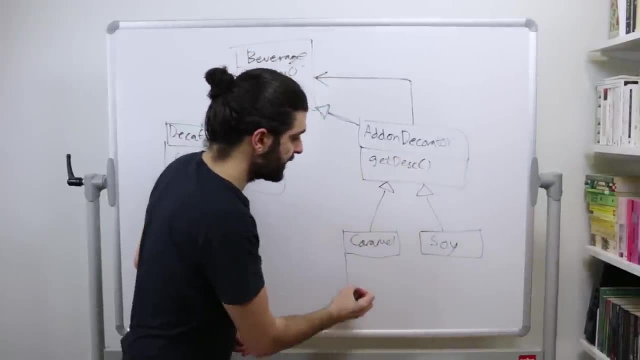 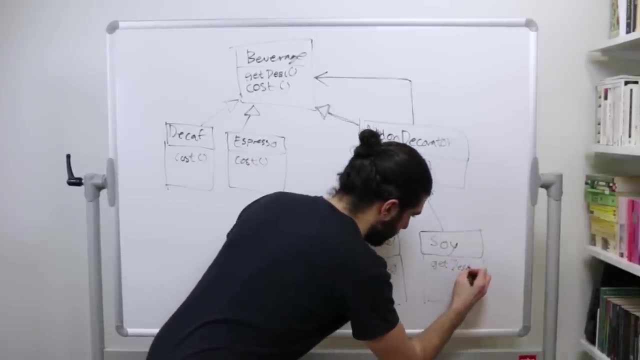 doing. But here, to save space and as they've done in the book, I'll just call this caramel And let's choose another one with soy. And these that are decorators, that are add-on decorators, these implement, both get description and cost. So both of them have get desk and they have cost And this: 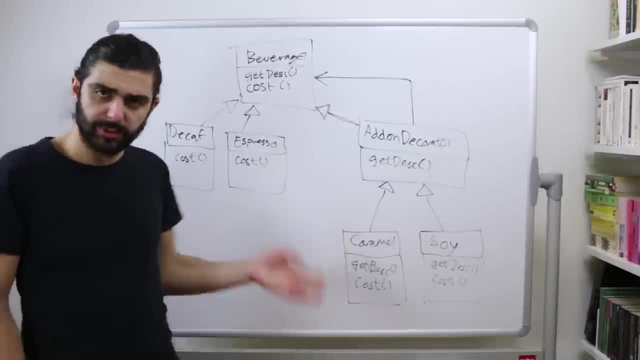 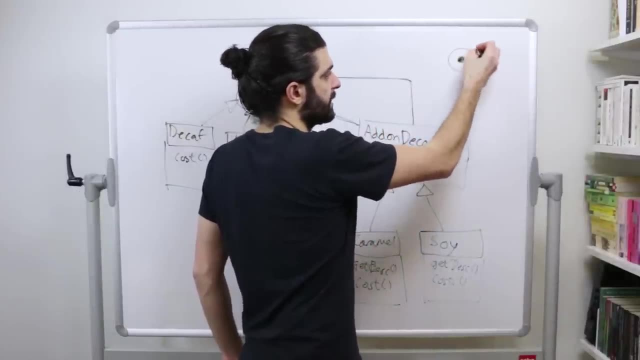 might seem really odd, and don't be frightened, but it's actually kind of smart. So the point here is that remember the original image that we drew, where we had one class in the middle and then something that wrapped it and another thing that wrapped it. Here's the point. The object in the 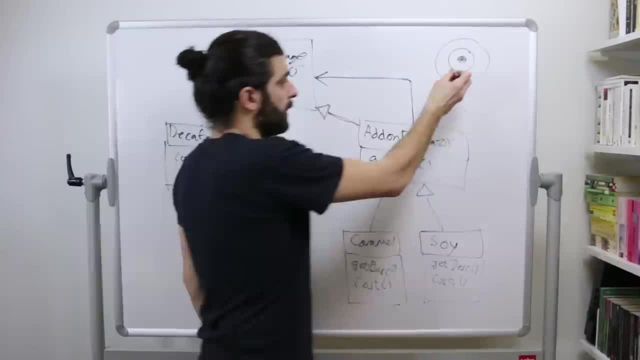 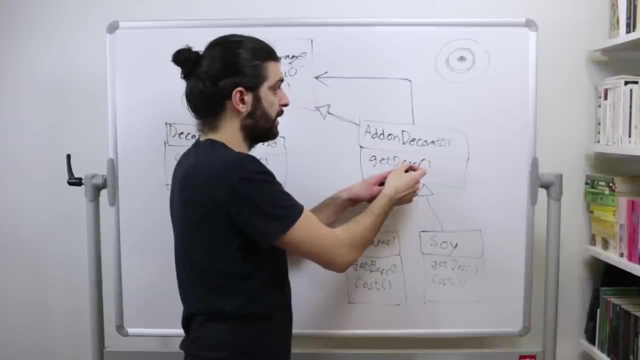 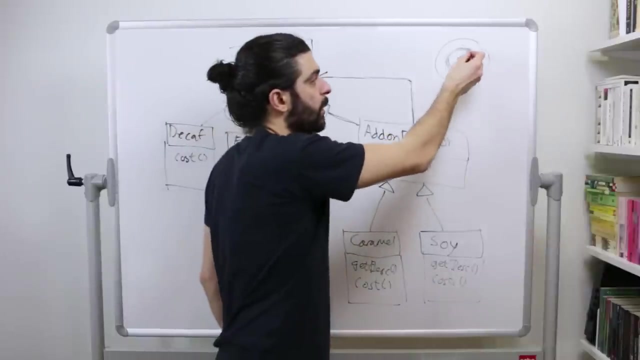 middle right, the instantiated object in the middle, that's a beverage. The thing here, the thing that wraps it, the first decorator is an add-on decorator. It's an add-on decorator that is a beverage. It behaves as if it were a beverage, but it also has a beverage, And that's what we're trying to denote. 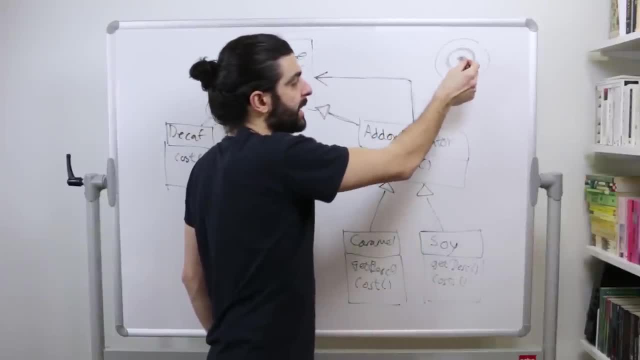 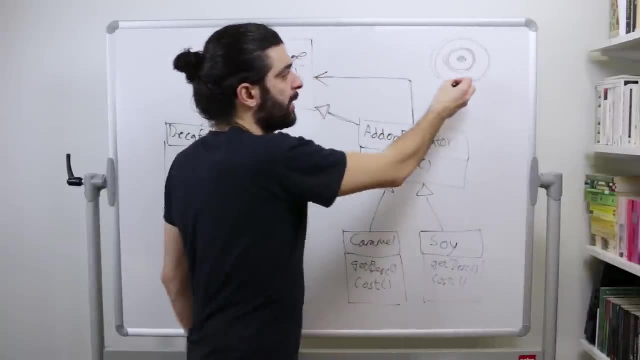 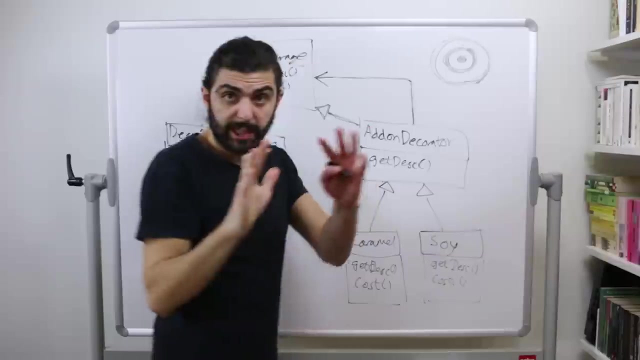 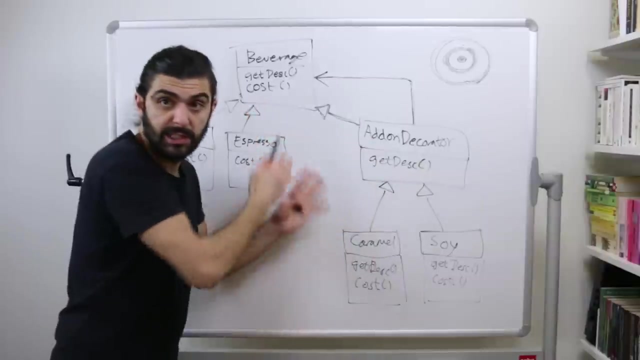 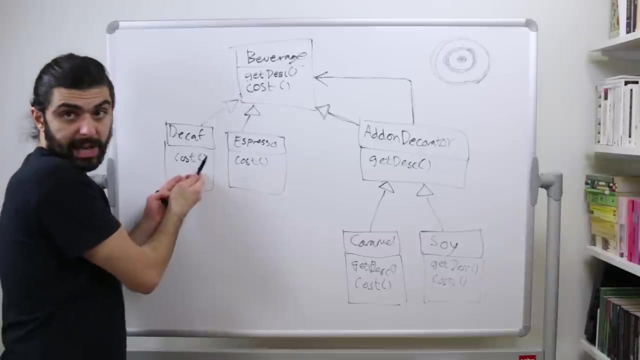 when we're drawing it outside or like as if it were comfortable. So this thing is an add-on decorator and this thing is actually an add-on decorator as well. So we have an add-on decorator as in the type. we have an add-on decorator that wraps another add-on decorator that wraps the beverage. And concretely, now we're talking about what sort of abstractions they are of. but if we talk concretely, this object has to be either- given that these are the only classes that we have, it has to be either an espresso instance, an instance of the espresso class, or it has to be an instance of the decaf class. 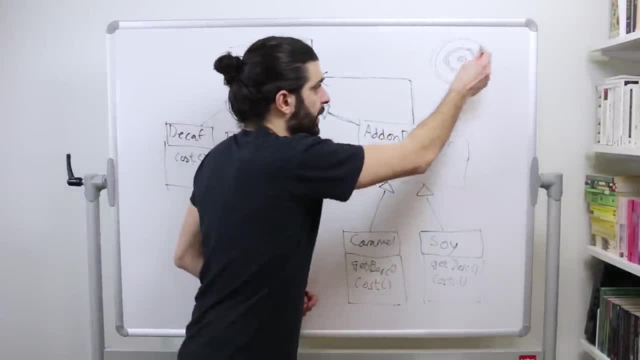 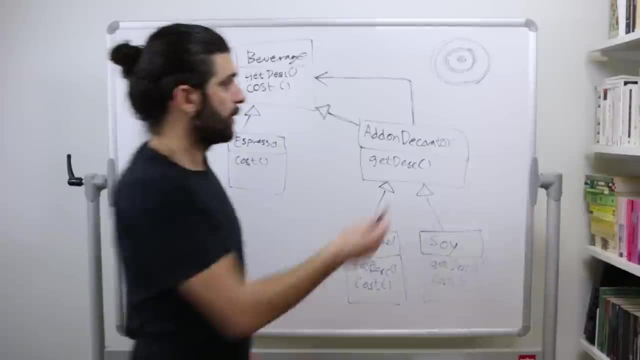 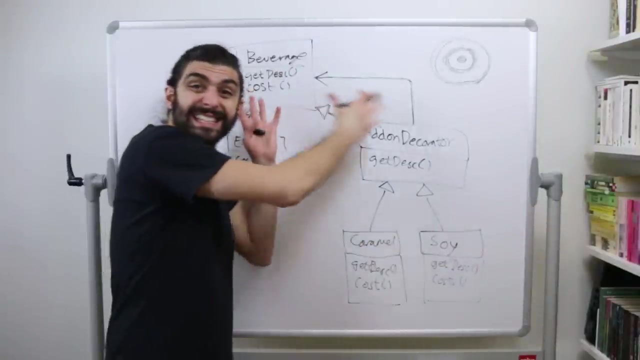 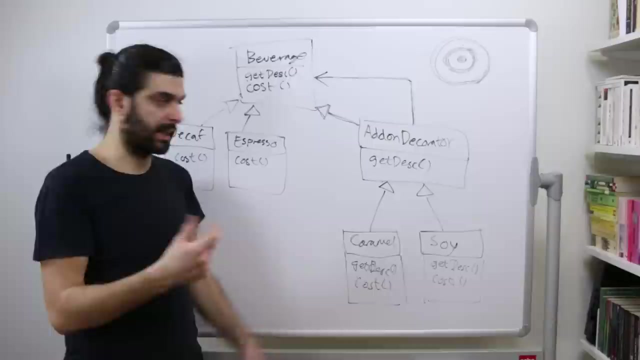 Because This is a beverage and this decorator and this decorator has to be either a caramel decorator, or it has to be a soy decorator, one of them, So this could be caramel and caramel, or caramel and soy, etc. etc. All of the different combinations that you can imagine. So the point, then, is that, with this design, what we've constructed is that we've constructed a situation where, instead of having a single class that describes decaf, a single class that describes espresso, a single class that describes decaf with caramel, a single class that describes espresso with caramel. 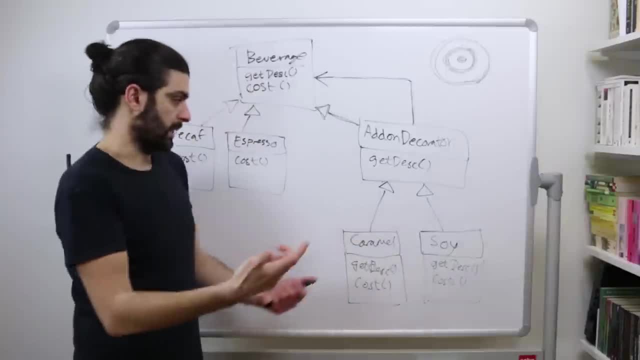 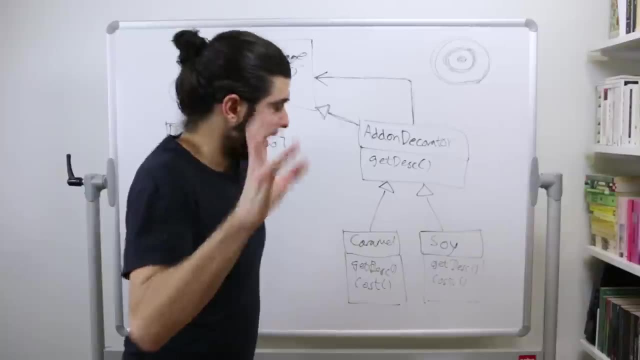 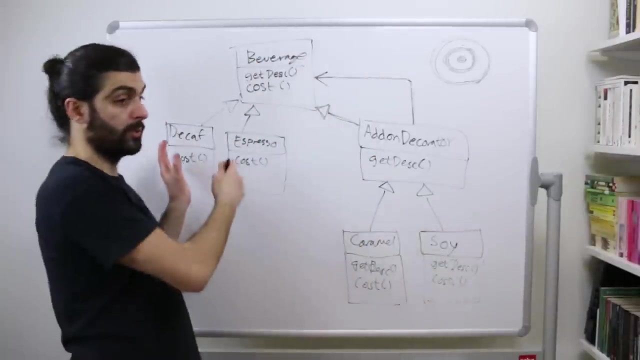 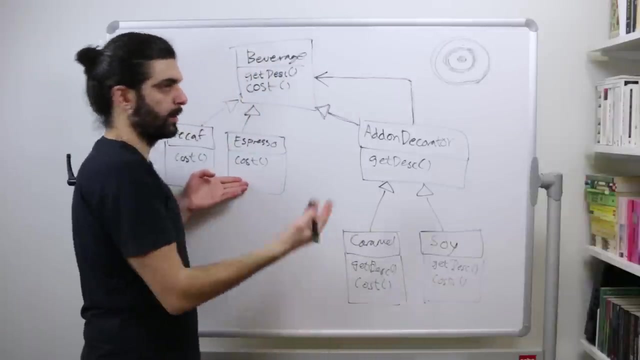 A single class that describes decaf with caramel and soy, a single class that describes espresso with caramel and soy, and so forth and so forth. Instead of having all of those classes in the class explosion scenario, instead of that, what we've done is that we've separated the concerns like this and we decorate in all of the different add-ons that we want to add to the coffee. So how do we do that? We wrap them So with this design, you can create an espresso with caramel. You could create just an espresso. You could create an espresso with caramel and soy by saying: I'll create an instance of espresso. 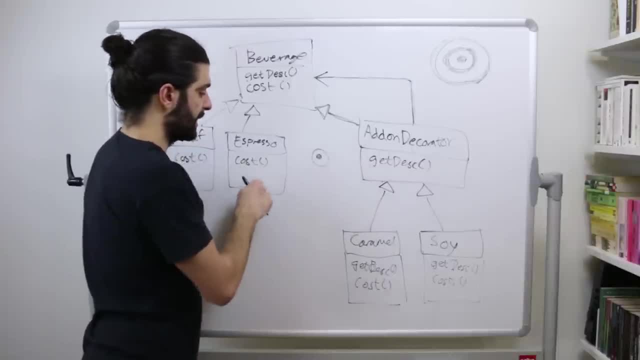 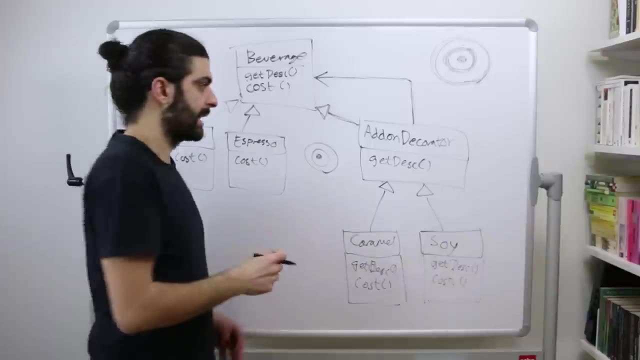 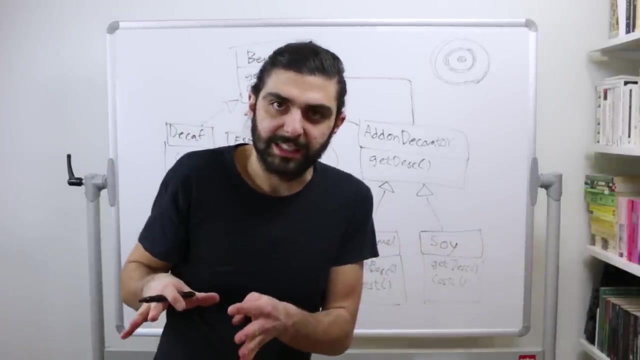 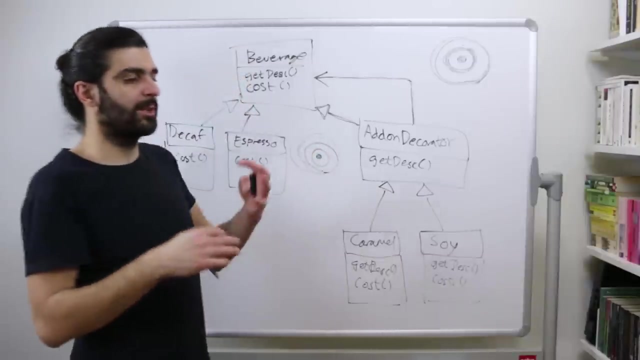 Then I'll pass that instance of espresso to a caramel and I'll pass that instance of a caramel decorated espresso to an instance of a soy class, Essentially making that a soy decorated caramel decorated espresso. Right, and you can see the critique creeping up of the fact that this design pattern often makes it much more difficult to reason about your code, and after you've wrapped it and wrapped it, and wrapped it, and wrapped it, it's kind of tricky to remember what you actually have. 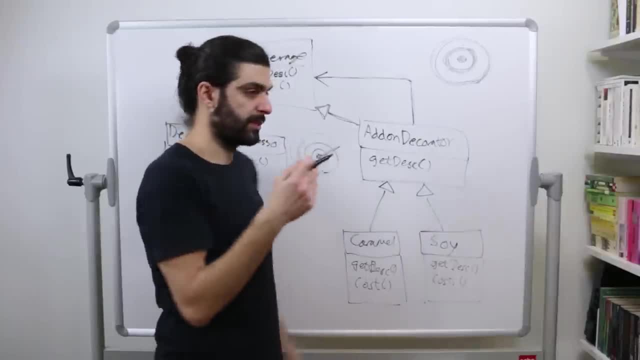 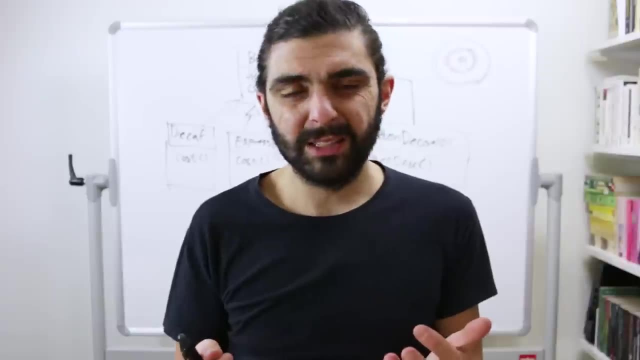 And, as far as I understand, if you're interested in order, If you're interested in the order of how you wrap things, and this design pattern is not suitable for that scenario. but that's a different discussion. So we haven't really talked about what get, description and what cost, what these two methods do. 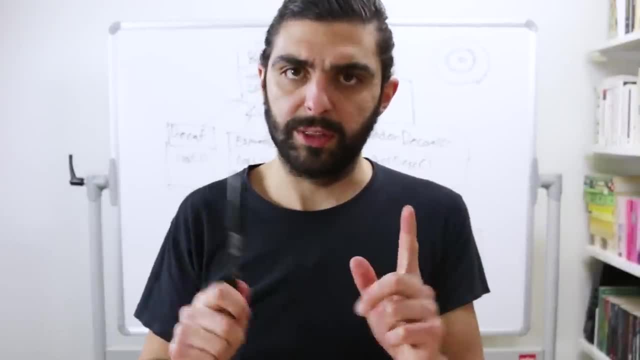 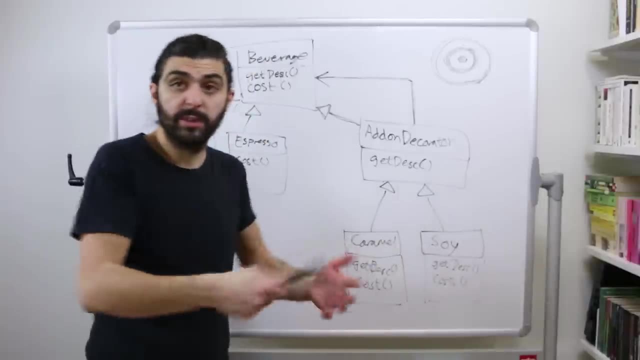 So let's quickly talk about that. Let's actually only talk about the cost method, because I think you can figure out how get description works in exactly the same way. So the point is again that depending on which add-ons you put into your coffee, the price will be different. 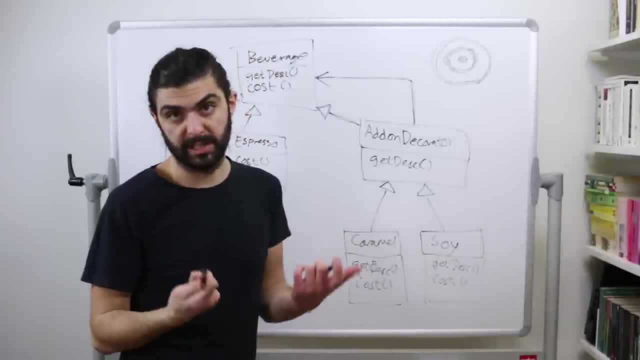 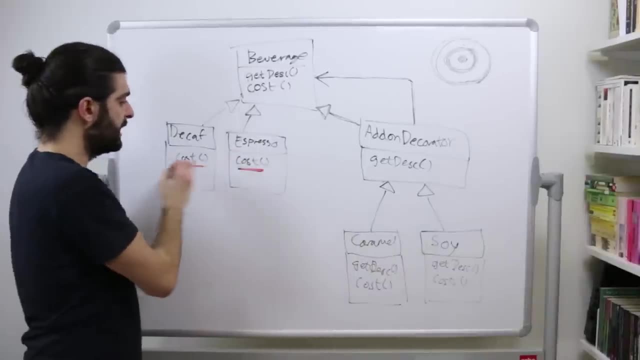 So remember that the idea of the cost method is that it returns a number that represents the cost. So for the sake of simplicity, Let's try this, Let's just say that it returns an int. So the cost methods here in the beverage classes, these cost methods, they in some sense return the baseline cost. 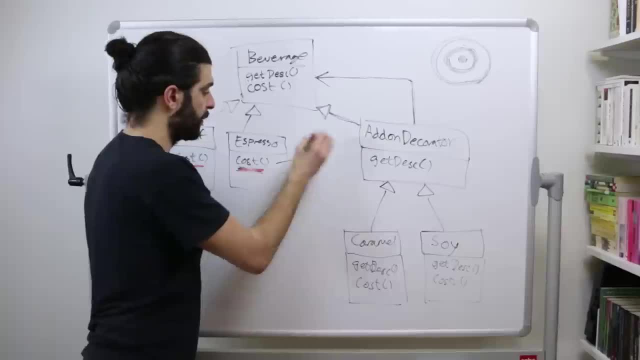 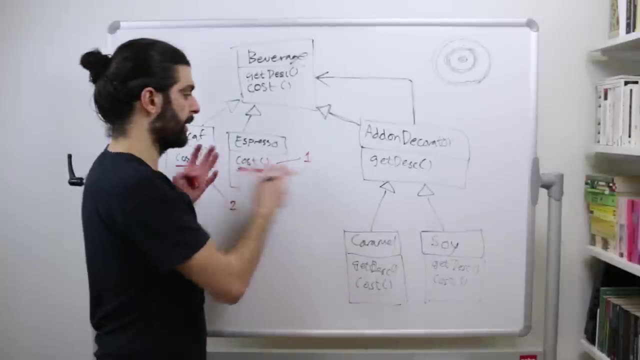 So if you just order an espresso, then this is what you'll get. So say, the price of an espresso is one and the price of a decaf is two. Hypothetically, I mean never mind the currency and never mind the relative pricing. Let's just say that these are the prices. And then let's say that when you add caramel to whichever beverage you already have, you add an additional two to whatever cost you already have. And let's say that when you Add soy, you add an additional one to whatever cost you have. 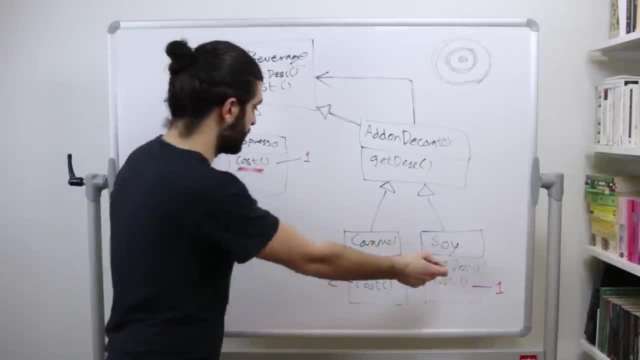 So if you get, hypothetically, if you get- an espresso with caramel and soy, then you should have one plus two plus one, So three plus one, four. So the price of an espresso with caramel and soy should be one plus two plus one, So one, three, four. 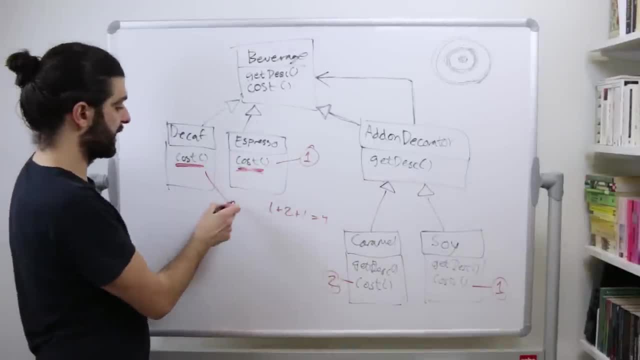 And in the same way for all of the different combinations. So if you get a decaf that has a baseline cost of two and then you only add caramel, then you add two and then you also end up with a price four, And so forth and so forth. 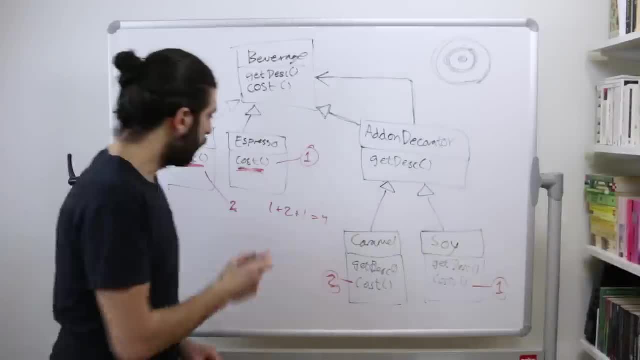 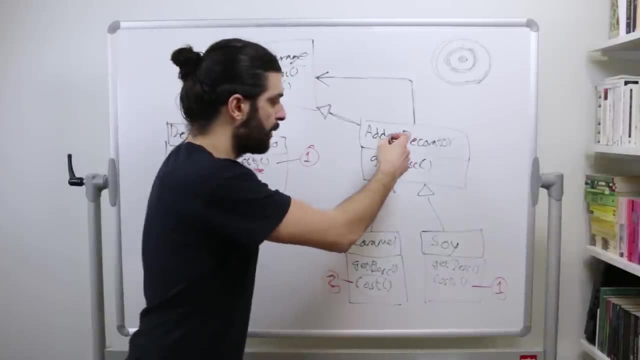 I think you can see how that works, But how do we actually implement that? What is the implementation of this method And why isn't it actually the same as this method? Because, if you think about it, you could just keep wrapping decorators and decorators, and decorators. 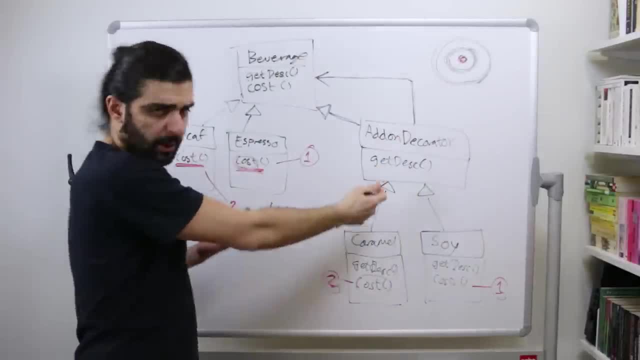 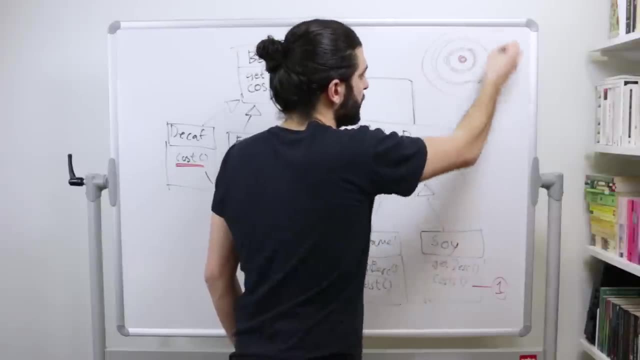 Why do you need to have something here that's different from the decorators? If you're familiar with recursion, you can think of it as that this is the base case. So you're using recursion to go down the chain of decorators, But then at some point you need to reach the base case, which is decorators. 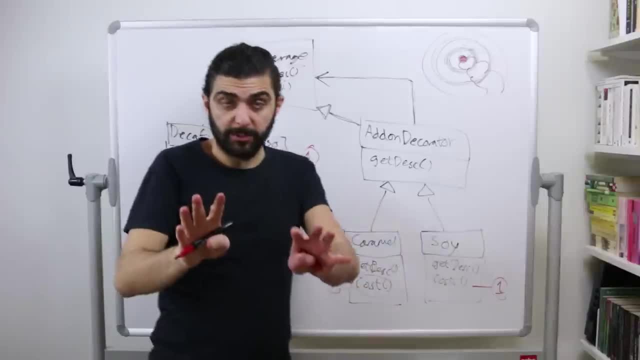 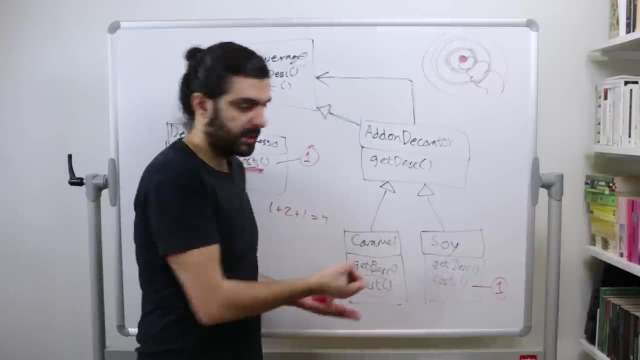 This cost and this cost and then you can go back up. But if you're not familiar with recursion, never mind, we'll have that discussion some other time. You can just think of it this way: This cost is an add on. This is not the baseline cost. 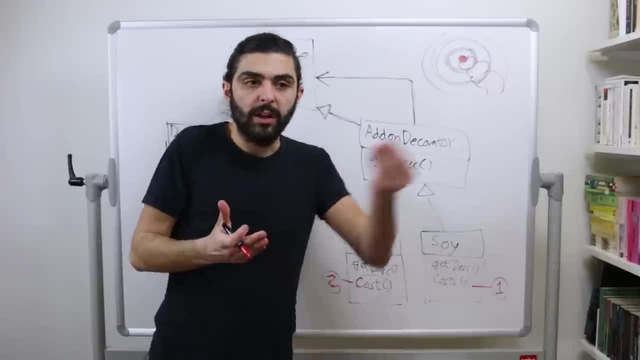 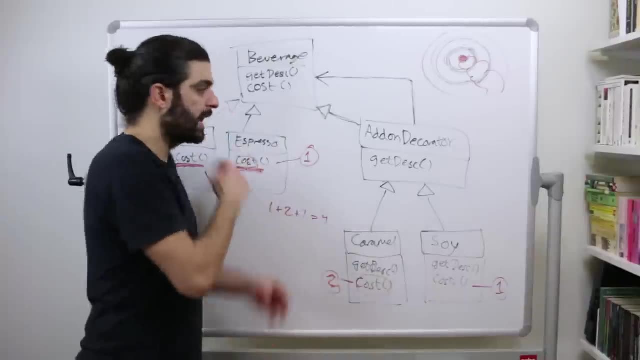 This is a cost that can only exist if you have another cost that it adds to. This cost is existent in and of itself. This is the baseline cost. You can get this thing in and of itself. You cannot get a decorator in and of itself. 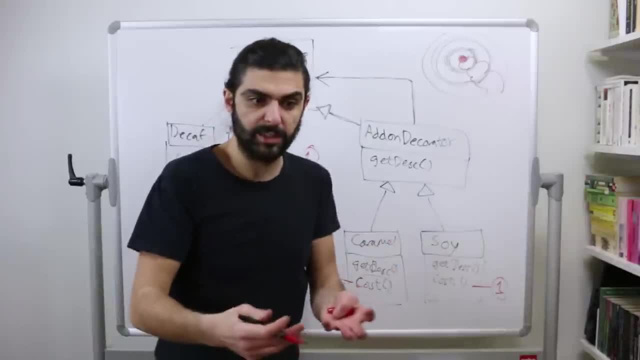 Caramel just by itself doesn't make any sense, Right? Imagine you go to the counter and you say: Can I just get this thing? I just have some caramel. and then you stick out your hands or you just drink it from the machine or whatever. 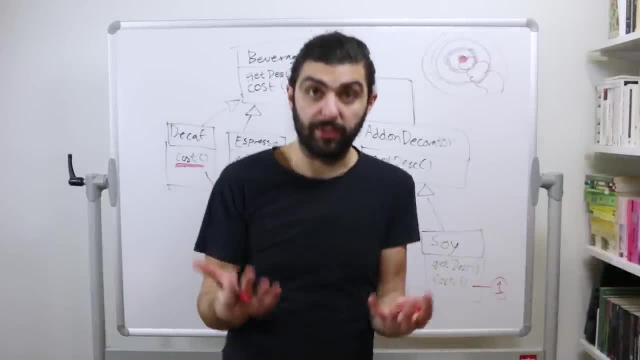 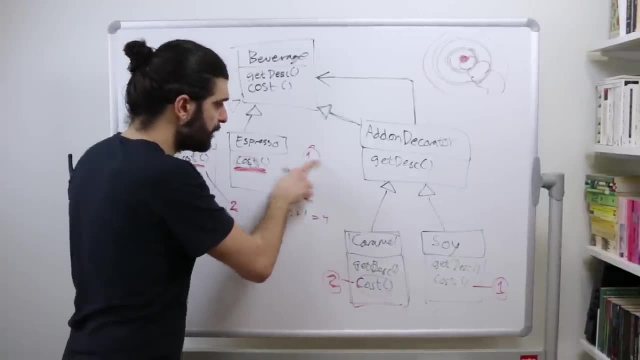 Essentially, that doesn't make any sense within the scenario, So decorators have to wrap something that can exist in and of itself. So if you think about the implementation of cost here, when we say that the cost here returns one, We actually mean that explicitly. the implementation of this method would probably be something like return one, semicolon done. 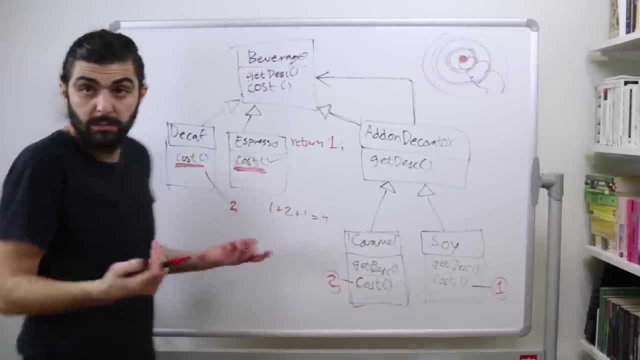 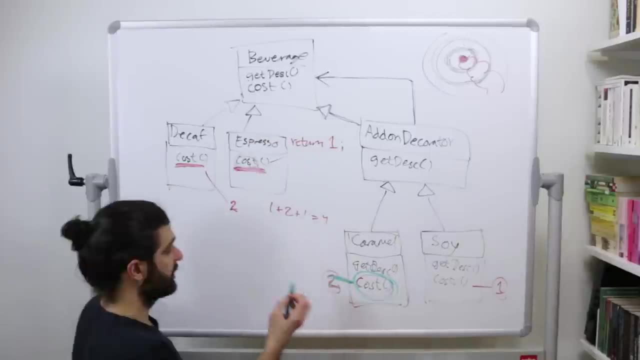 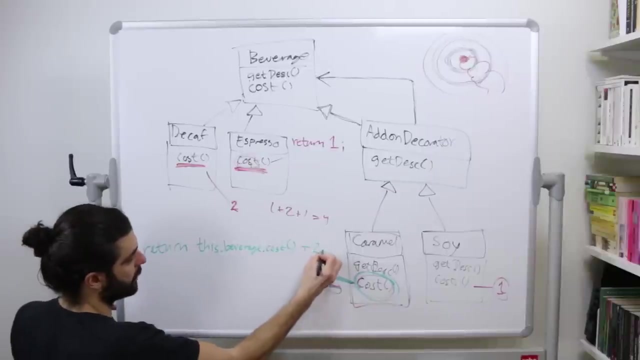 That would be the implementation of the cost method and saving your return to implementation of that method. But the cost method here. what that does is that It would say something like: remember that the cost of it is two. So you would say something like: return this dot beverage, dot cost plus two. 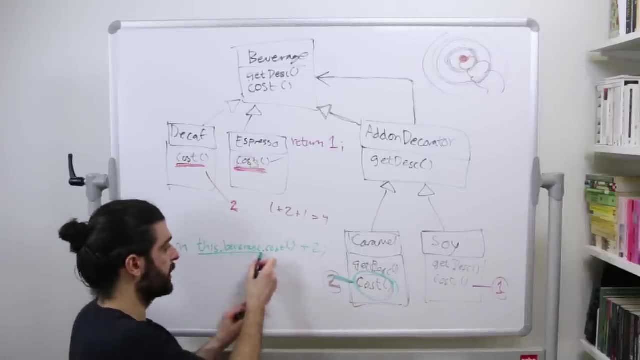 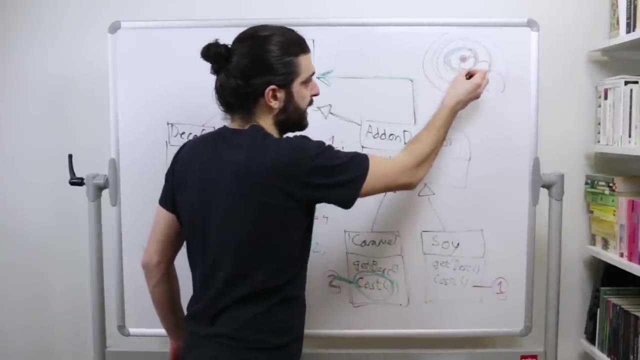 So this dot beverage? we haven't talked about this, but this dot beverage refers to the fact that it has a beverage. This thing wraps another thing and when this thing says this dot beverage, it refers to this thing. When this thing says this dot beverage, it refers to this thing. 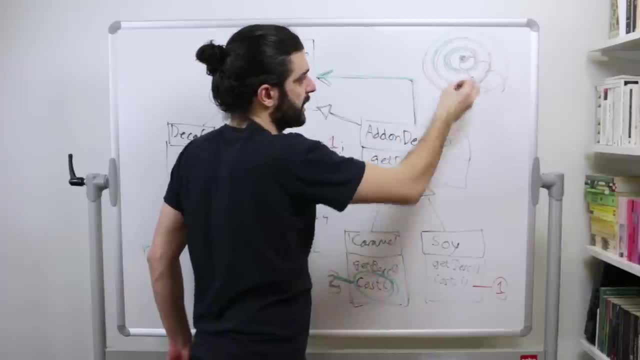 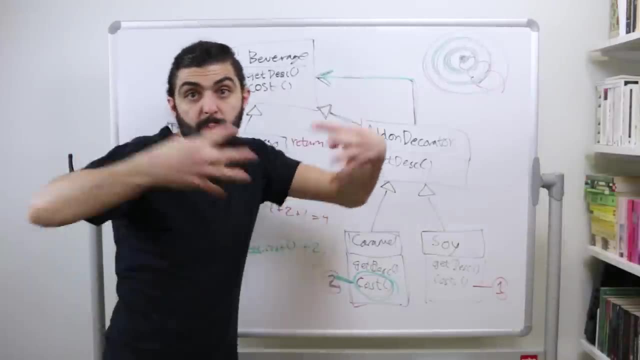 When this outer thing says This dot beverage, it refers to this thing. So from the outside it refers inwards, So it refers to the thing it's wrapping. The decorator refers to the thing it's wrapping And in this case, the thing it's wrapping happens to be another decorator. 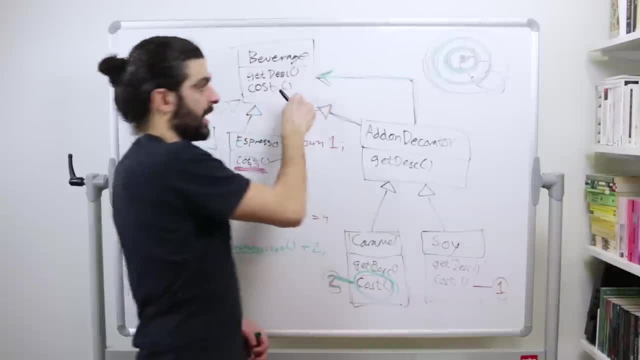 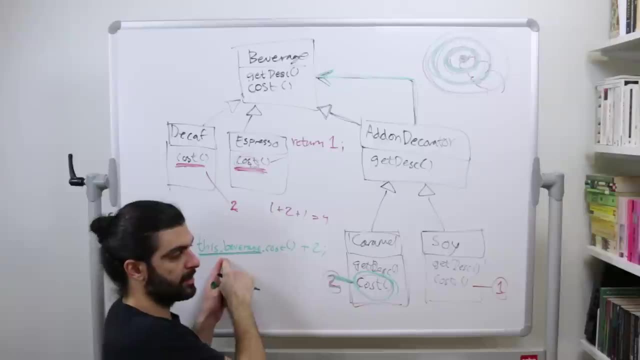 But this thing, when it refers to its beverage, it happens to be an actual beverage. So that's what we're saying: Get the cost of the thing I'm wrapping, because my cost is supposed to be added to that cost. Right, We're saying, plus, here, it's supposed to be added to this cost. 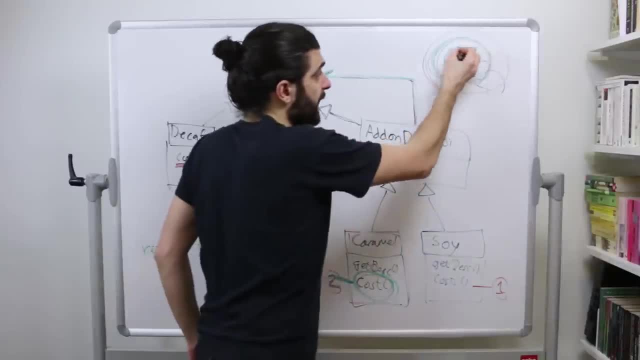 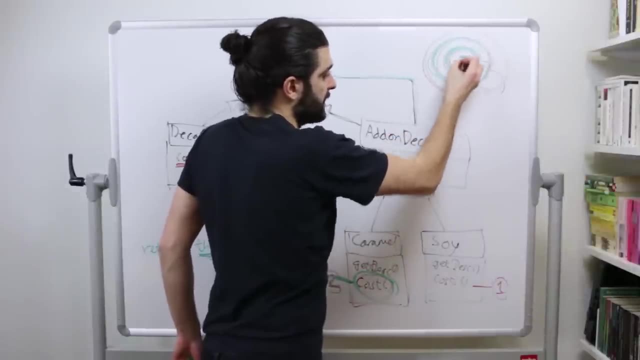 We take the Baseline cost, which could be, which is the baseline cost if we're here, Right, If we're here, this dot beverage refers to this, which is the baseline cost. But if we're here, it refers to this cost plus this cost. 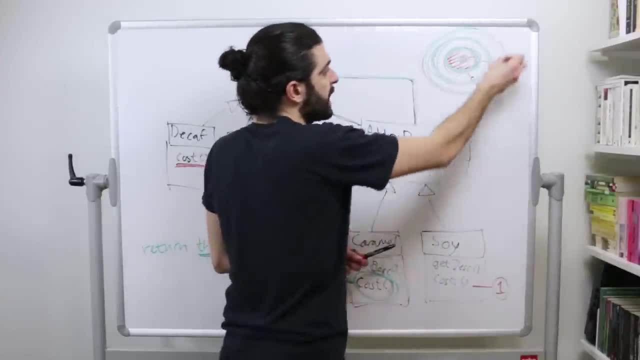 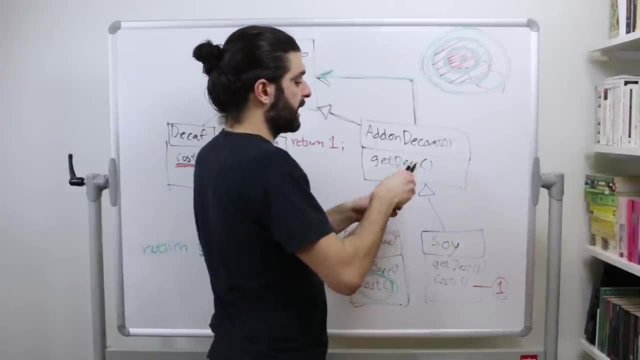 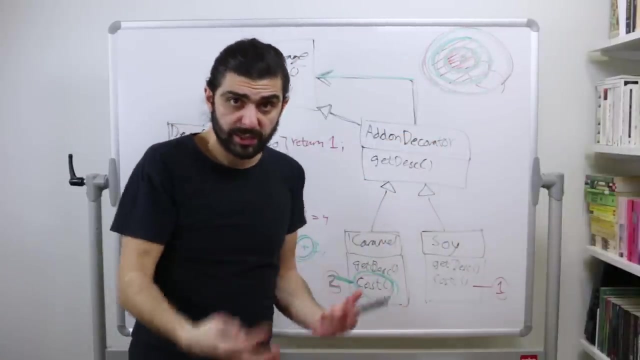 So essentially this stuff, and if we're here on the outside and we say this dot beverage, dot cost, we're referring to the cost of this stuff, of the total price of the thing that you are wrapping. Because if you think about it, this thing, this outermost thing, only knows that it's wrapping something and it's agnostic to what it's wrapping, as long as 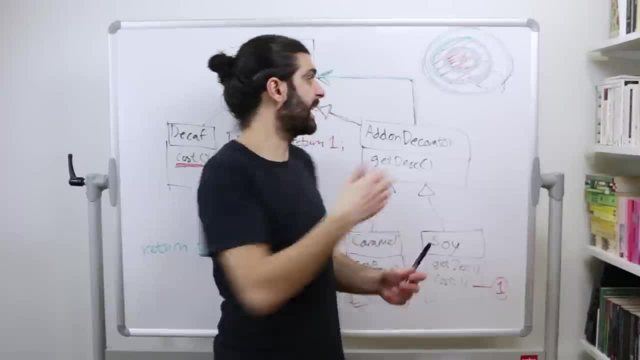 it's Of type beverage. it wraps something that's of type beverage and it has no idea whether the thing that it's wrapping actually also is a decorator that wraps the thing, that wraps the thing, that wraps the thing, et cetera, et cetera, et cetera. 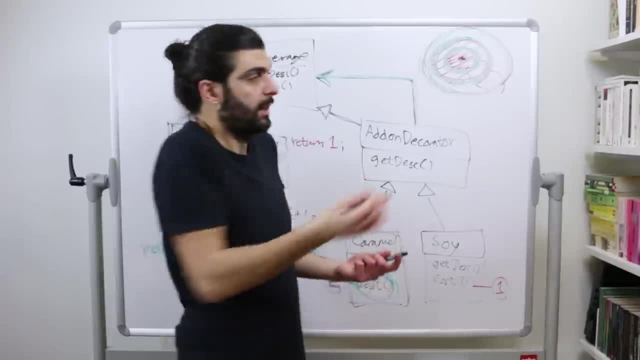 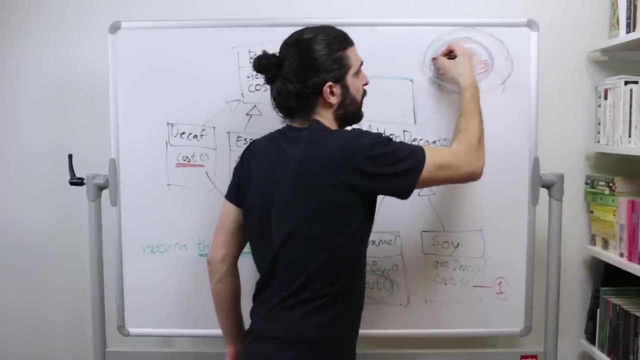 And then, at some point down the chain, you end up with a beverage. it has no idea, it just knows that it wraps something that calls itself of type beverage, and then it says, OK, give me the cost for your thing. So it's like a black box, right? 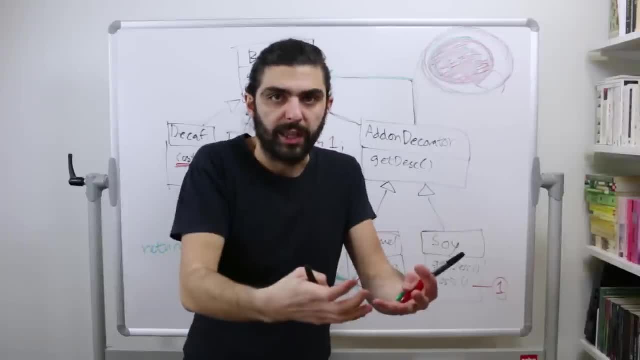 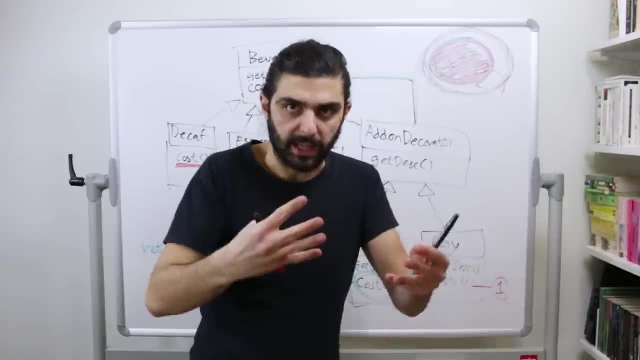 Every decorator thinks that it's only wrapping a single thing. but that single thing might also be a decorator that thinks that it's wrapping a single thing, And that thing might be a decorator that thinks that it's wrapping a single thing, and so forth, and so forth, and so forth. 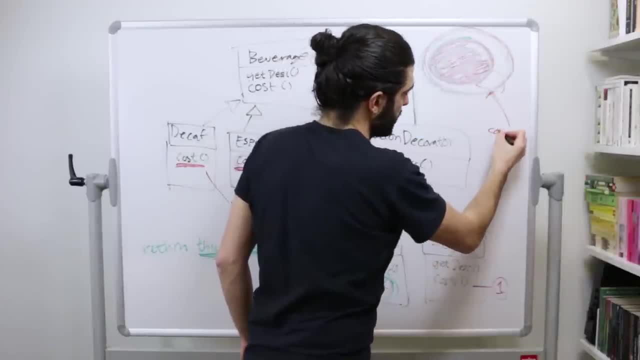 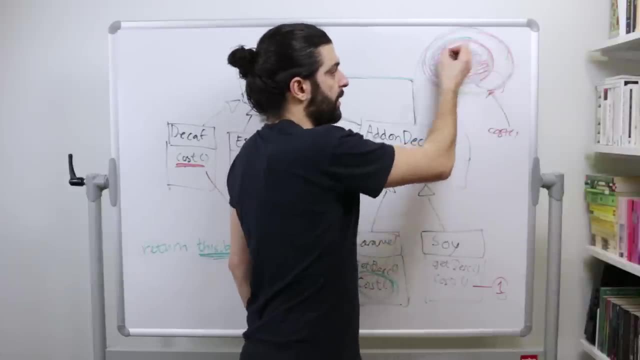 So when this thing, when you want to compute, when you ask this thing- hey, what's the cost? It says, actually, for me to be able to report the cost, I need to figure out what the cost is of the thing I'm wrapping and then add to that the cost that I have for myself. 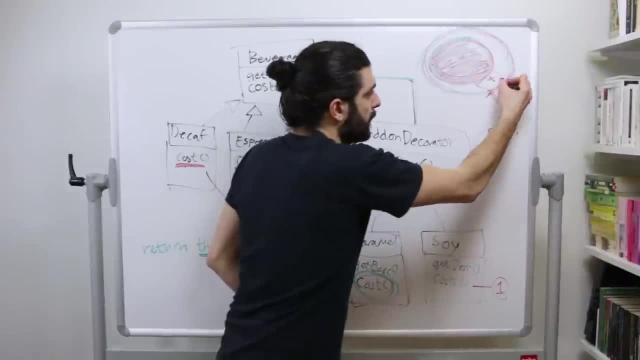 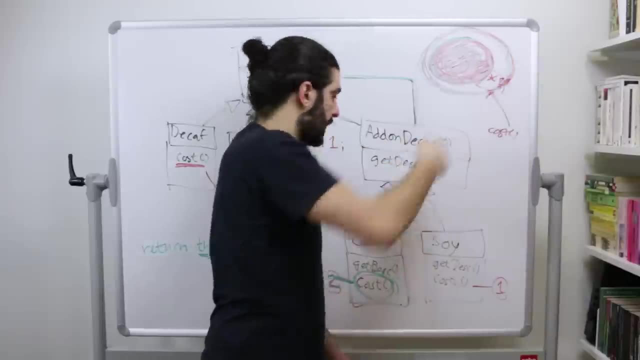 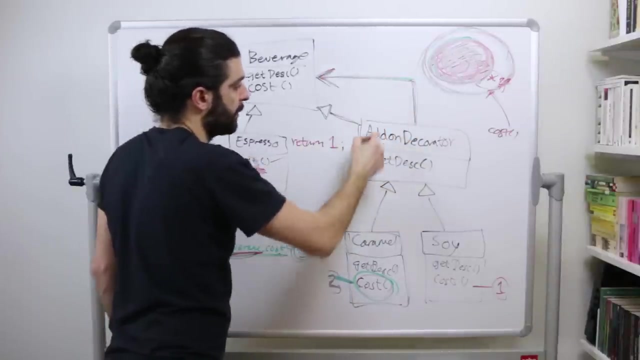 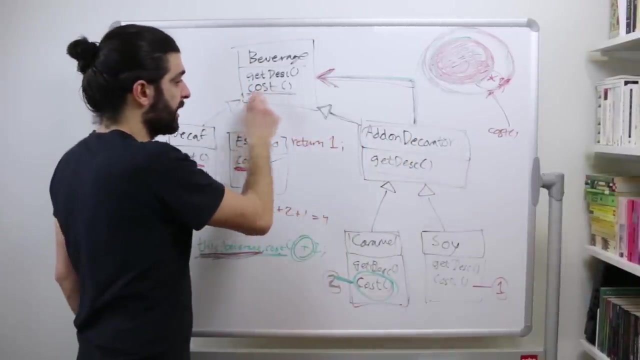 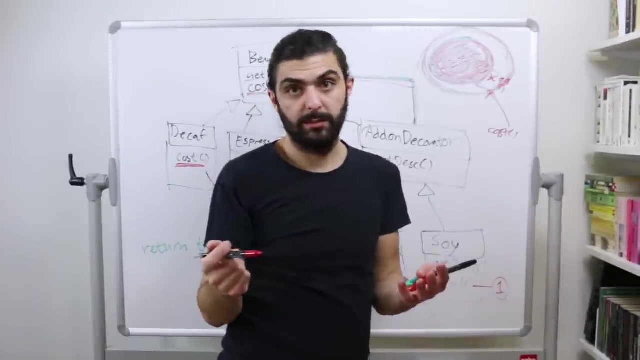 If this thing is caramel, then this thing should add the two. so it should say: what's the cost of this thing that I'm wrapping? and then let me add the two to that, Because that's the cost of the caramel add on, and this is why it says thisbeverage. let me return the price of the thing that I have. I am a decorator. I have a beverage which might be a decorator, it might be a baseline beverage. let me ask for the cost of that thing and then let me add whatever I want to that and get. description behaves in exactly the same way. essentially. the difference is, of course, that that works with strings and, as example, it's a way of composing together a name that represents the whole thing. 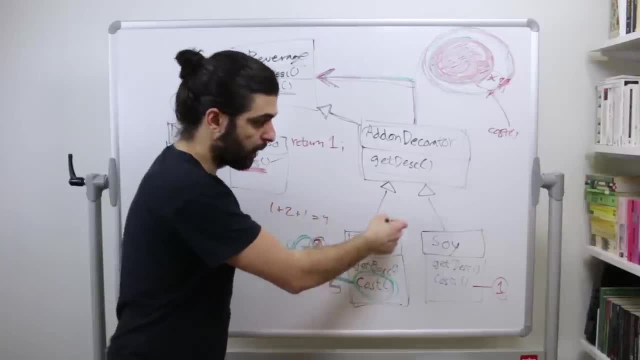 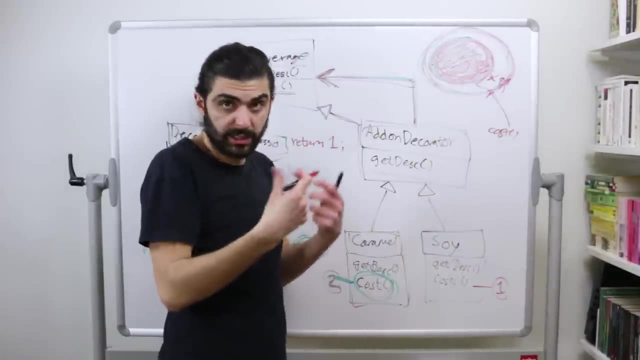 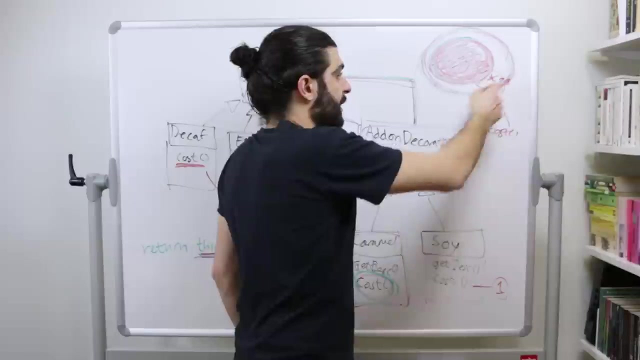 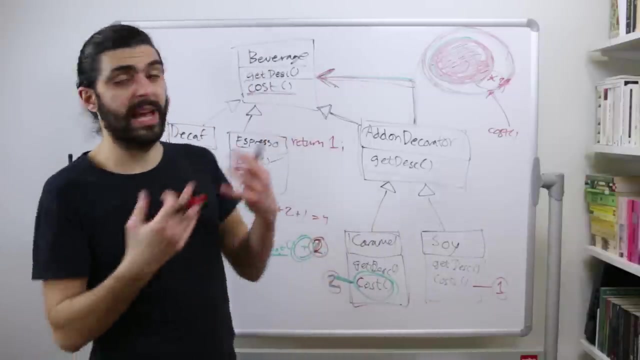 Beverage and, for example, could say espresso, colon, caramel, coma, soy or something like this. right, it's in some sense a way of iterating through this data structure. it's a way of traversing this data structure which is, by the way, if you're familiar with that, very similar to a linked list- it's no, that points to a node, that points to a node, etc. and returning and aggregating some kind of result. so when you get description, example, we aggregate the string and the cost, example, we aggregate a number. now let's look at the generalized UML diagram. so the generalized UML diagram, 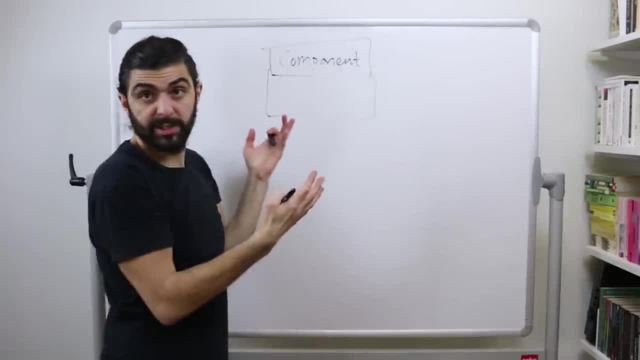 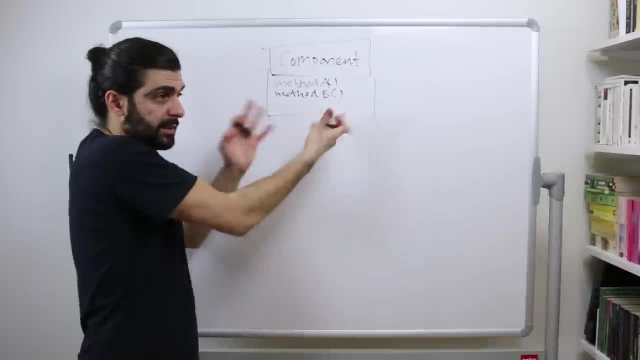 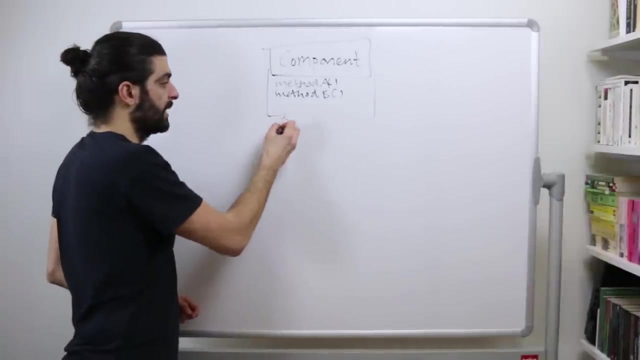 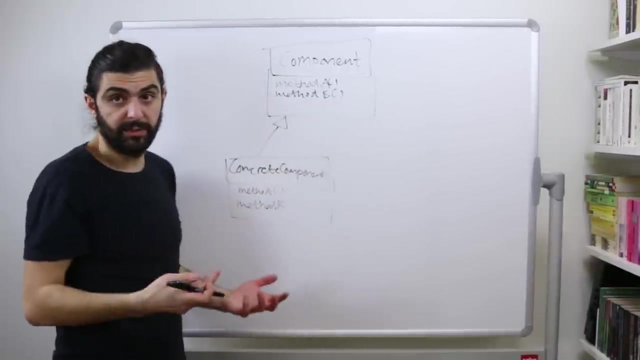 looks something like this: you have a component- in our previous case it was a beverage. you have some set of methods on this, so we'll say method A, method B. you can't define them here in the general case because it entirely depends on what you're actually building. you have some methods, so let's call them A and B. inheriting from the component is a concrete component which has method A and method B inheriting because it is a component. in our previous case we had an abstract class with a concrete class, but it could of course be an interface and a class. 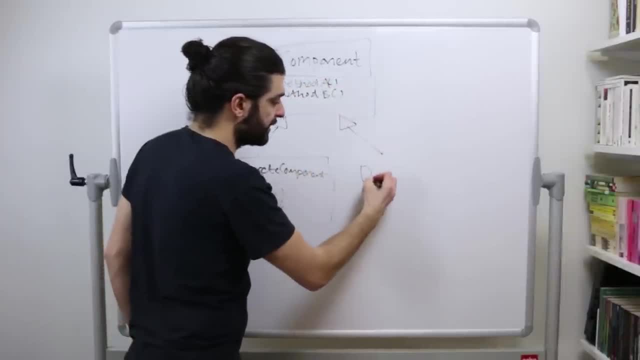 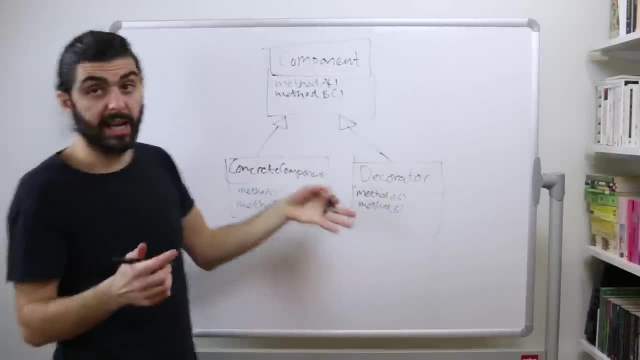 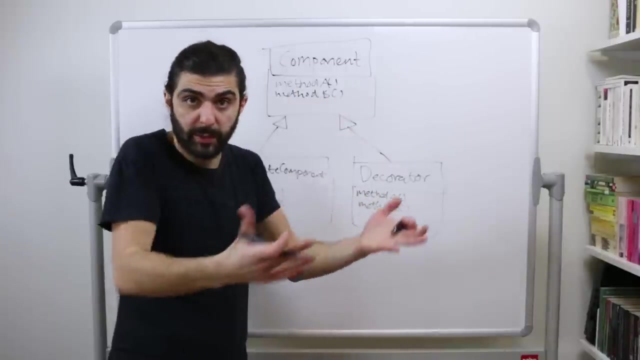 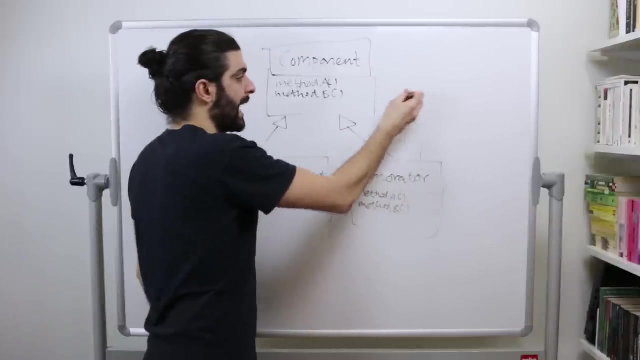 then also inheriting from this component is a decorator and the decorator of course also needs to specify method A and method B. but again, if it's an abstract class, perhaps it only overrides or defines some of the methods, because some of them it may want to use from the component- depends on your scenario- but because it's decorator pattern that we're looking at. the decorator not only is a component, it also has a component. so the decorator is a component, but it also has a component. 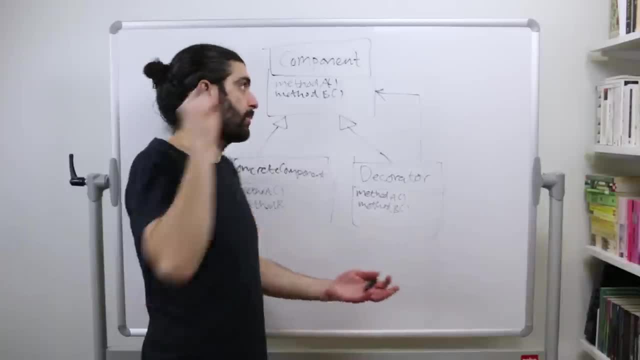 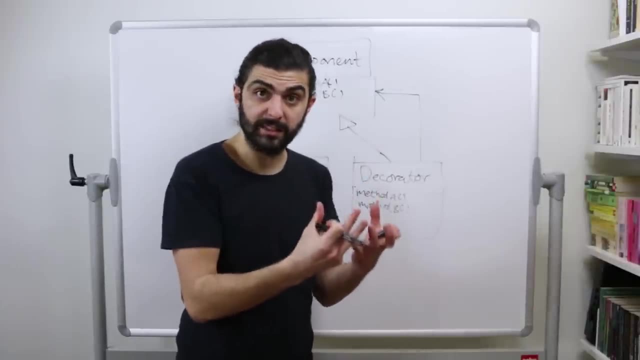 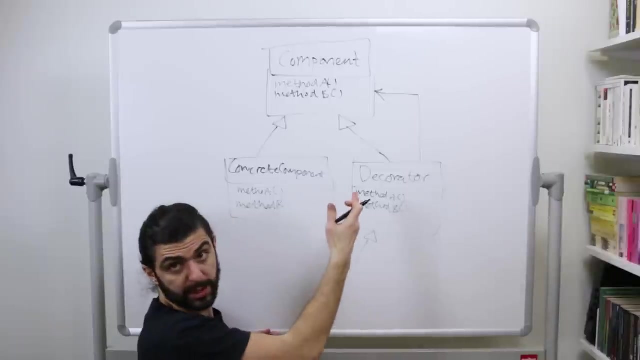 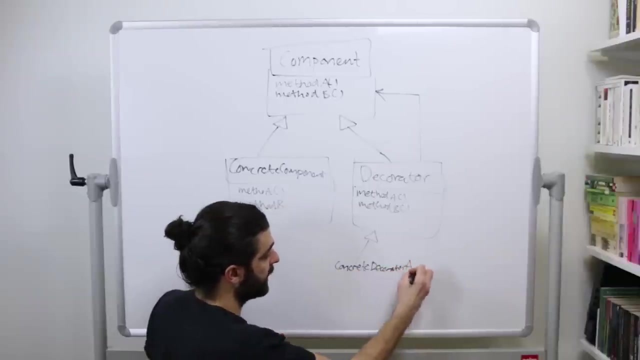 another component. so when you instantiate the decorator, you provided a component. so the decorator behaves as a component but also has a reference to another concrete component, and that component could be another decorator, because a decorator is a component and that's on the abstract level. so concretely, we of course need to have concrete decorators. so we have, hypothetically, concrete decorator A and concrete decorator B. let me actually rename these from A and B. 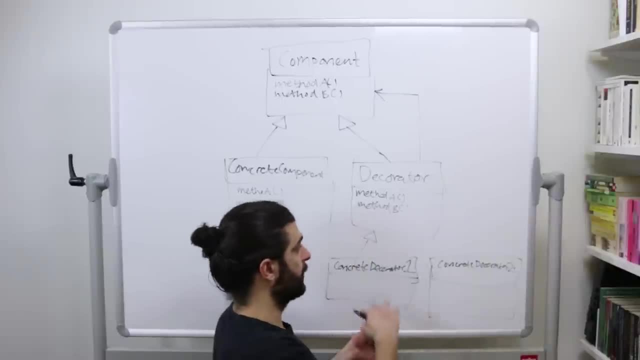 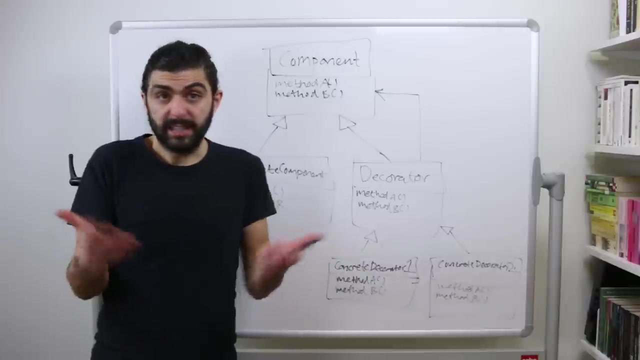 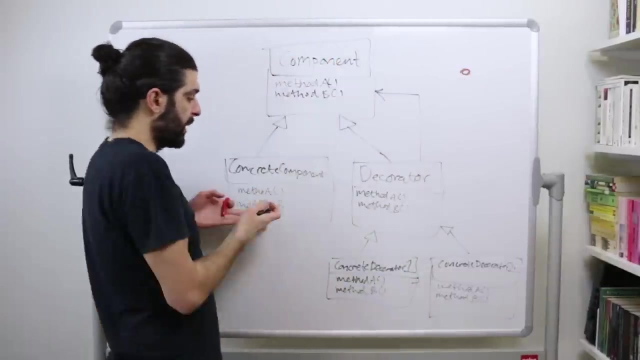 to one and two. just to emphasize that this A and B has nothing to do with the A and Bs in the method names. so these also have method A and method B. method A and method B and concrete decorator 2 is a decorator and that's it. that's the decorator pattern. you instantiate a component, you create an instance of a component. it behaves as a component but it is a concrete component because this is an abstract class. you can instantiate the abstract class or you can create an instance of a component. 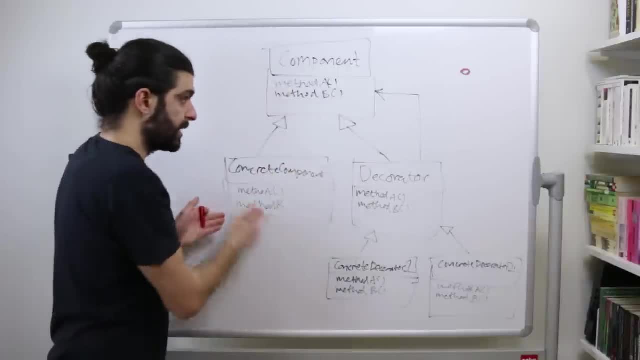 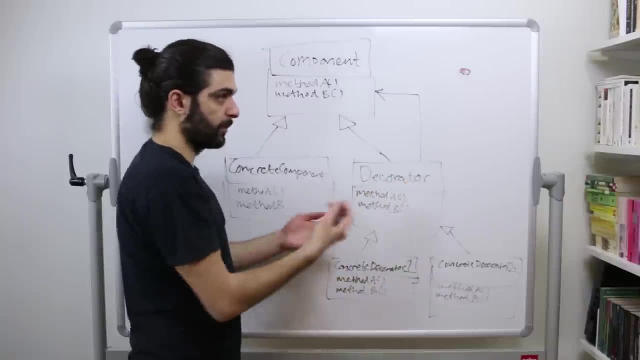 if this is an interface, you can't instantiate the interface. So you instantiate the concrete component. that's the concrete component and then you wrap that, you give that to some kind of decorator And of course, again, you can't instantiate an abstract decorator if this is an. 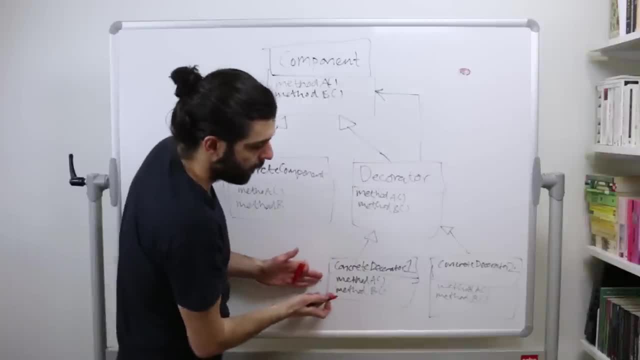 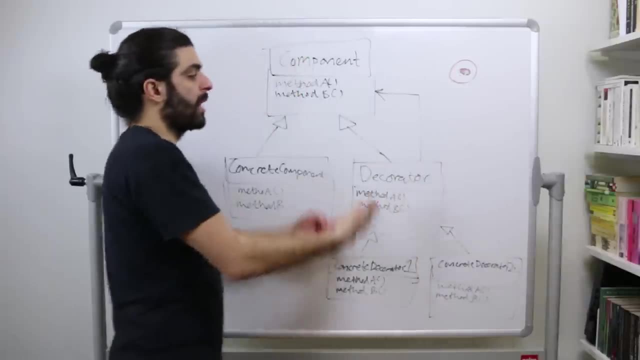 abstract class or if this is an interface. So you have to instantiate either this concrete decorator or this other concrete decorator And then, when you instantiate that concrete decorator, you pass it the component, And that's how you're wrapping that concrete component. So you're wrapping this. 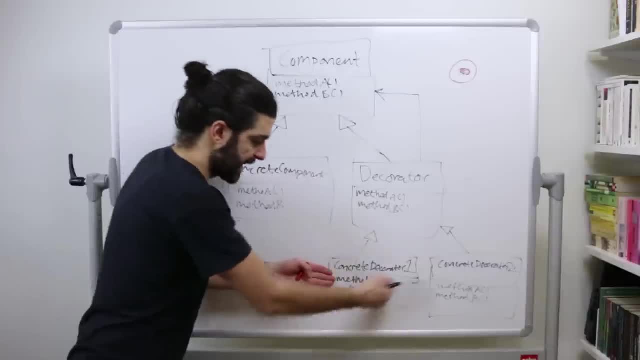 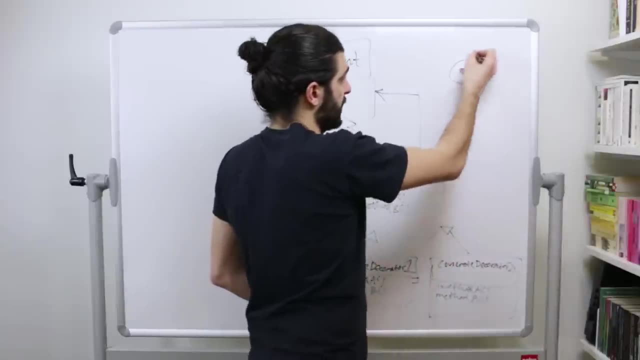 concrete component within this concrete decorator. So when you instantiate the concrete decorator, you pass it, the concrete component, And then perhaps you instantiate another decorator, perhaps the concrete decorator 2.. So you instantiate the concrete decorator 2. And when you do that, you pass it the instance of the concrete decorator 1, which was wrapping the 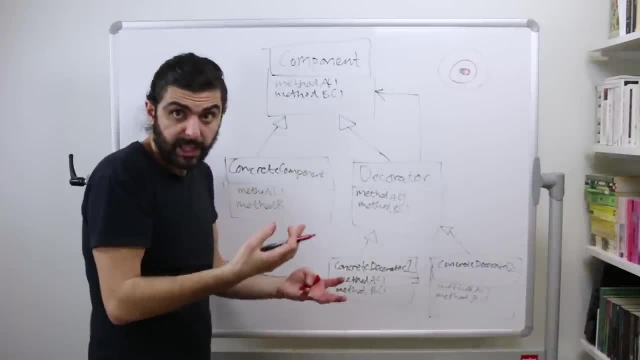 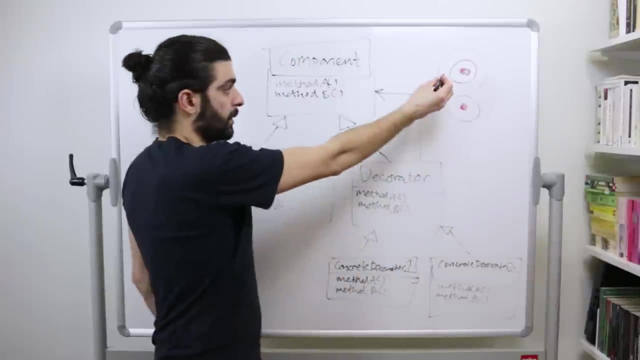 concrete component. And of course you wouldn't have to do that because that's the power of the decorator pattern. You could instantiate the concrete decorator 2 and pass it the concrete component. So you would have something like that. So maybe this is the concrete component. 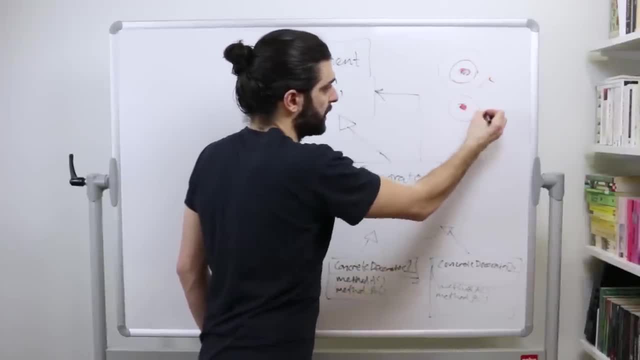 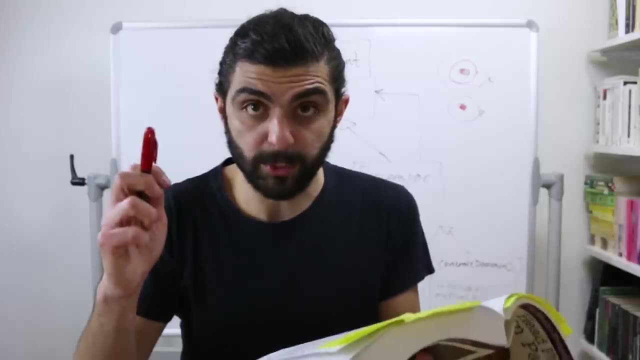 and this is decorator 1, and this is decorator 2.. And this is the concrete component and this is decorator 2.. That's the flexibility of decorator pattern. You can, at runtime, compose these in any way you want. So before we look at some code in 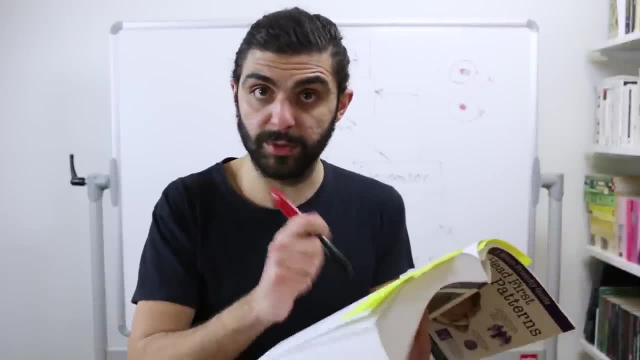 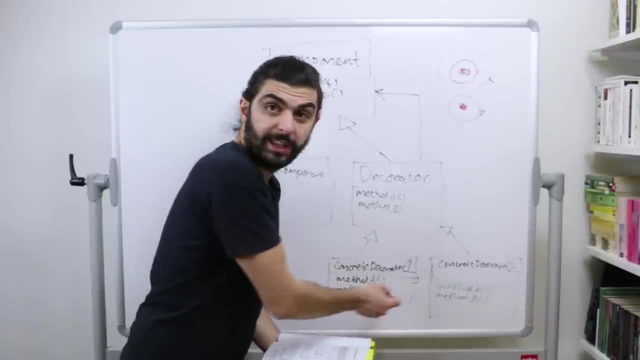 order to wrap this up, let's just quickly go back to the definition from this book. So the book said that the decorator pattern attaches additional responsibilities to an object dynamically. So these are the additional responsibilities We're saying. this defines some kind of additional. 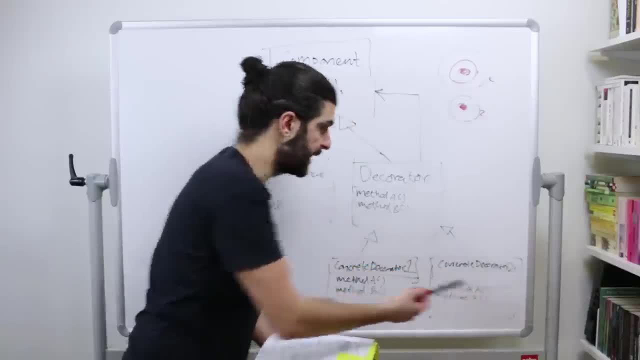 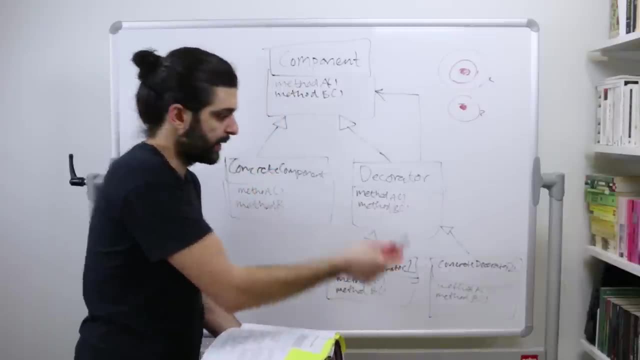 responsibility and this defines some other kind of additional responsibility And when you have this object, you can add additional responsibilities to it. So you can add additional responsibilities to this object. you can attach this additional responsibility dynamically to this object, or you could attach this additional responsibility to this object. But, moving on further, 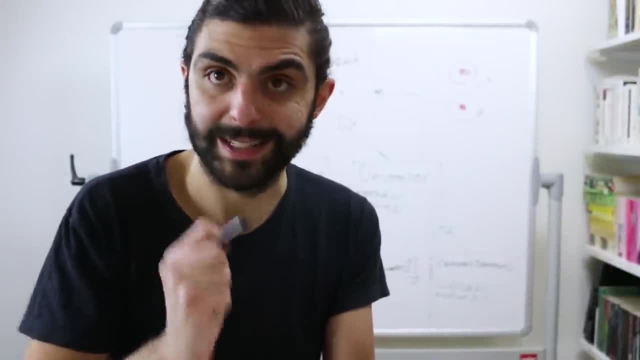 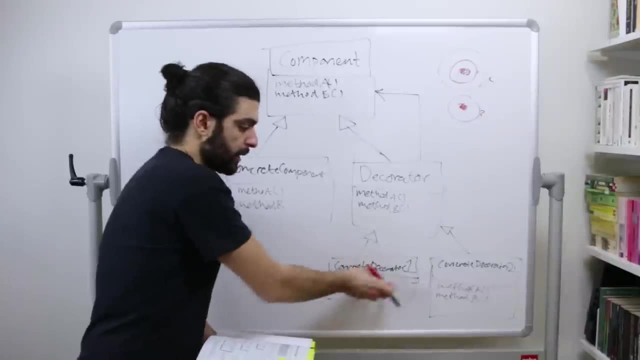 decorators provide a flexible alternative to subclassing for extending functionality. So it's not just that you can take the concrete decorator and endow the concrete component with the power of the concrete decorator. It's very, very flexible because, as we were saying before, 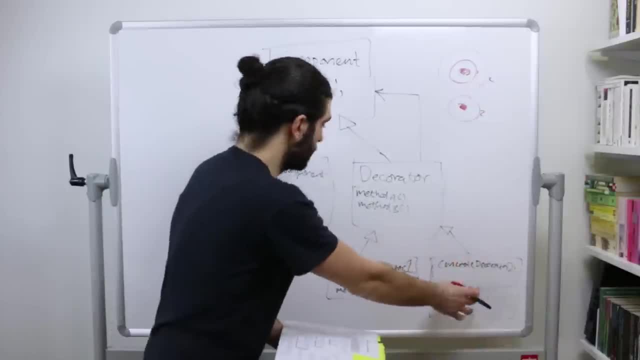 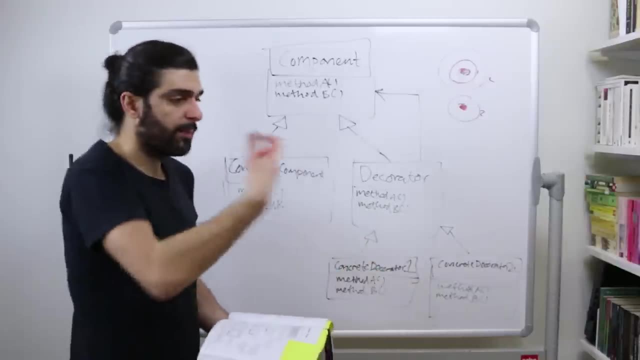 when we were talking about this. you can take the concrete decorator 1 and also the concrete decorator 2 and endow the concrete component with both of them. Or you could take the concrete decorator 1 and create 10 instances of it and wrap them in each. 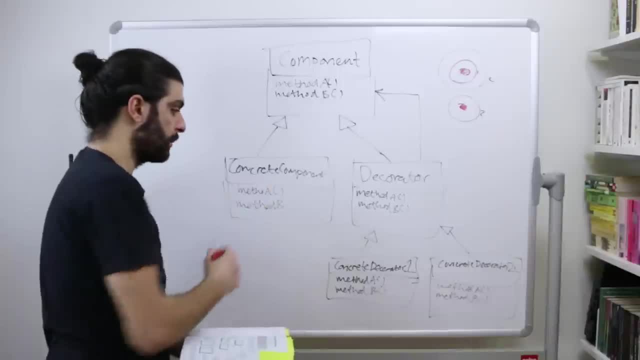 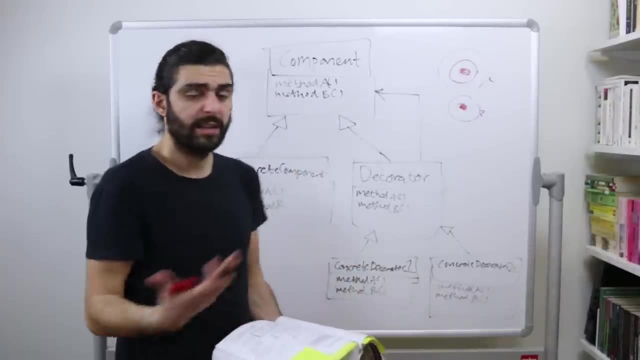 other and then the bottom wrap it around the concrete component. So you have a concrete component that's endowed with 10 concrete decorator 1s And in some scenarios, in some applications that might make sense, In some applications that might make no sense, For 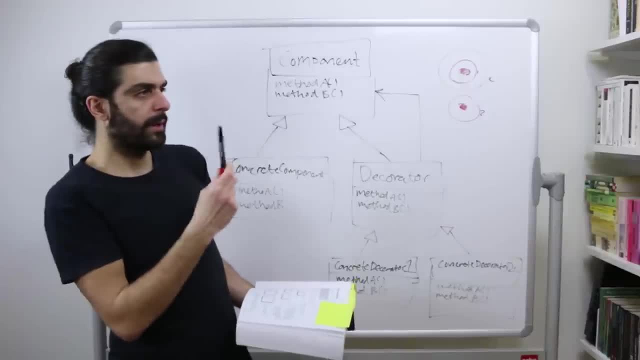 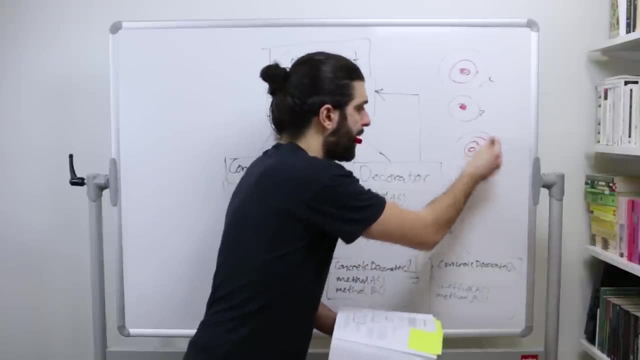 example, think of the cost method that we had before. If the cost method were multiplying and if the cost of concrete decorator 1 was 1, then it wouldn't matter if you were wrapping multiple 1s, Because if the decorators that you're wrapping all multiply, 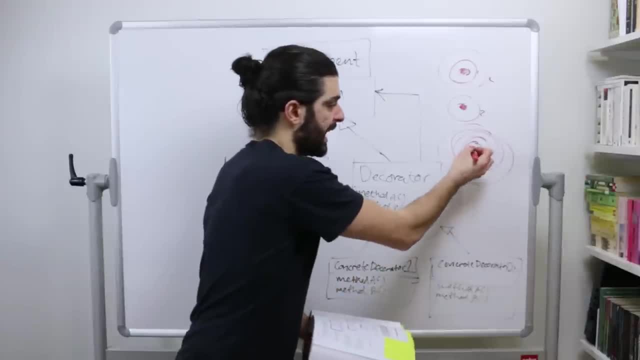 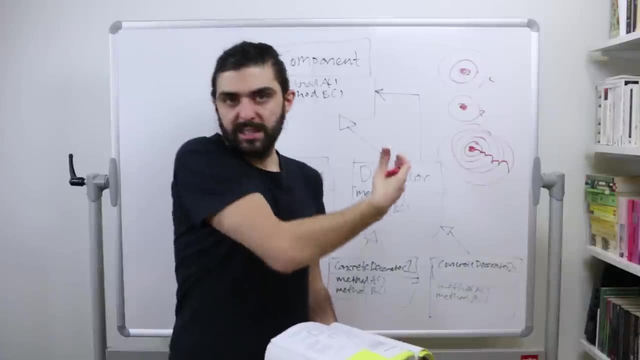 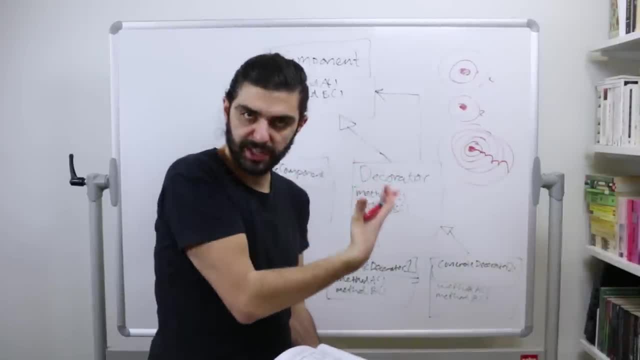 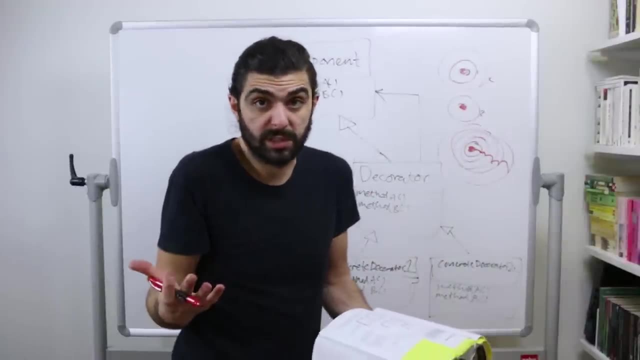 no sense. But the decorator pattern is completely agnostic to your scenario. So syntactically, programmatically, you can do that, You can wrap it just as many times as you want, But in some scenarios it's just not meaningful. But essentially, I think this is how they're thinking when they're 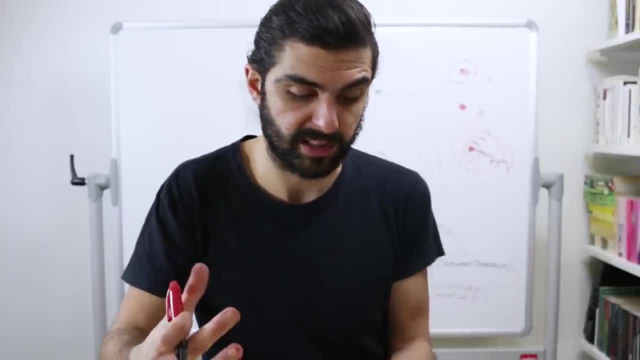 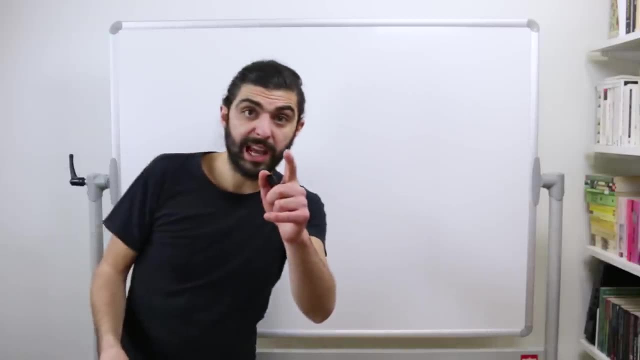 saying that it's a flexible alternative, Because it's actually very, very flexible, Because you can use them in any way you like. Let's now, super quickly, look at a code example. Let's stick with the coffee example. So we'll start with the abstract beverage class. So we'll say abstract. 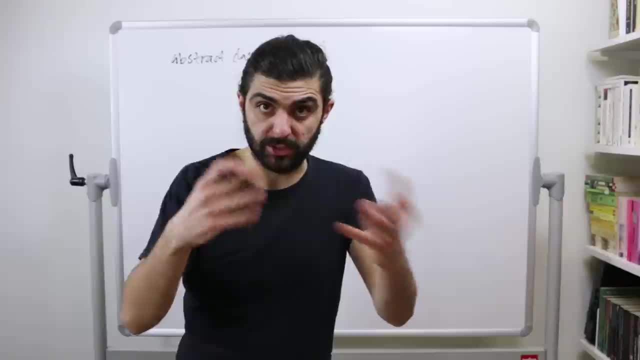 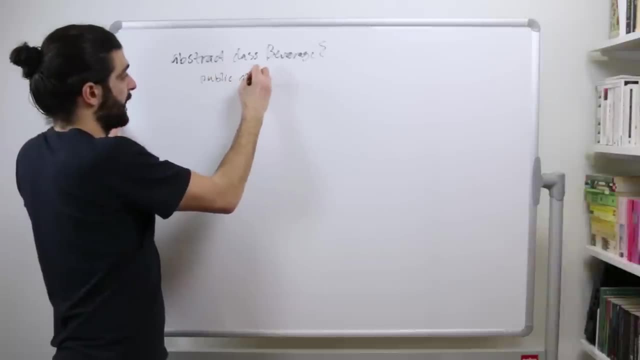 class beverage open, And I'll skip the description methods just to keep things short. So remember that I'll only do the cost methods. So because of that, we only have public abstract cost, the cost method. Remember that because it's an abstract class and we don't want to give cost. 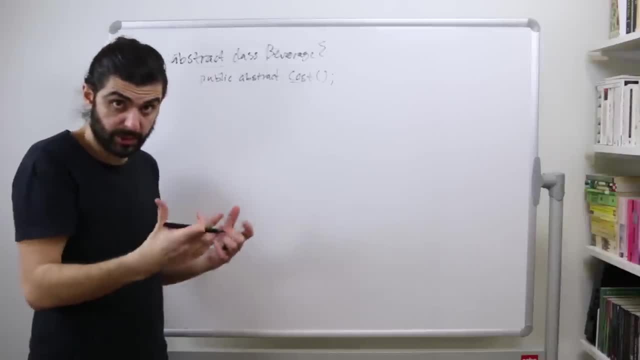 and implementation here in the beverage class because we don't have a baseline cost for beverages. We need to know which type of beverage it is And we don't want to give cost and implementation here in the beverage class. So we declare it as abstract because then we're 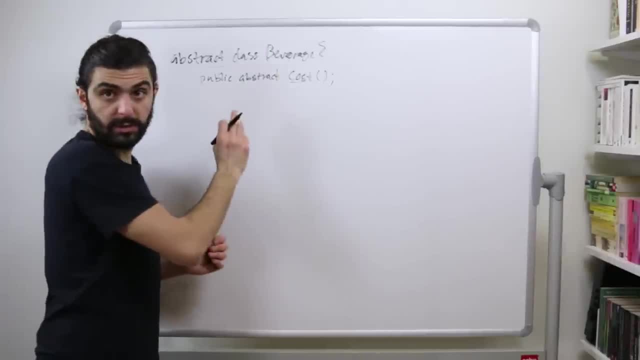 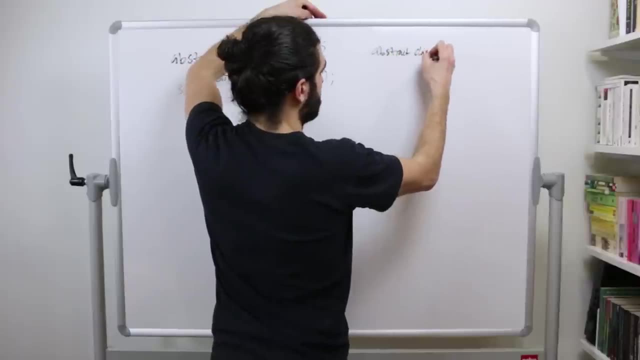 saying that whoever subclasses beverage has to give an implementation of cost. That's that for the abstract class. And then let's do the add-ons, In other words the decorators. So then we have abstract class, add-on decorator. I'm running out of space here, but continuing on the same line. 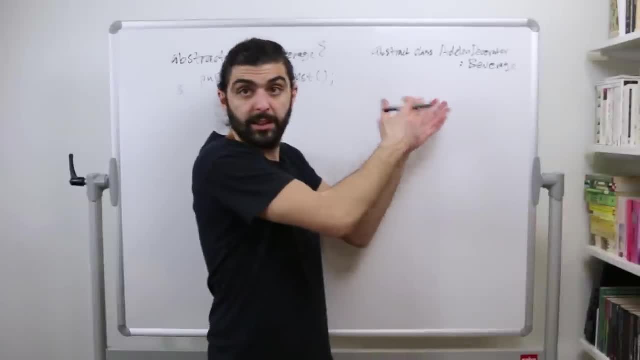 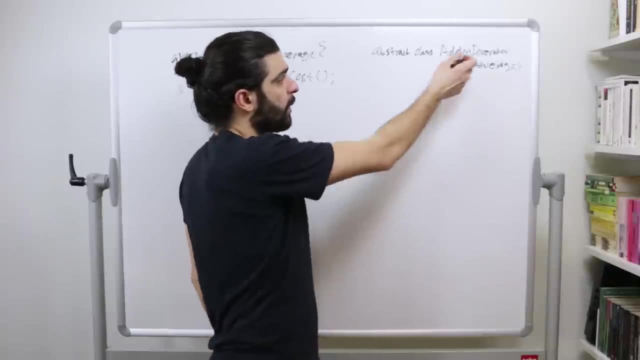 is of type beverage Because, remember again, the decorator is a component, So it is a beverage, And the implementation of that is just that the abstract class is stating that if you are an add-on decorator, then you have to give an implementation for cost Because, again, there is 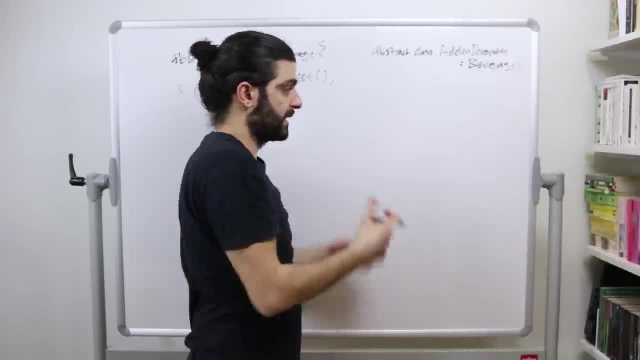 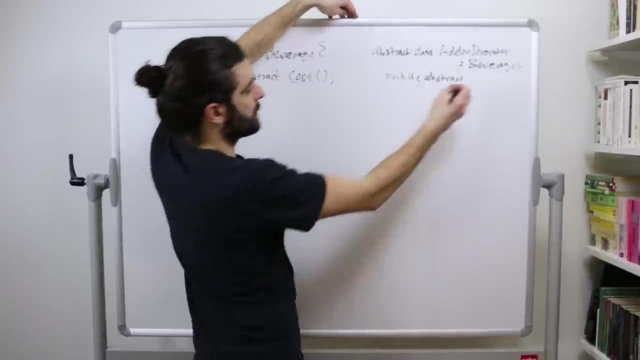 no baseline decorator. This is only so that we can have the same type of all the decorators. So that's why we're saying that they need a public abstract method called cost. And again, no implementation. So in this particular scenario, just to be a bit more complete, of course we don't actually need 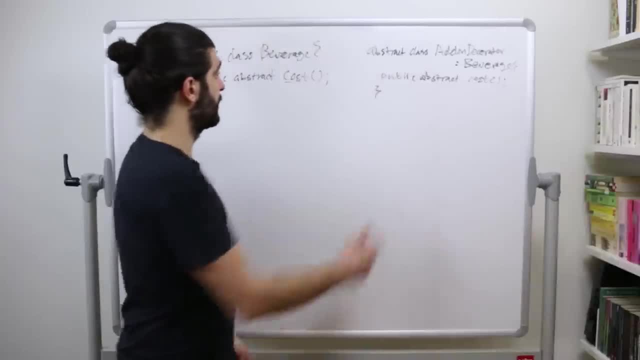 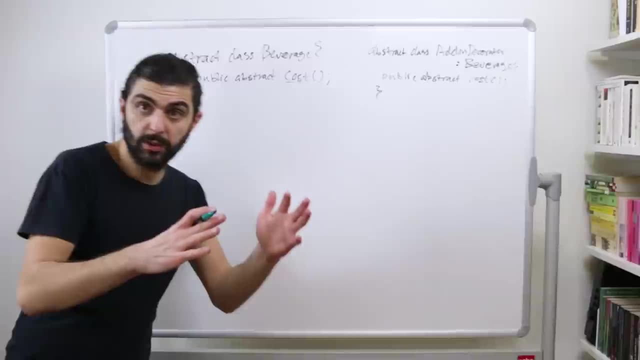 the add-on decorator. We could just say that all of the decorators behave as beverages and have beverages. Moving on to the concrete implementations, A concrete beverage. let's only look at espresso. Remember, we had decaf and we had espresso. But 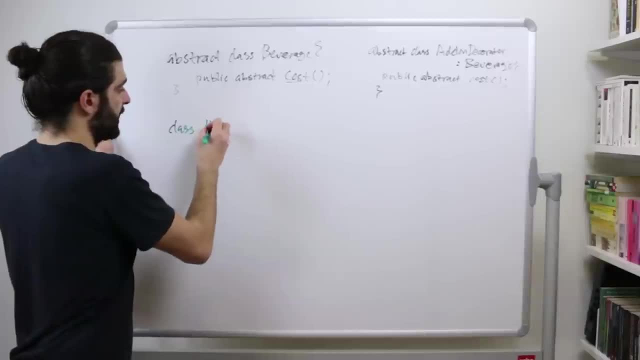 let's now only look at espresso. So then we have a class called espresso, which is of type beverage and has an implementation for the method cost. right, Because it's a beverage, it needs to implement the method cost, So it has a public. I, of course, I forgot the type here. I forgot 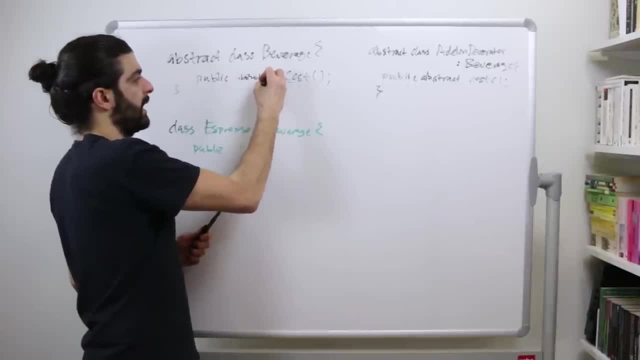 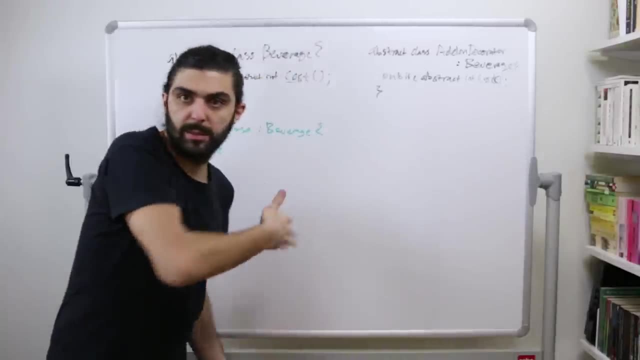 the data type here. So let's actually quickly add that public abstract int cost and public abstract int cost. Probably it makes sense to use a double or something like that, But let's just keep it stick to ints. So the espresso needs to have an implementation for public int cost. It needs to. 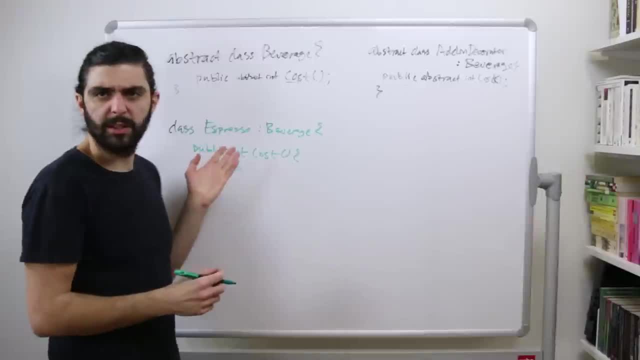 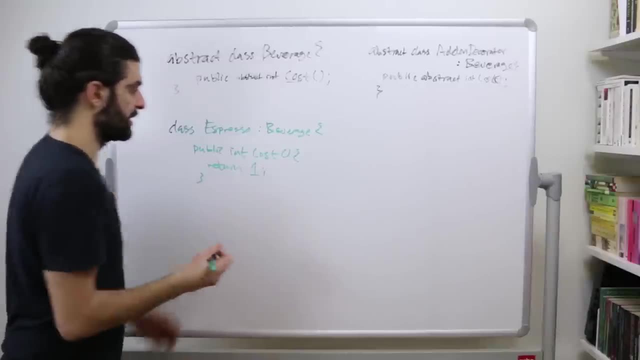 have an implementation for the cost method. And what do we return? Well, I think before we said that the espresso has a price of one. So, because it's the baseline implementation, because it's the base case, because it's the innermost thing, because it's the actual beverage, then we actually 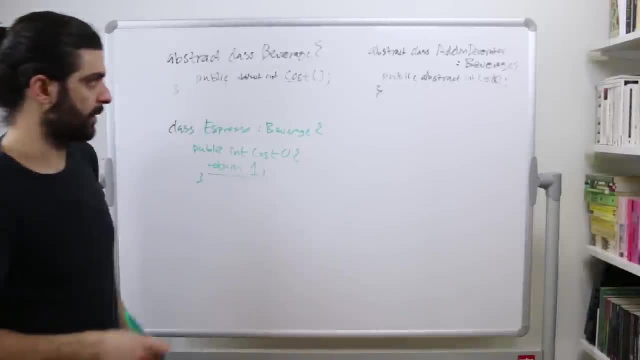 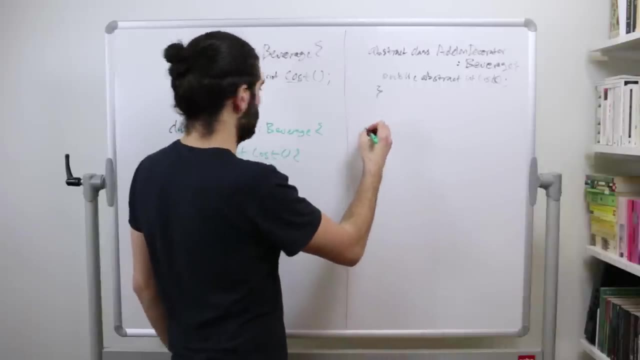 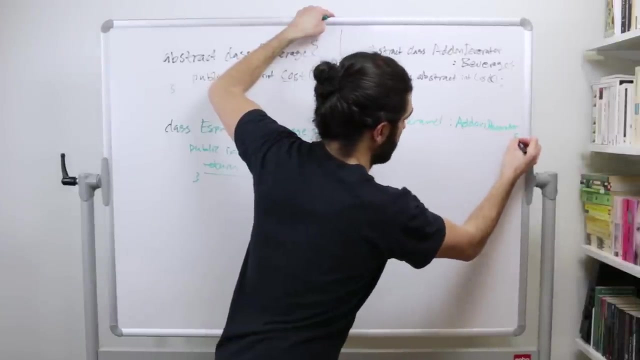 just return, whatever the price of that thing is. So let's say we return one, But what happens at the decorator end? So in the decorator end let's do the caramel. So then we have a class called caramel and that is of type add-on decorator running out of space. 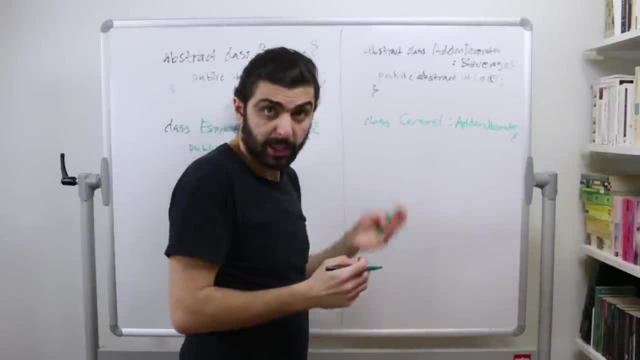 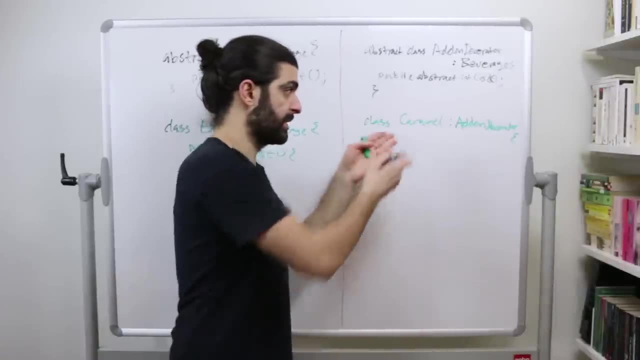 So the class caramel which, remember, is a decorator. So in a real world scenario, remember I said before I would probably call this caramel decorator, just to be explicit, so that when people see the word caramel they know that it's not just a standalone class, It's actually a decorator. that 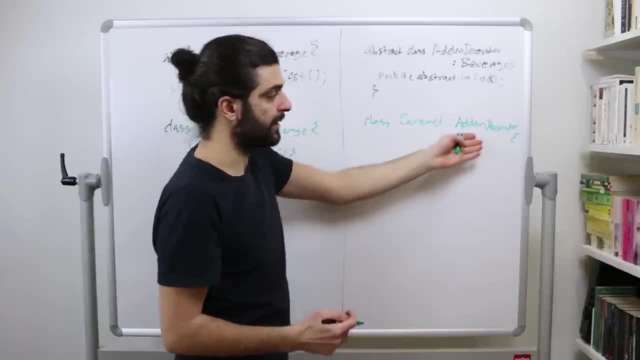 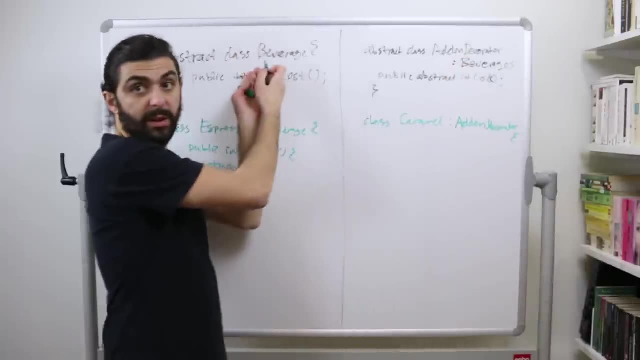 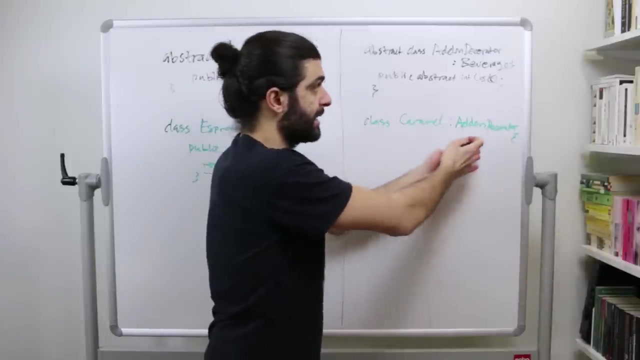 needs to decorate something. So the caramel decorator is a add-on decorator And the add-on decorator is a beverage. So, by proxy, the caramel decorator is a beverage. So back to that idea. the decorator is and has a component, And now we've only described that it is a decorator. 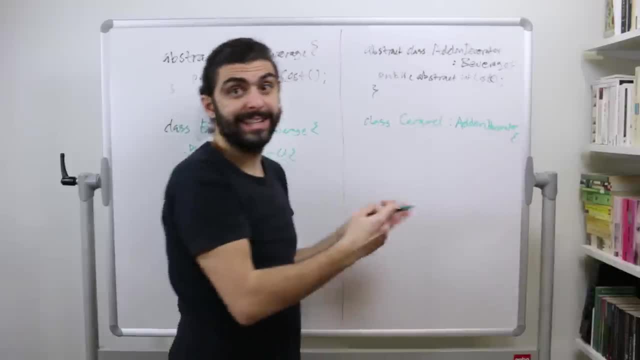 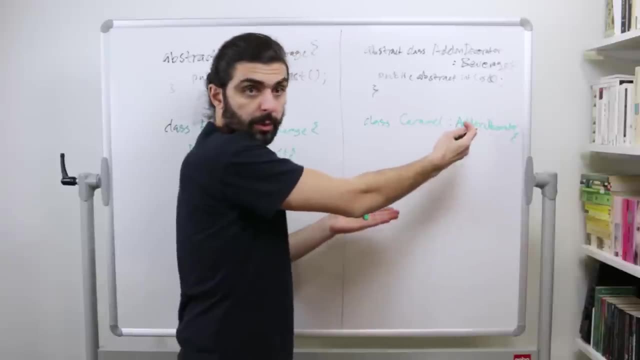 but because the decorator is a beverage, it by proxy is a component. But then to the has part, we say that a decorator has a component as well as is a component. So how do we describe the has a component? So we describe that by saying that it has of type beverage. 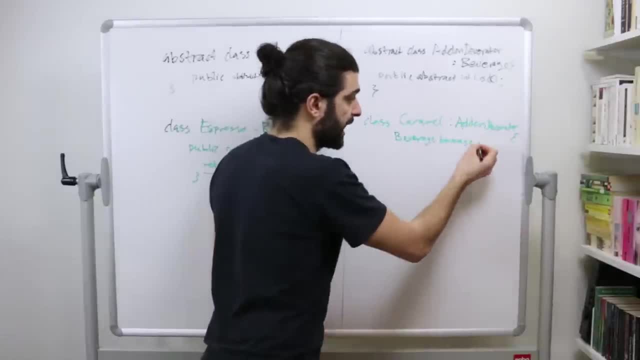 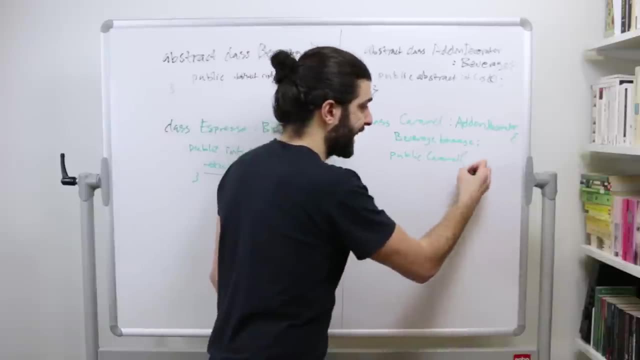 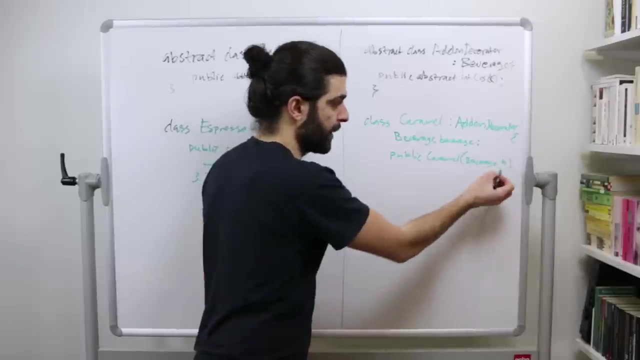 Let's call it beverage. And before instantiation we can't know what that is. So for the constructor public caramel. So in the constructor public caramel, we take an argument which is of type beverage- beverage, Let me just call it B, so that we can differentiate between the beverage that's. 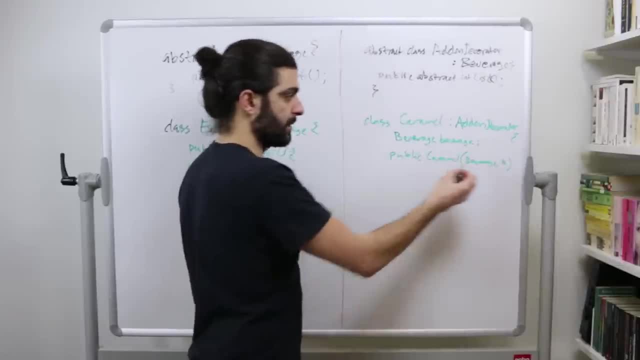 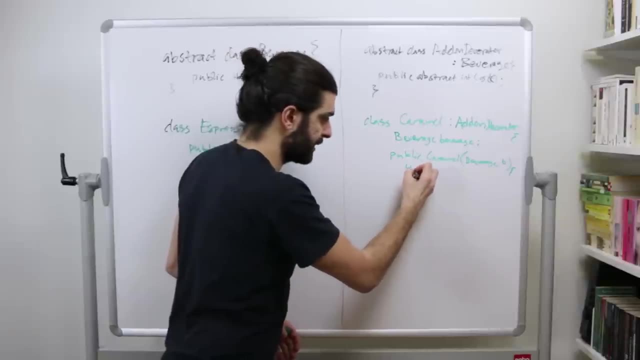 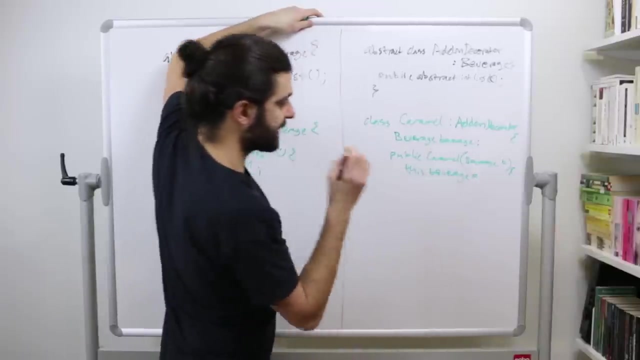 passed in through the constructor and the beverage that exists as an instance variable. So then, in the body of the constructor of the caramel decorator, we do what We say this dot beverage, in other words this instance variable beverage. we say this dot beverage and assign that the value. 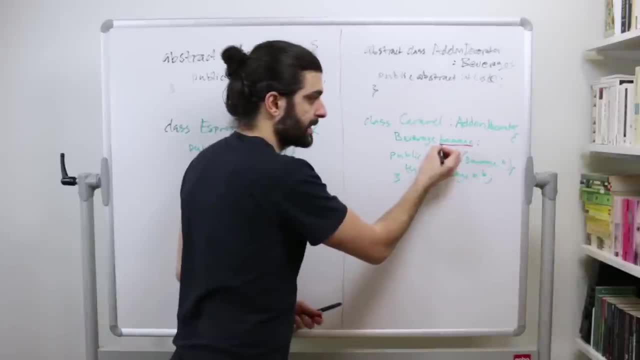 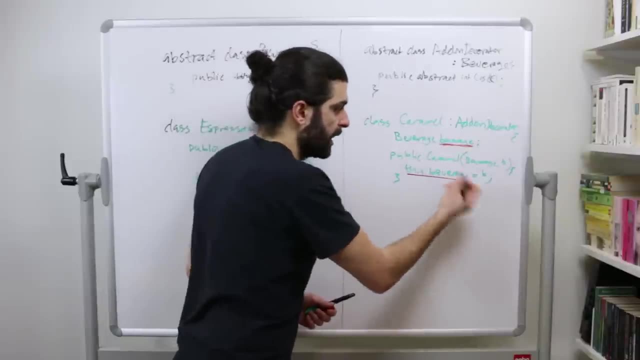 B, close the constructor. So what happens here? We assign to the instance variable beverage. Here we say this: dot beverage. In other words, we assign to the instance variable beverage. we assign it the value B and B is what was passed in here through the constructor. So we have a beverage. 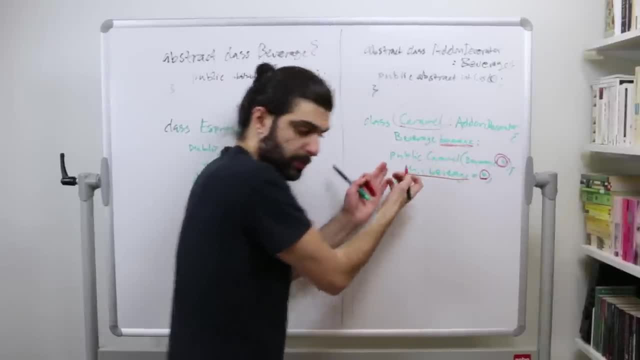 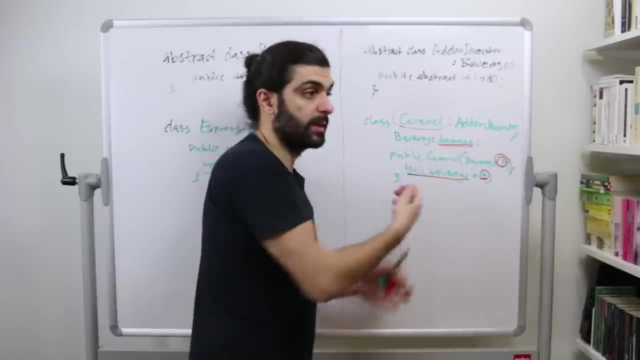 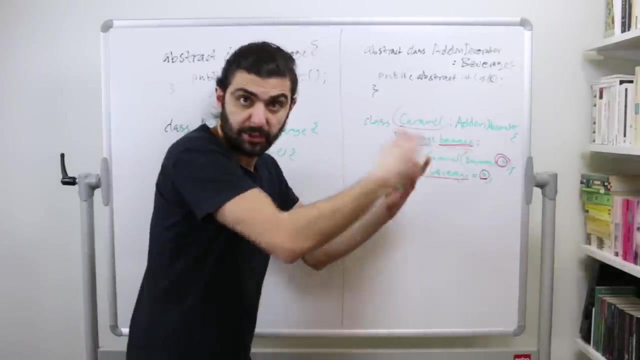 here in the caramel decorator And after construction, after we've instantiated the caramel class, we will have set the value of that beverage to whatever was passed in through the constructor. So again, the caramel decorator class has a beverage, has a beverage that's set. 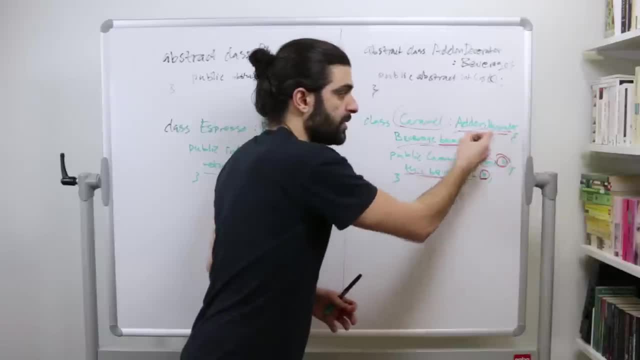 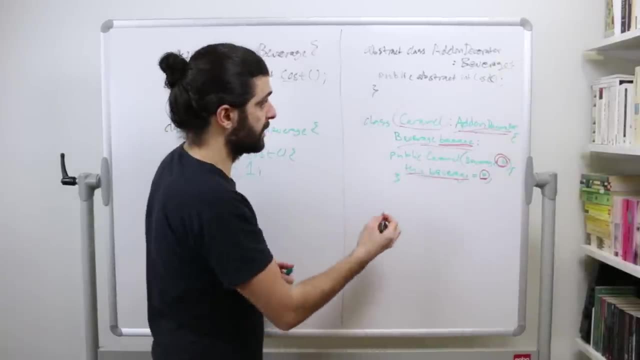 through the constructor, but also is a beverage, because here, by proxy, it is because it is a decorator and the decorator is a beverage And that was the constructor. But then now we have to also implement the cost method. So then we say public int cost, And what's the implementation of? 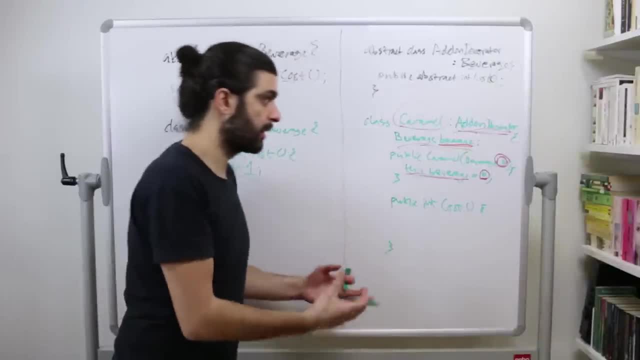 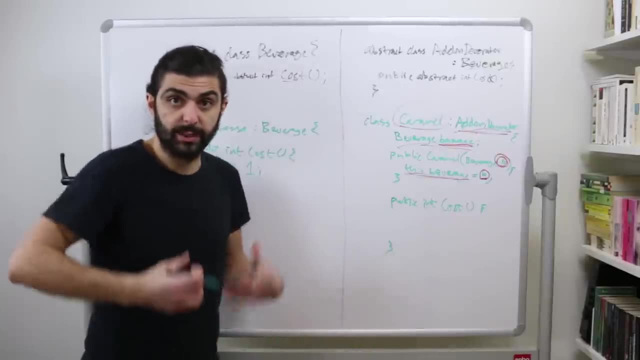 that. Remember we drew that before when we said that the cost method was the cost method. So now that the difference between the cost method of a decorator and a component is that the component is standalone, So the component can actually return its own cost, whereas the decorator cannot exist. 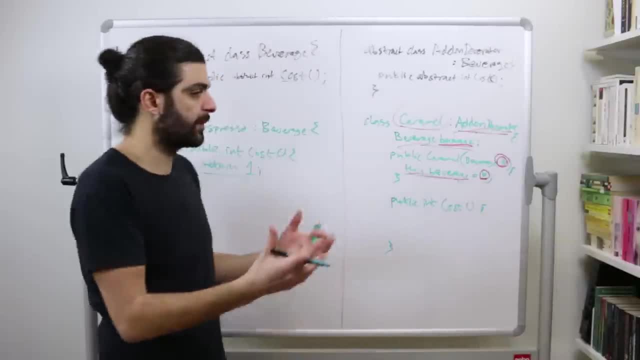 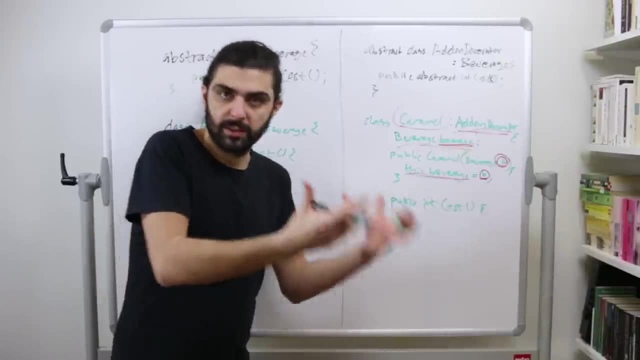 in isolation. It has to decorate something. It has to decorate either another decorator or it has to decorate a component. So that means that when we ask a decorator for its cost, it can't just stand alone report its cost. It has to report its own cost in relation to the thing that it's decorating. 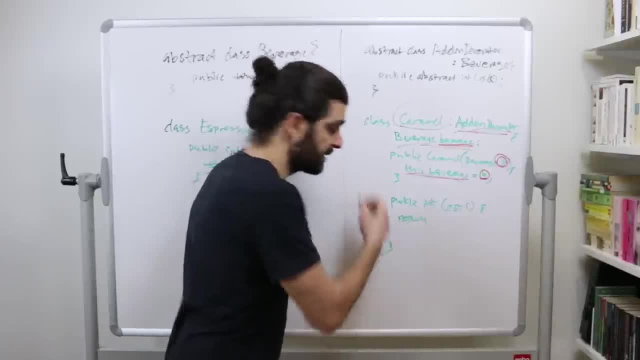 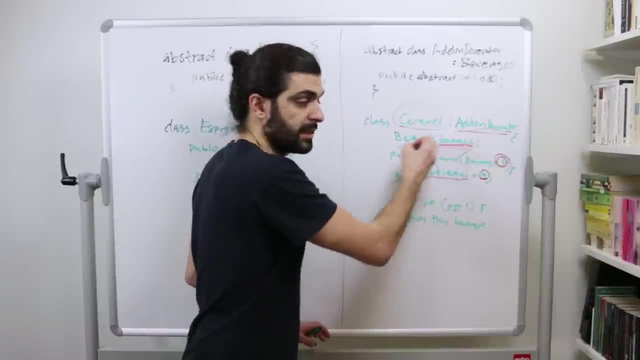 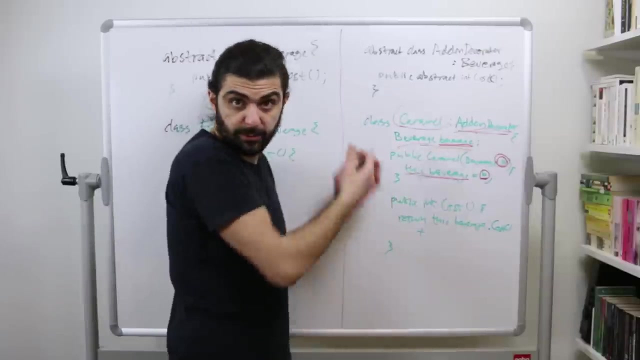 And that means, as we drew before, that we can't just say return some kind of cost here. Instead, what we do is that we say: return this dot beverage, this again, this instance variable beverage, this dot beverage, dot cost. In other words, calculate the cost of that plus the cost that's. 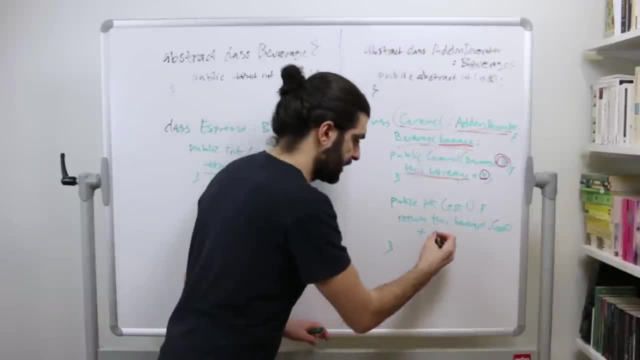 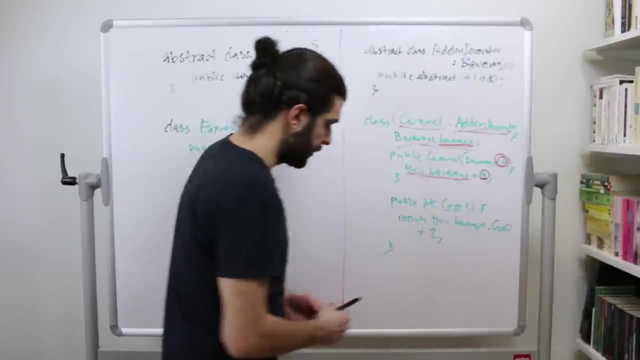 for this caramel decorator, And I'm not sure if I remember correctly, but let's just say that that cost is two, for example. Could be something else, right, I can't remember. that's the same as we had in the example before. So in other words, we take whatever the cost of the decorator is and we take. 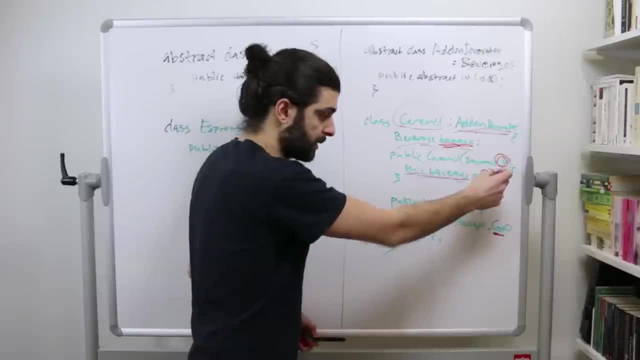 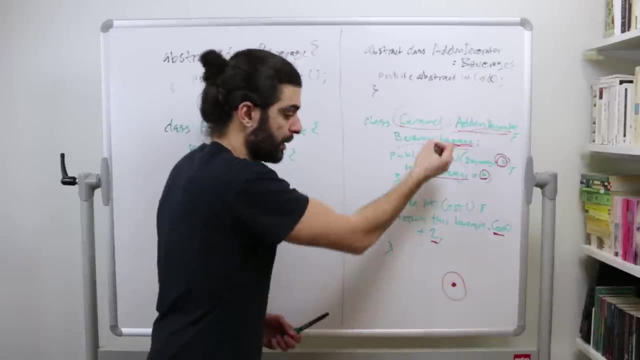 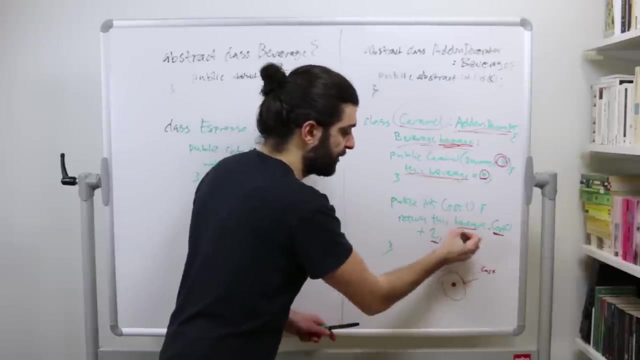 whatever the cost is of the beverage that were passed in through the constructor And we add to that two. So when you have some kind of beverage and then you wrap that with the caramel decorator, then when you ask the caramel decorator for cost, the caramel decorator will ask the beverage that 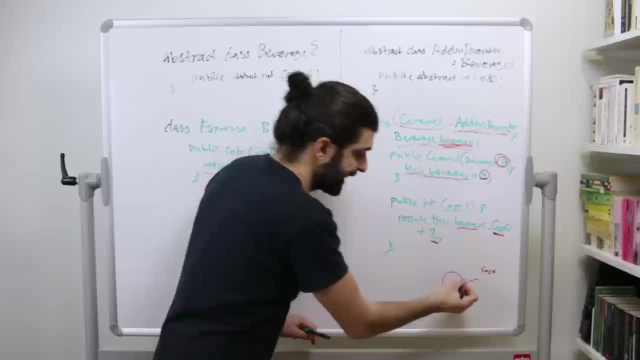 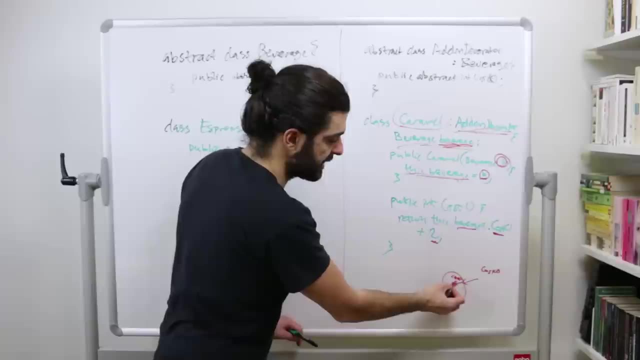 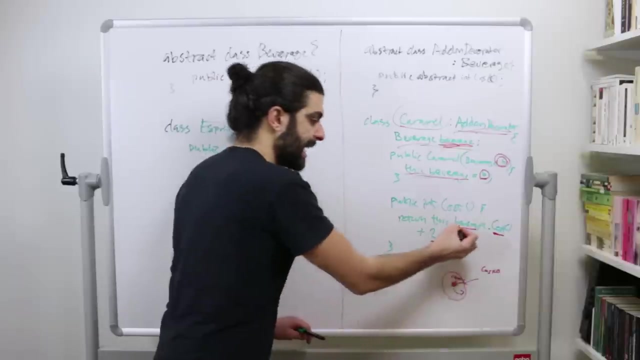 it's wrapping, let's say that that's the espresso beverage. it'll ask that for its cost. So we have the call to cost here, and we have the same call to cost here, but inwards, And then this espresso will return one. So one will go up here, but then the caramel decorator will take that cost and add to. 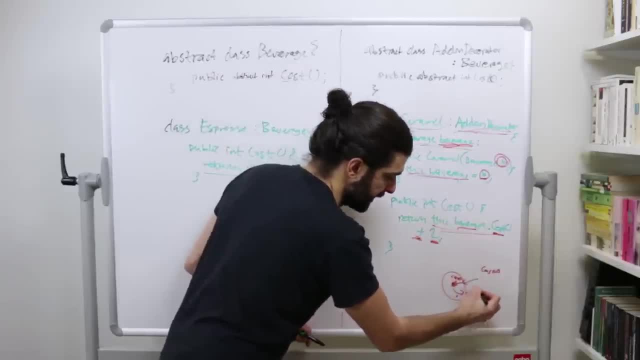 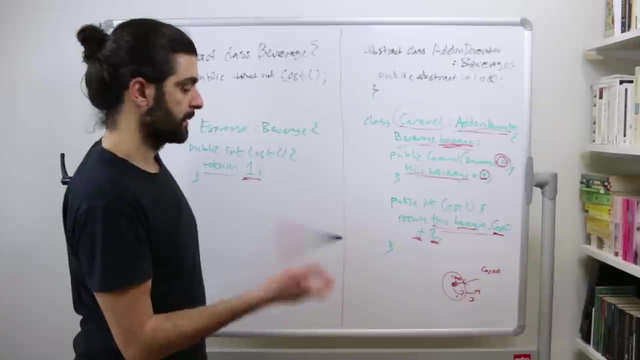 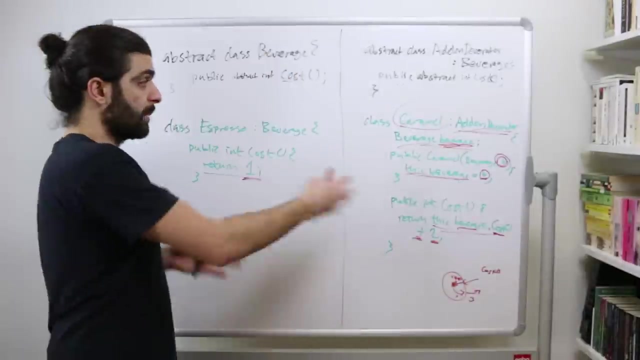 that another two. So here we get one, and then we'll get another two here, But of course it's two plus the one that we already have. So we get three out here, And that's essentially it. The methods that we have in all of these places are completely dependent upon your scenario And the number of 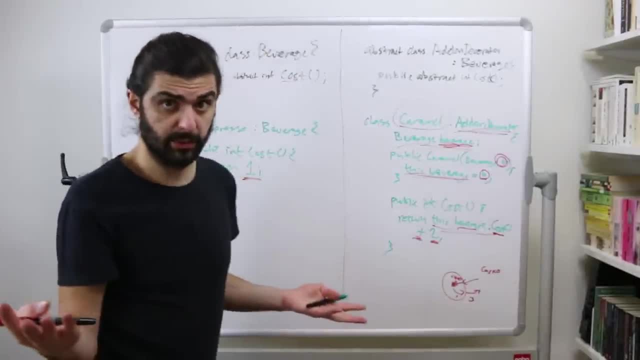 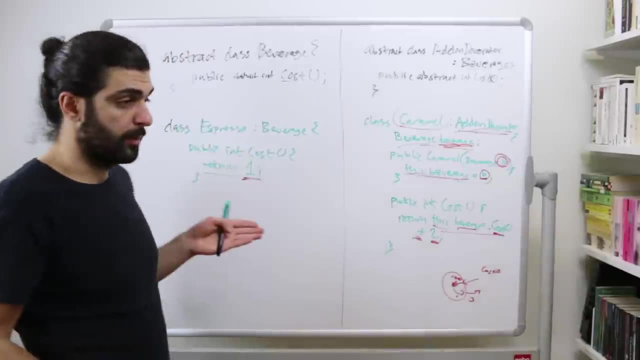 decorators and the number of components that you have are completely dependent on your scenario. So when we looked at the generalized UML diagram, we said decorator one and decorator two and we said concrete component. but you can have any number of concrete components and you could have any number. 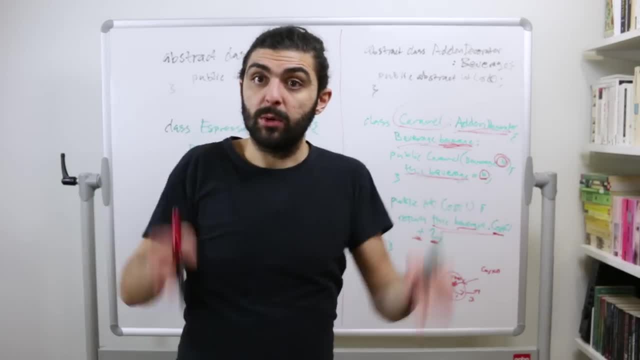 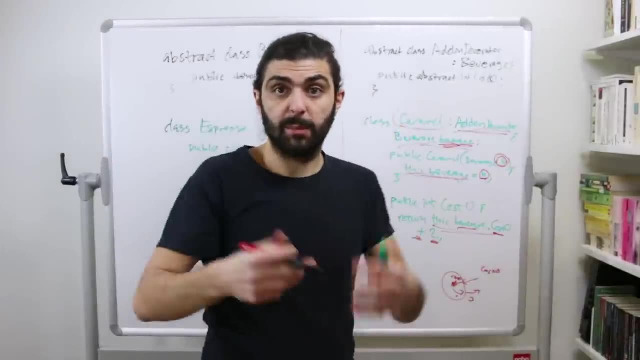 of concrete decorators. So that's sort of on the class level. And on the method level you could have any number of methods. So here we happen to talk about only cost, And in the earlier versions of this example we also talked about description. So the fact that all of these had descriptions- 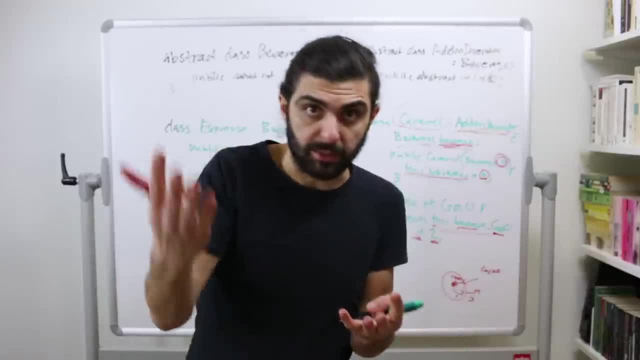 but you could have any number of methods And in the generalized we said method A and method B, And I also want to add that the generalization of the method A and method B is the same thing. So when I said that the decorator cannot calculate cost in and of itself, I mean 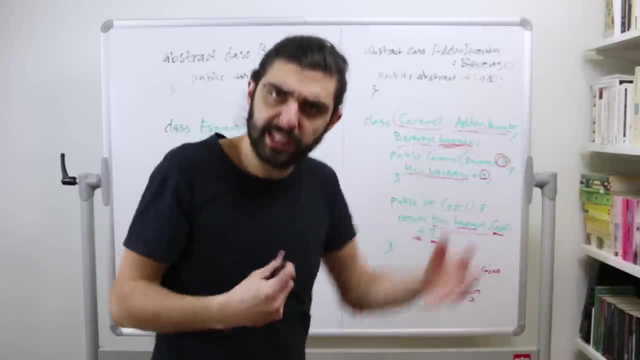 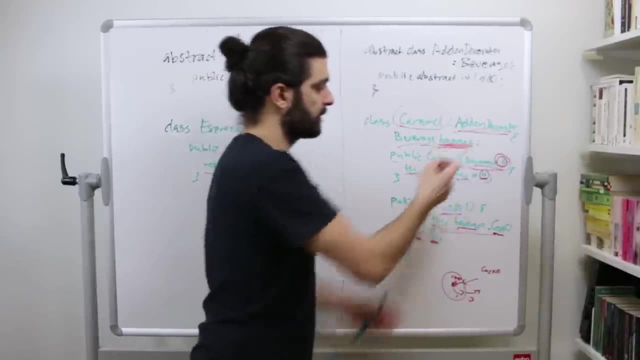 that's accurate, but it's also dependent on this scenario. So in this particular scenario, that's true. So when I say that the cost method here cannot be computed without also looking at the cost of the component that we have a reference to, in other words, without looking at the cost, 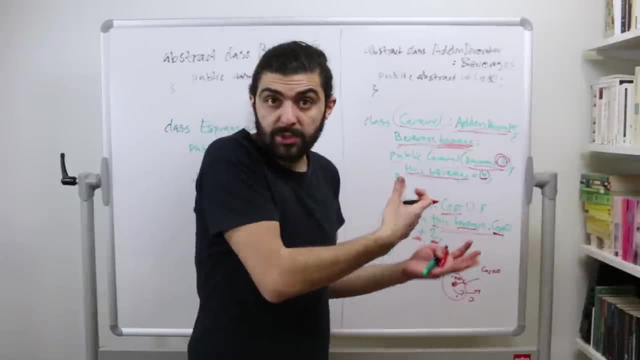 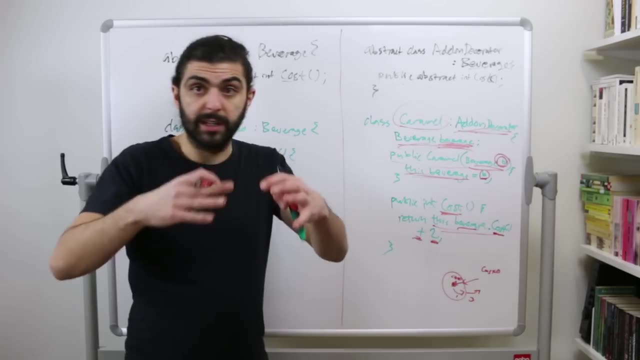 of the beverage that we have a reference to. that's dependent on the scenario. Generally, the cost method could, of course, calculate something without looking at what it decorates, So now we're leaving the whole context of a coffeehouse. So just generally, if you have, 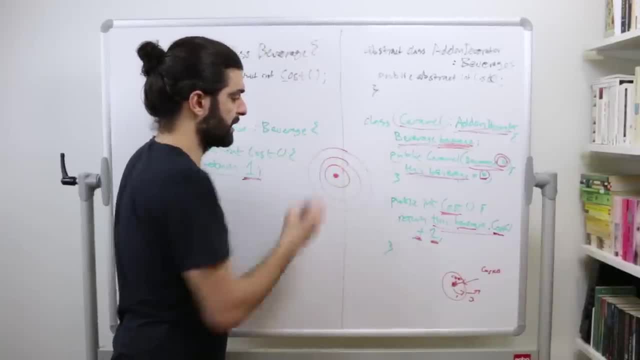 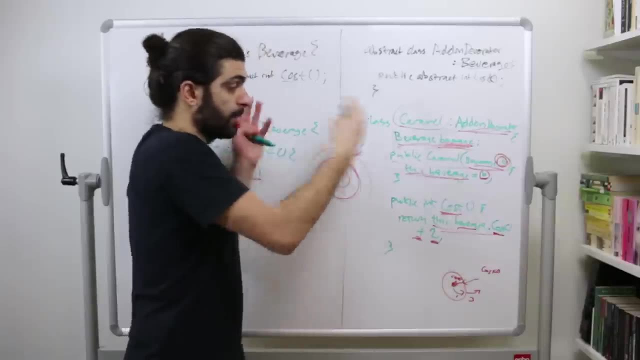 something that's decorated by something that's decorated by something that's decorated by something, and then perhaps this decorator is something like a reset decorator. So you make a method call to the outermost decorator for something and then that call is passed in and 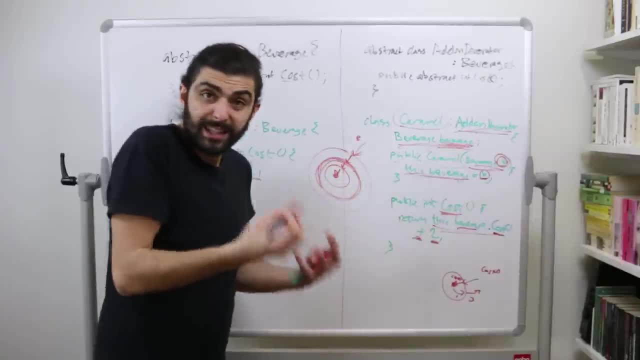 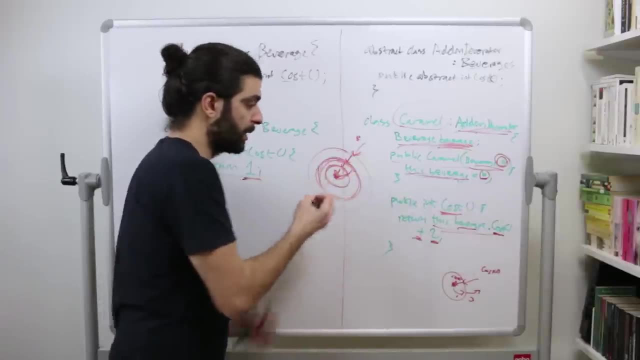 passed in and passed in, And perhaps this decorator completely ignores what's down here. It completely ignores what this decorator reports and thus, by proxy, completely ignores what the component or the decorator actually reports. So decorators can be used for tons of different things And if you want, 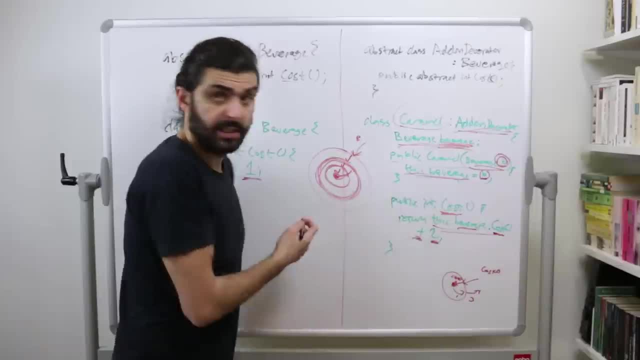 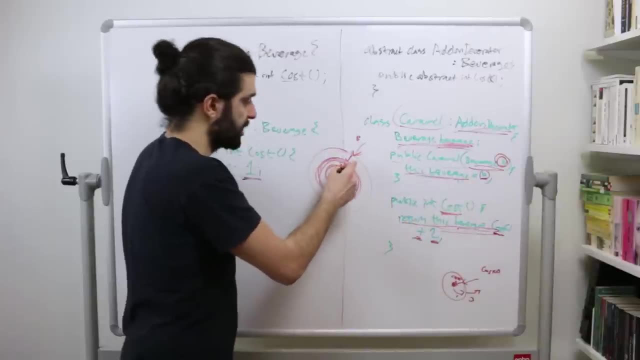 to think of it in terms of math. you can think of it as this thing multiplying by zero, for example. And if you would multiply by zero, then it doesn't even need to look at what's inside, It doesn't even need to further the chain of making calls downwards towards the component, because it's not going to. 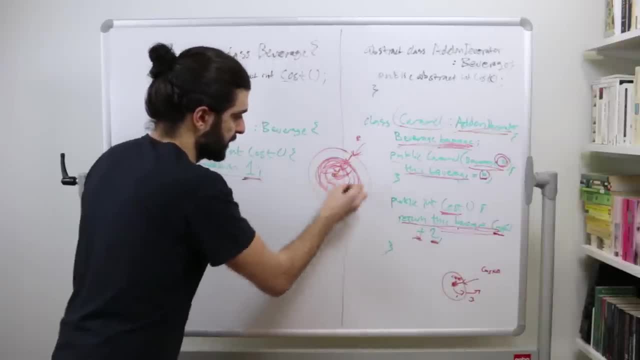 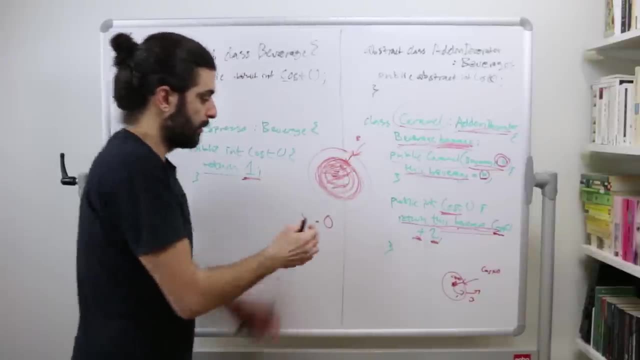 matter what's in here, because it's still going to take. let's say that what's in here. we call x. we don't need to compute x, because we're still going to multiply x by zero. when we get to this thing, we could just say return zero. So again, the implementation of the methods that you have. 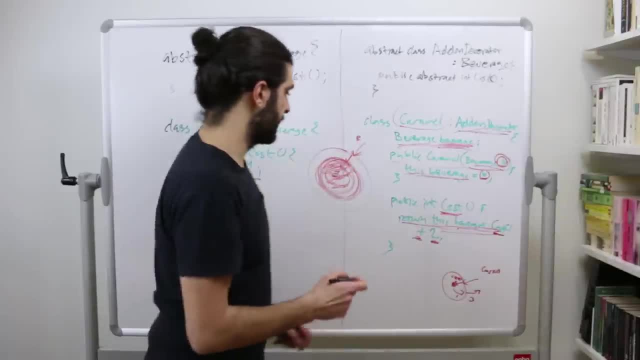 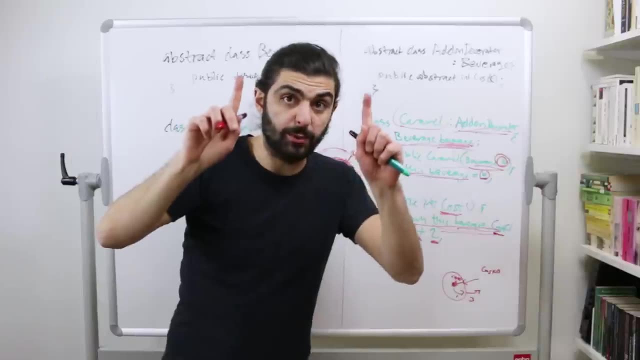 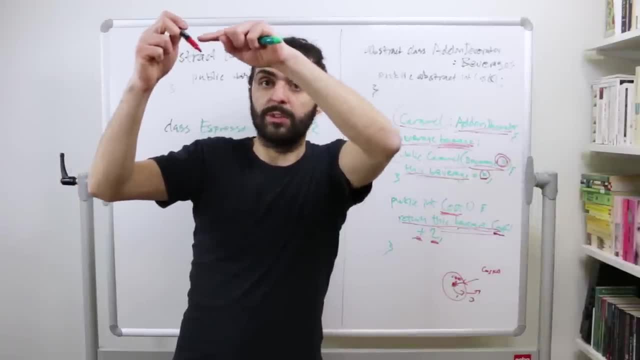 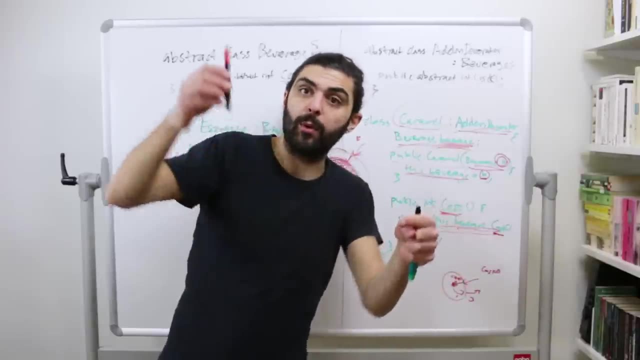 want. So you make a call to the thing in the outermost layer, that makes a call to the thing it's decorating, that makes a call to the thing it's decorating, that makes a call to the thing it's decorating, et cetera, And then the value propagates up all the way back. 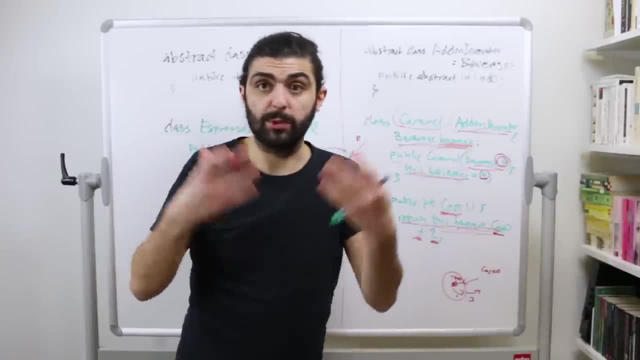 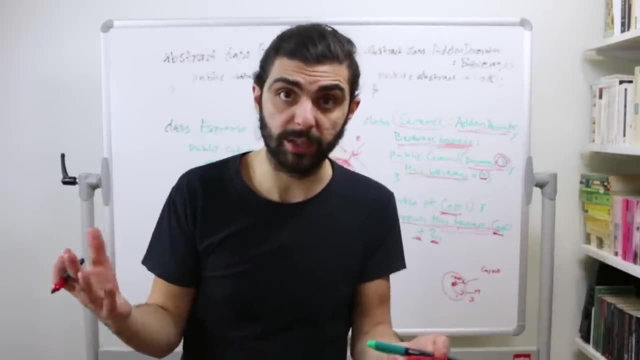 and then you have your value. But how that processing of the value or construction of the value happens again is completely dependent on your scenario, because it depends on what you're modeling and it depends on what kind of value you're actually looking for. So that's the 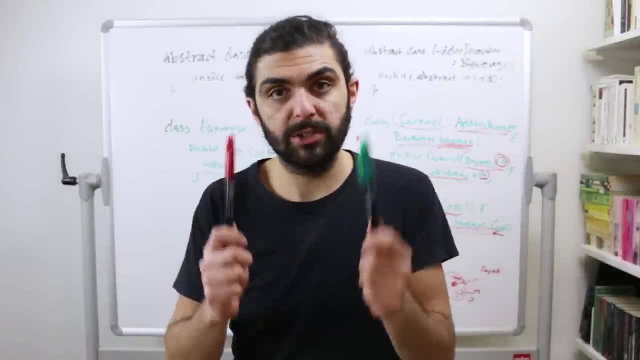 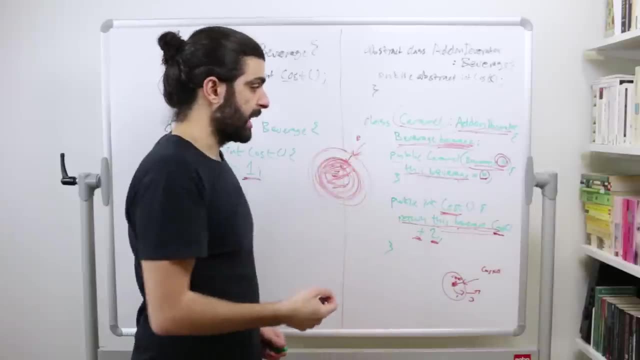 decorator pattern. Before we wrap up, I said before that I wanted to mention why I don't think that this particular example is actually suitable for the decorator pattern. So in my mind, what we're doing here is unnecessarily complicated for the problem that we're facing. A more suitable 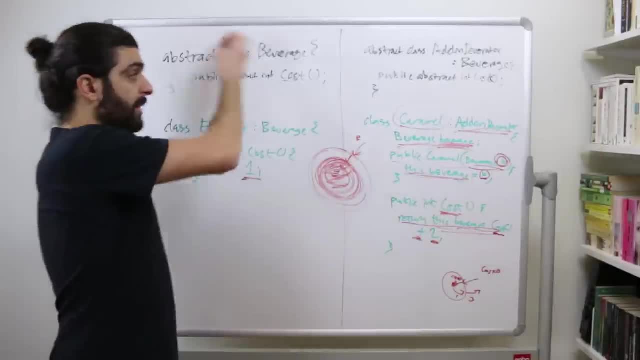 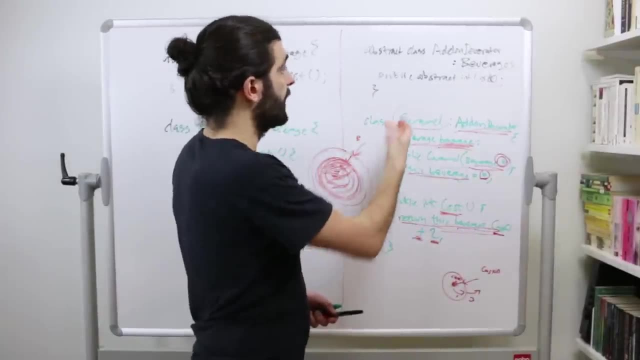 way of approaching this problem, I find, would be to have a beverage class, And in the beverage class, for example, via the constructor, you can pass it a bunch of condiments or, as we call them, add-ons or extras or flavors, And 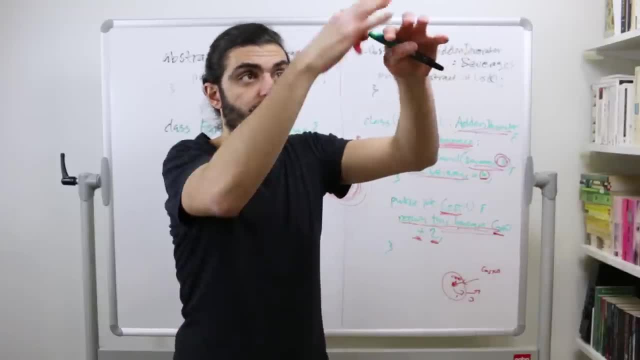 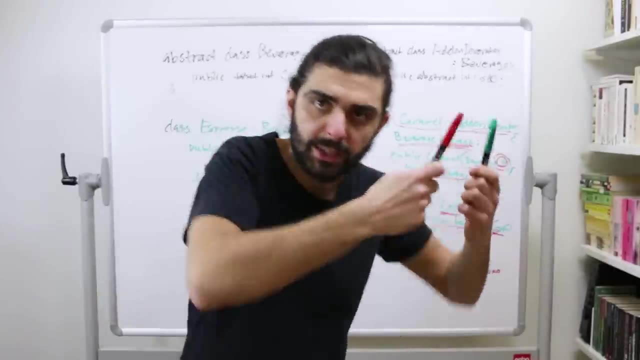 these are all of the same type. So you have flavors and then you have concrete flavors sharing the flavor interface or the flavor abstract class, or whichever way you want to design that. But the point is that you take these flavors and then you pass them into the beverage. 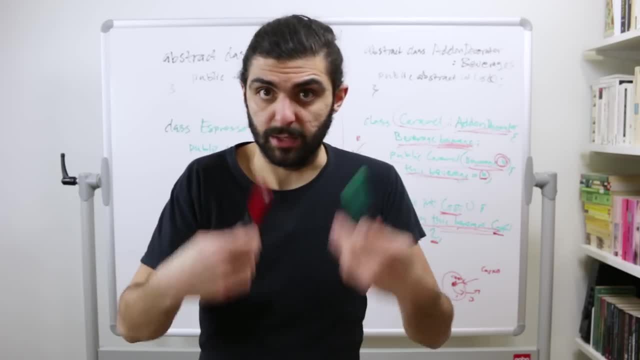 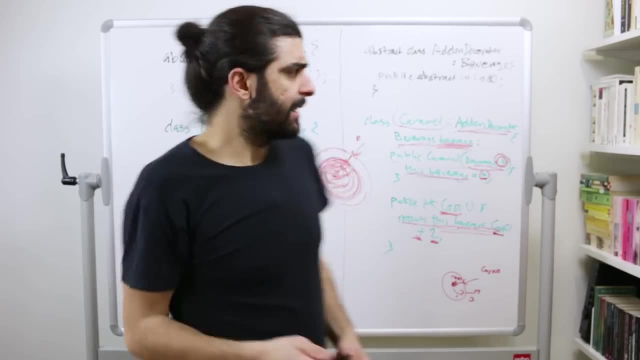 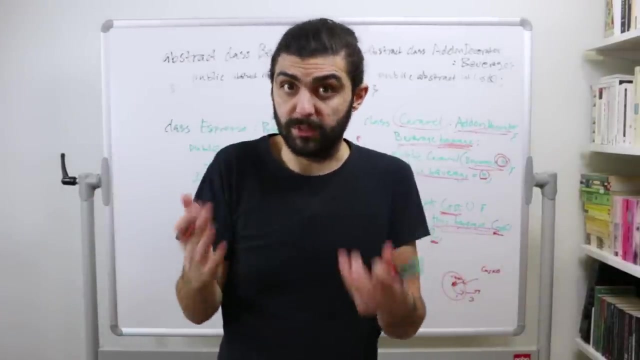 When you construct the beverage, in the constructor, you pass a list, array, list whatever: a collection of condiments, a collection of extras, a collection of condiments to the beverage, And then, when you ask for the cost, you simply aggregate, you simply iterate over the collection of extras and produce. 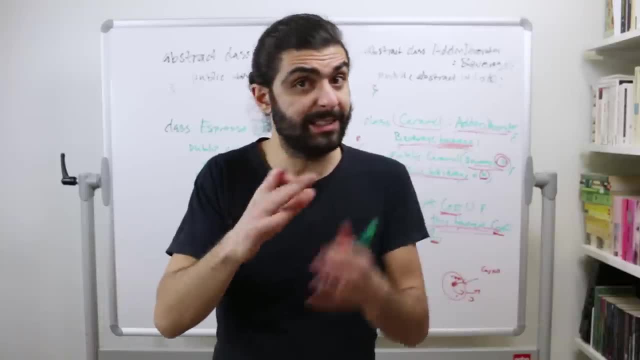 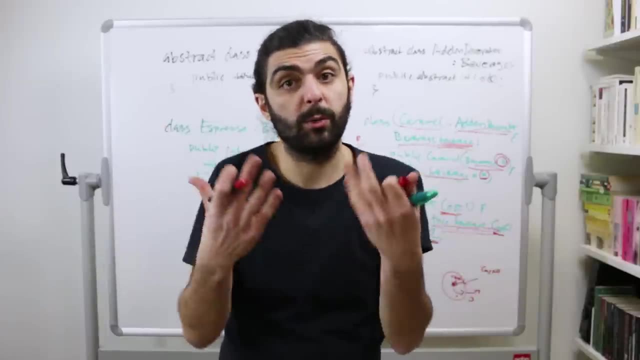 a value. When we talk about iterator pattern, for example, you'll see why that's actually a very useful strategy, because you're separating two different concerns. You're separating how to iterate over the collection, how to aggregate a value based on the collection and the actual. 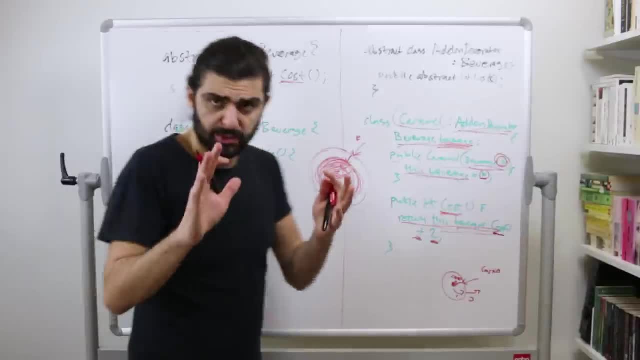 values of each of the items of the collection. So, for example, if you have a beverage, that's a little bit more expensive and you want to make it a little bit more expensive, and you want to make it a little bit more expensive. 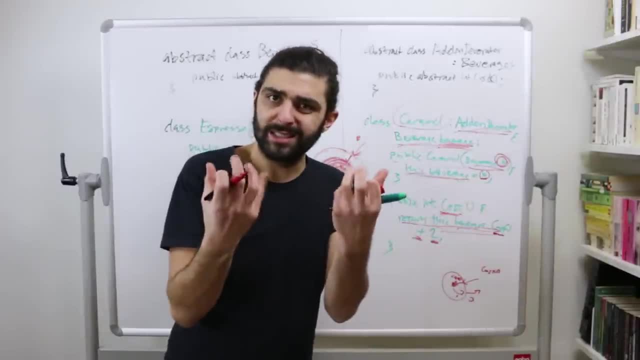 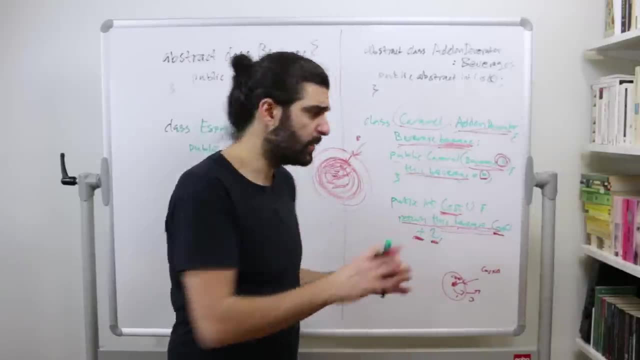 you're going to want to make it a little bit more expensive. So the reason I'm stressing this is that when we're using this for decorator pattern, we're actually mixing these two concerns. We're putting the plus here in each of the decorators, And what I'm arguing here is that that's unsuitable, because 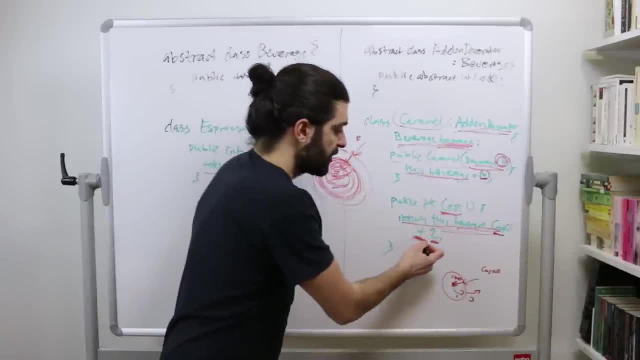 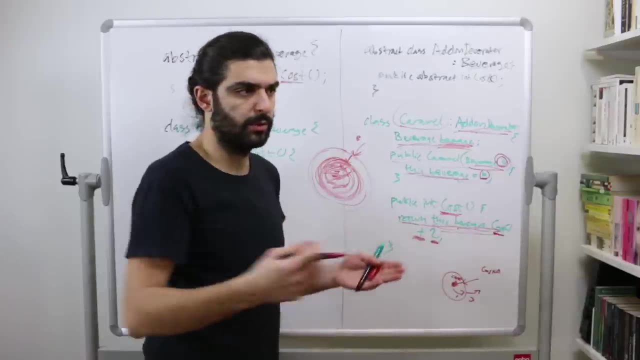 of the thing that we're building. It's unlikely that we'll want to change the plus to something else. It's unlikely that suddenly, if you introduce- I don't know, you put chocolate in your coffee, you want to double the price from before. That's unlikely. Of course you could argue that. 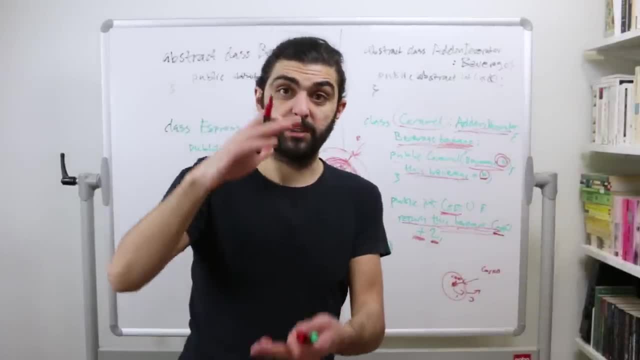 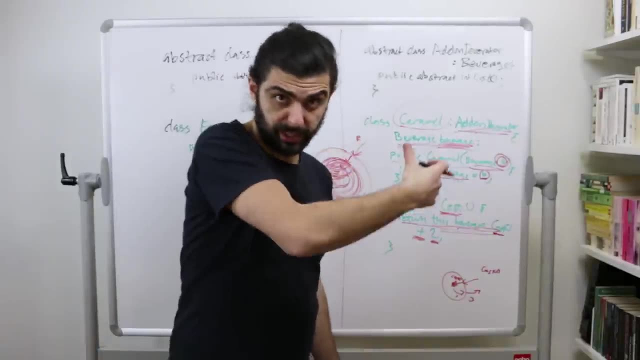 multiplying could become relevant. if you would look at things such as different sizes of cups, then it could actually be that the price is the same, but double if you have a larger cup. But again, I think this is totally overengineering. We would do much better with just a list and then 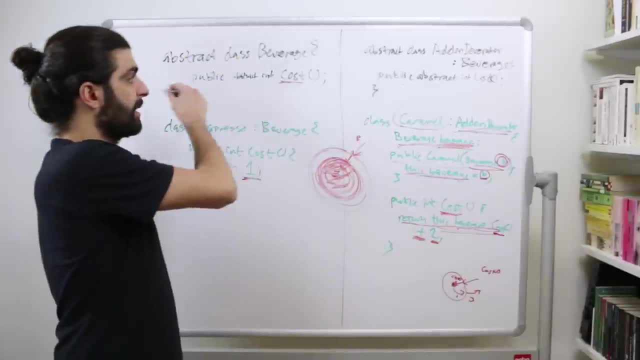 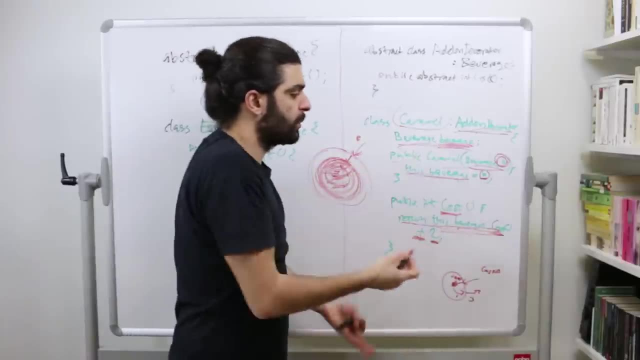 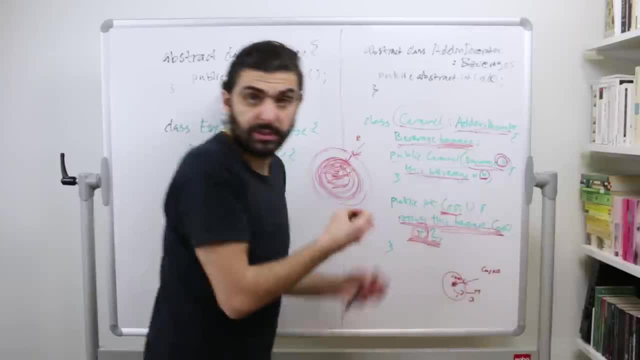 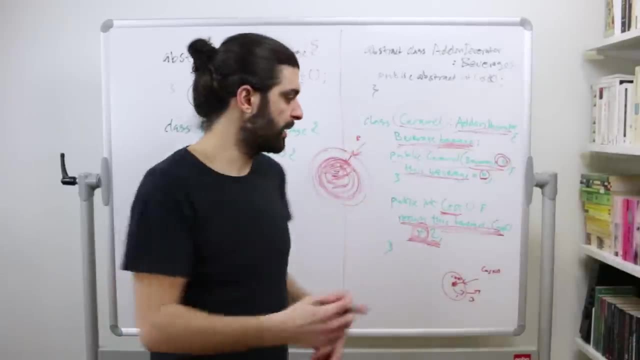 value and add that value to whatever was before. I'm arguing we're mixing two concerns here that shouldn't be mixed. I'm arguing we're mixing two concerns here that shouldn't be mixed And probably- if I try to generalize here- probably the problem lies in that the decorators 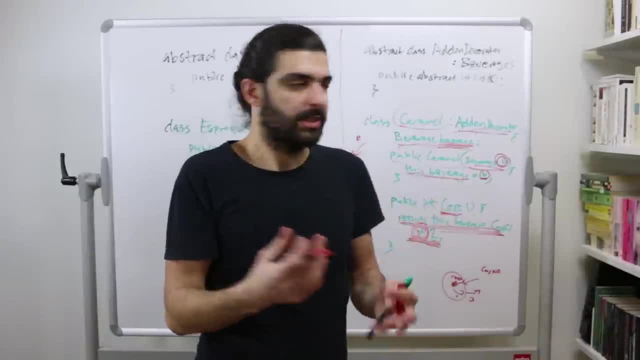 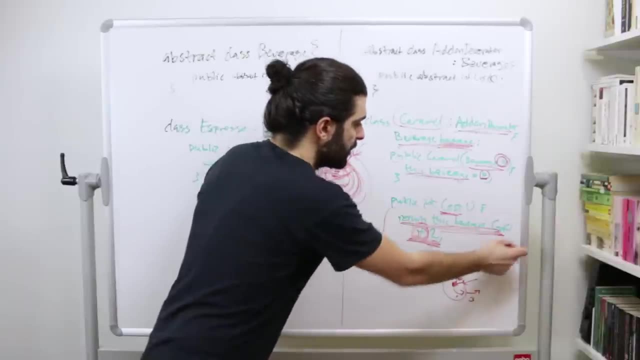 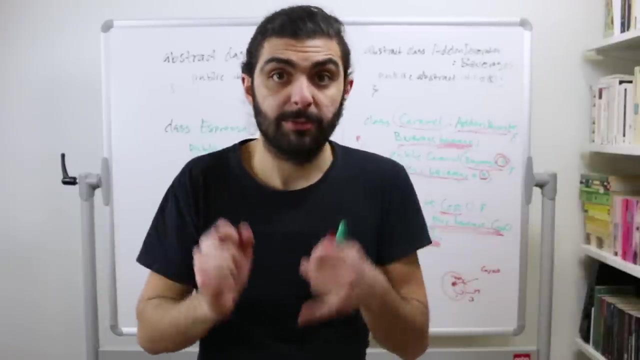 are too much alike. So we're looking at a scenario where it's unlikely for any decorator to be significantly different from another decorator. If the implementation of the cost method is significantly different between decorators, then I think you're looking at a scenario where it's actually potentially very useful to use decorator pattern. But 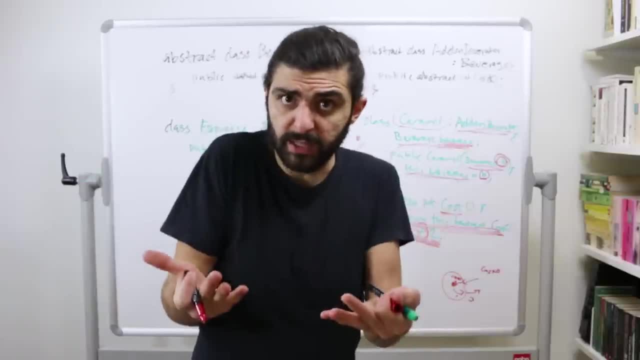 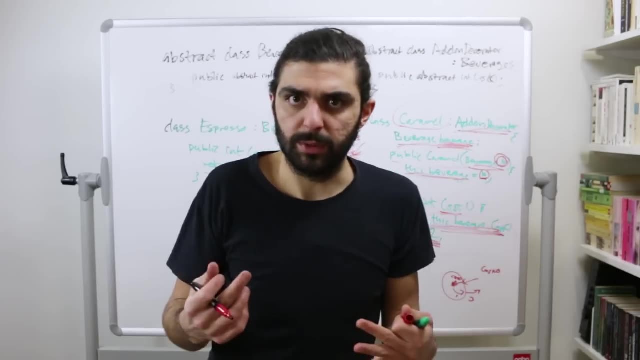 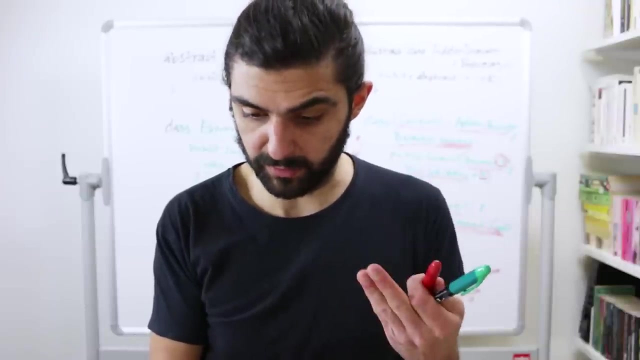 if what varies between these different decorators is a single property or multiple properties. essentially, if what varies is a property, then you're probably forcing in a pattern where it's not suitable. So the headfirst book actually has an example which is actually much more appropriate, which is from the Java API. So if you're in Java, you perhaps recognize the 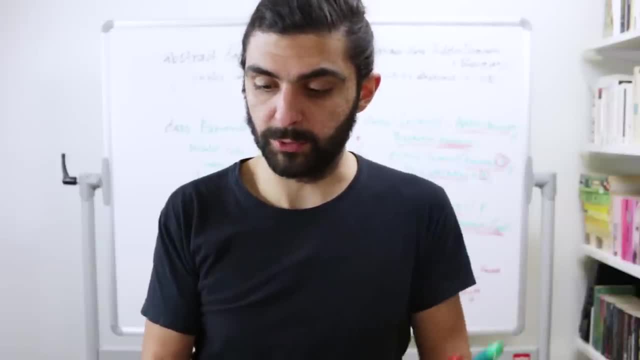 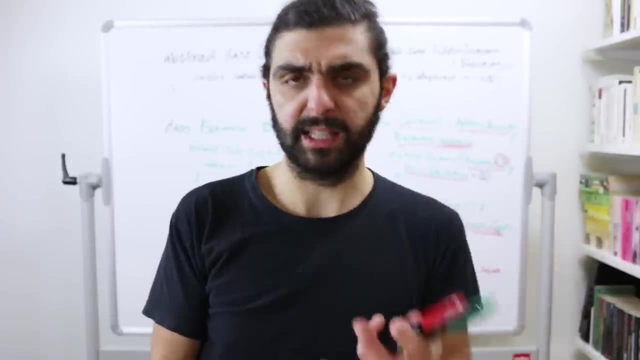 concept of an input stream. So you have an input stream which could, for example, be a file input stream, So if you're streaming from a file, you're reading the contents of a file from disk, and then you can decorate that file input stream with, for example, a buffered input stream with. 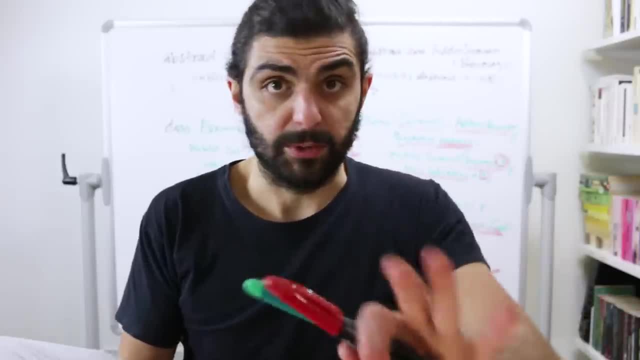 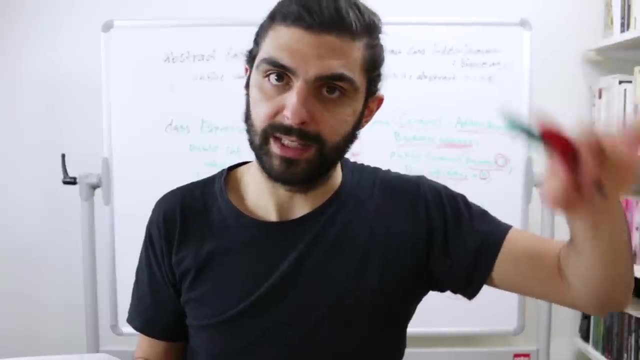 for example, a line number input stream, et cetera, et cetera. I mean, I'm not familiar with this API, but just by reading these names I'm trying to guess what they're doing. So the buffered input stream would probably help you. buffer, in other words, read in chunks, So you 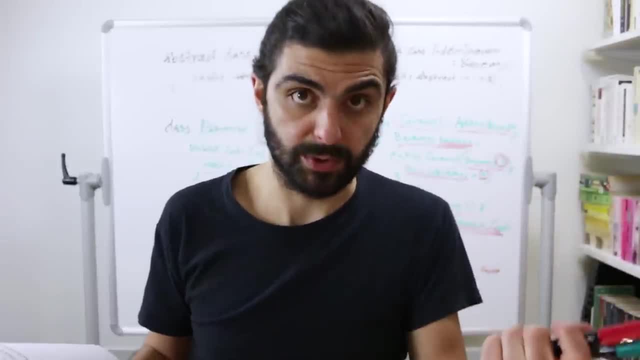 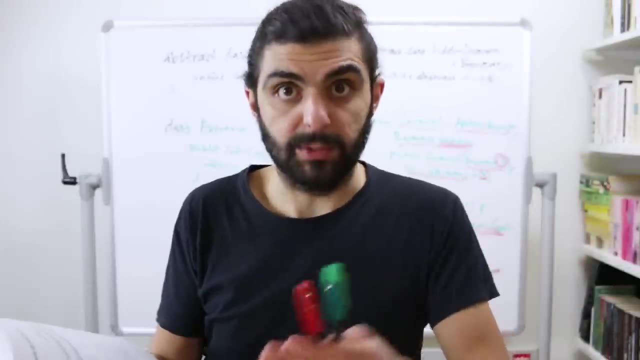 take a buffered input stream and then you wrap that around an input stream And then perhaps you would take a line number input stream, which I guess helps you to get the line numbers as you're reading. So, for example, you construct a line number input stream and wrap that around. 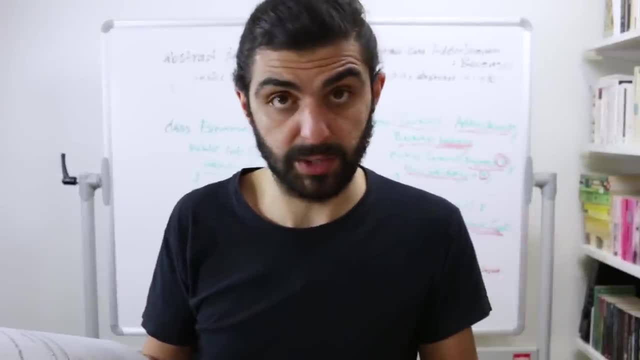 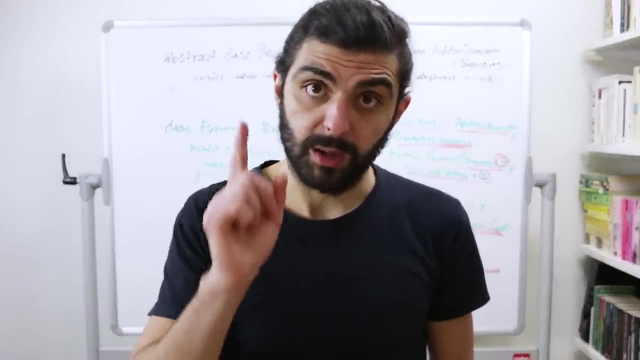 the buffered input stream that's wrapped around a file input stream. So to me that sounds a lot more sensible, And I think for two reasons. One, because we're talking about streams, So the decorator has a name that resembles the thing we're decorating. 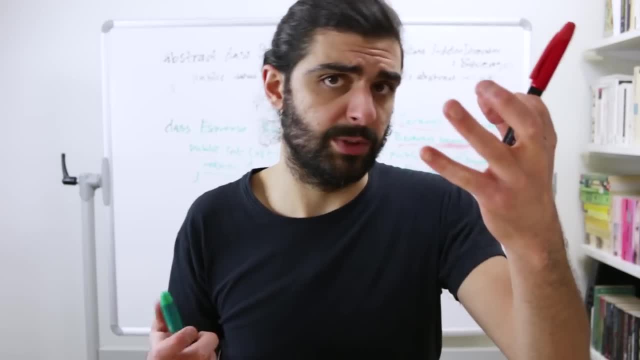 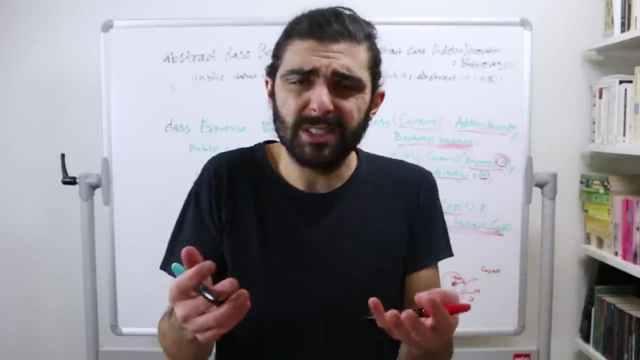 The decorator is named stream and the thing we're decorating is also named stream, Whereas, if you think about what we've been doing, we've been saying that condiments add-ons are beverages, but obviously they're not, And that's one of the reasons I think this is actually kind of 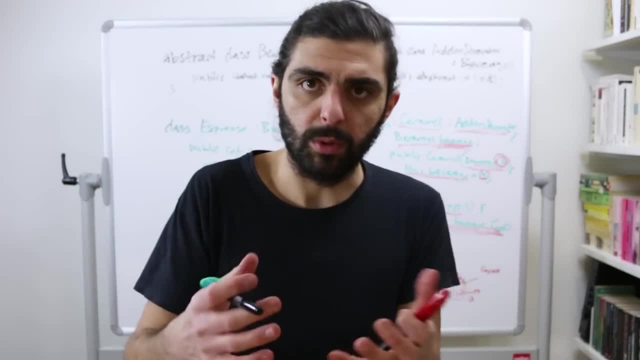 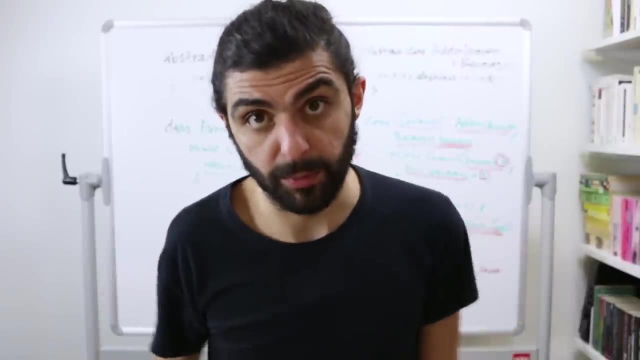 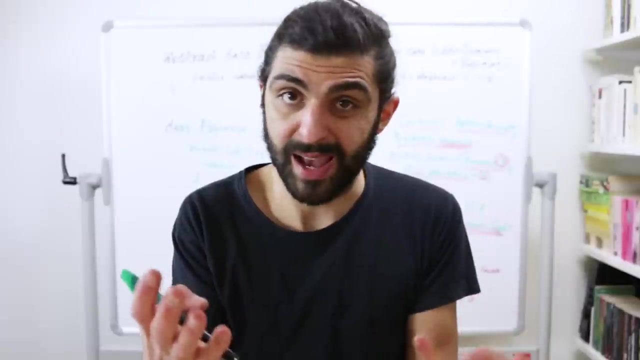 a strange example, because decorator pattern is probably more suitable when your decorators actually very much are what they're decorating. But again, the second point is probably a lot more important, And that was that the differences between these different decorators is so insignificant that decorator pattern is simply not probably sensible If the only variation is. 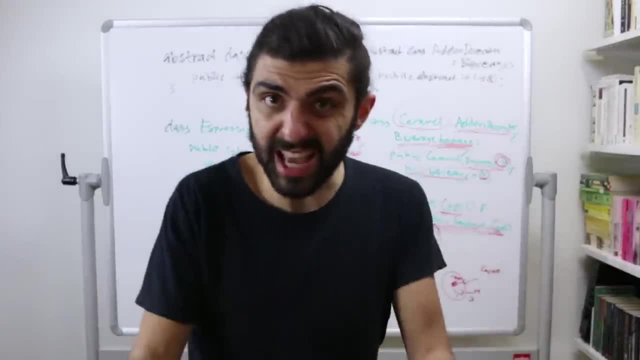 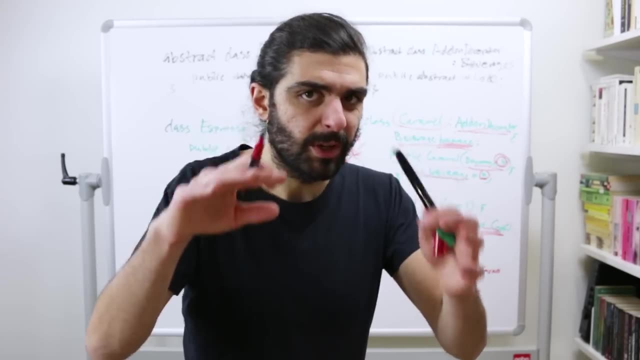 the actual cost and when we have more stuff, the name of the decorator, in other words the name of the add-on or the name of the condiment, as in like, is it whipped cream- Then those are sort of on the property level and not on the behavior level, I think. 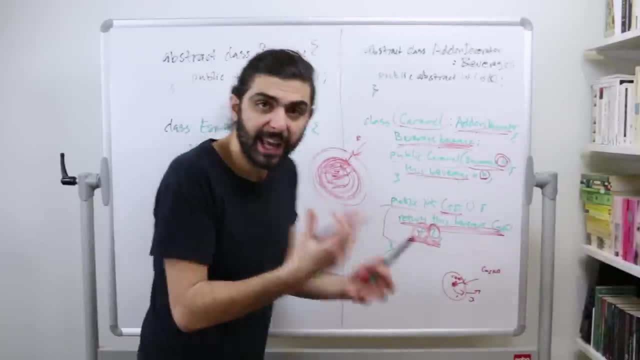 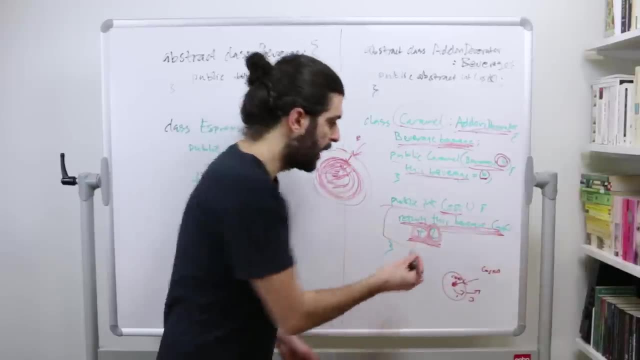 decorator pattern is probably more suitable when we're looking for behavioral variation. We're not looking for variations in that here we have a two and in the other one we have a three. That's not a behavioral variation. We're actually looking for variation in this plus. That's when 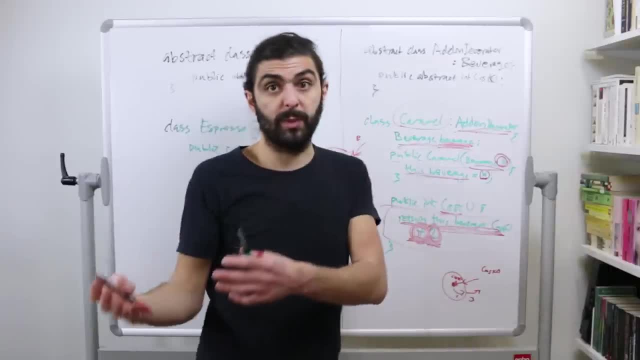 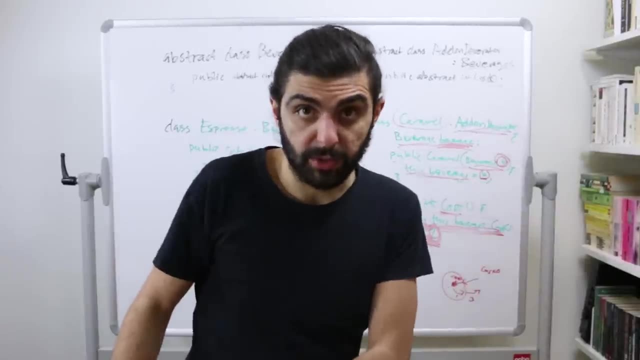 decorator pattern is more useful When in some of the decorators you want to use plus and in some of the decorators you want to use minus, For example, probably math isn't suitable either, because order matters. But just again, think of the input stream example, When behavior is. 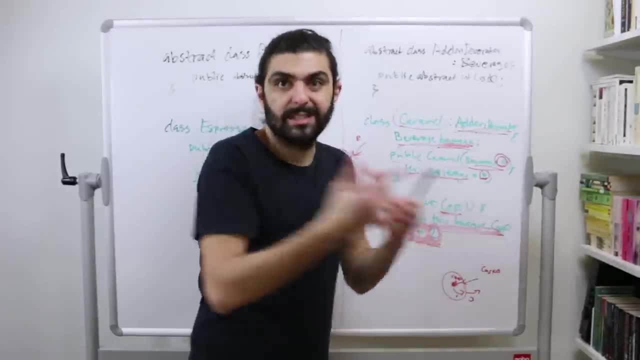 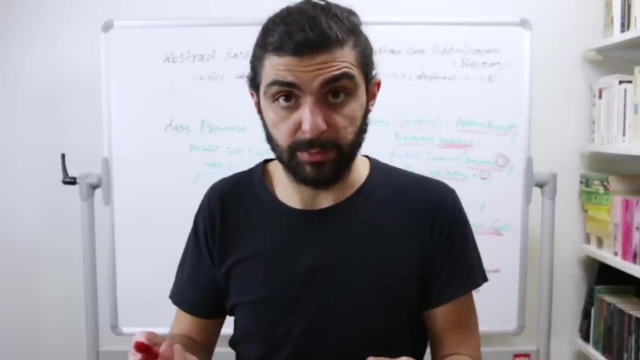 significantly different between the different decorators. Same method in the different decorators. So a very small example of when I've actually used something that looks a bit like decorator pattern in actual production source code is when I'm trying to deprecate something but I don't want to deprecate it in all of the places at once. So 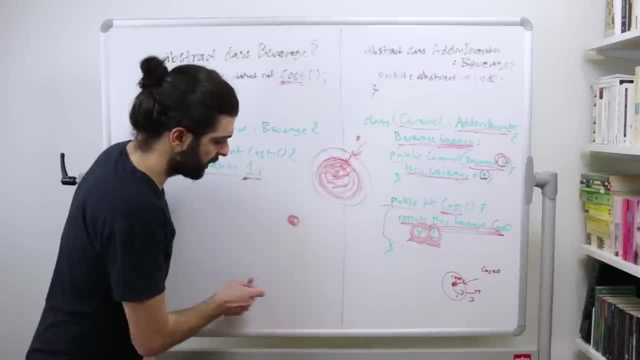 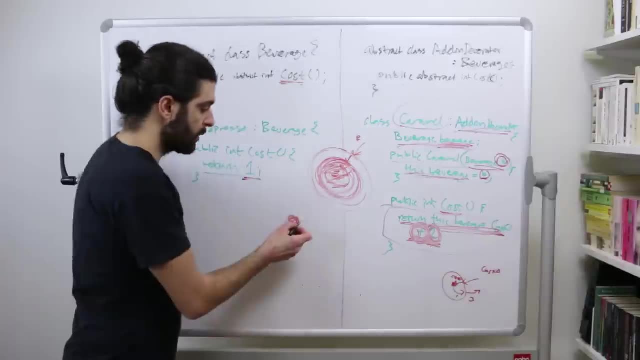 assume, I have this object, I have this class and it's used in a bunch of different places and I want to stop using this particular class, But for some reason I don't dare to change it at all places at once. So I'll create a wrapper, I'll create a decorator that decorates this thing and somehow 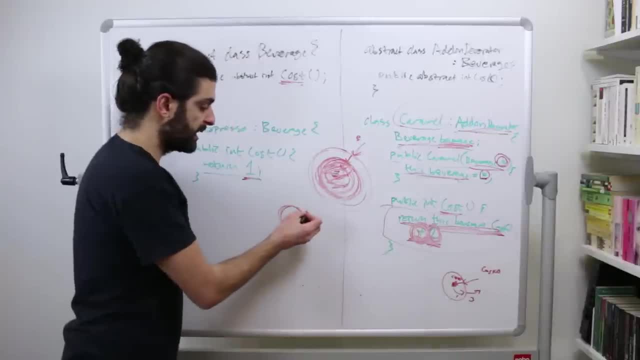 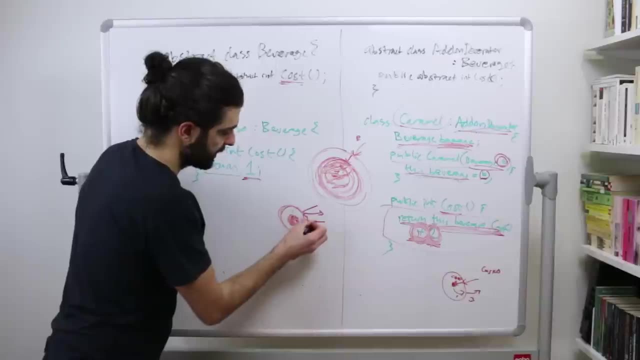 it accepts the operation here. So for some of the methods that I may want to deprecate, instead of making the call to the thing here, I just ignore making that call and let the decorator return a value. Or I, for example, do make the call but then somehow augment the value. So that means 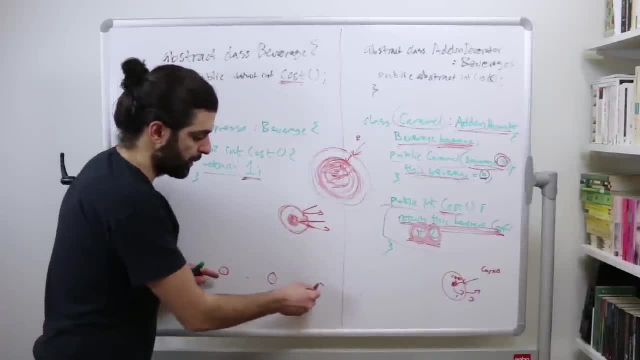 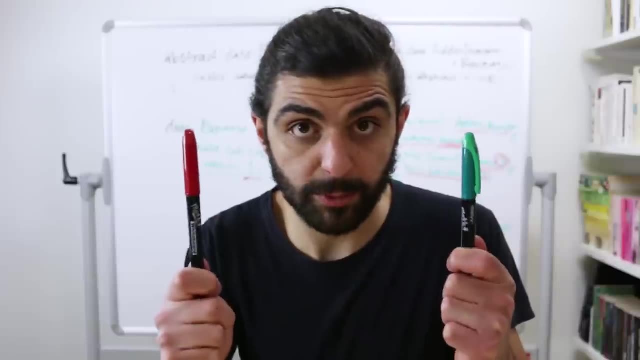 that I can use the decorator version in some places where I'm ready to change it, and I can use a non-decorated version in other places. So that just makes deprecation easier. So last thing, before we close this thing about decorator pattern: I forgot to actually show how we would use this. 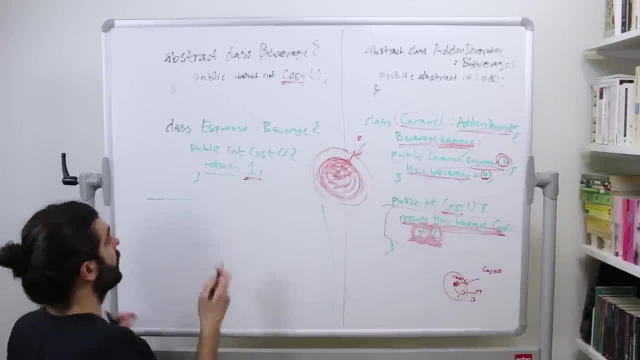 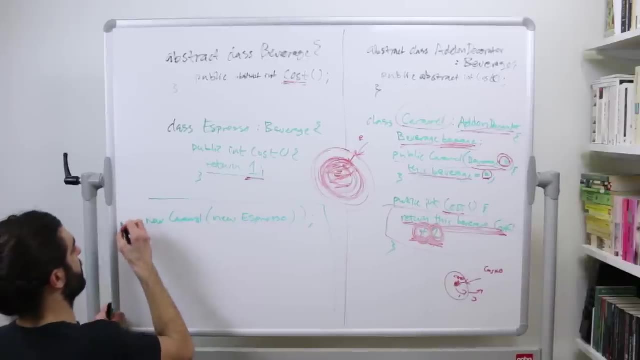 So how would we go about creating a caramel decorated espresso? What we would do is that we would say new caramel and in the constructor we pass a new espresso, And then we can save this into some variables. let's say, beverage b equals part of the double lines, And then if we call 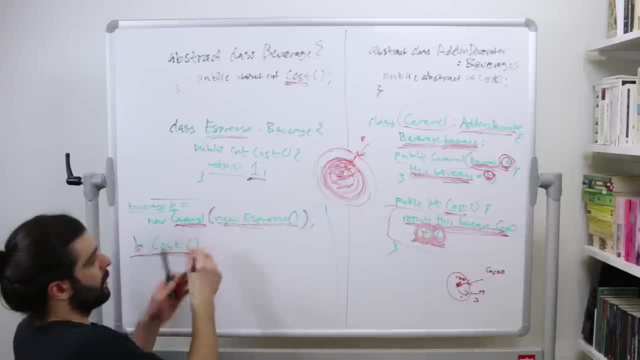 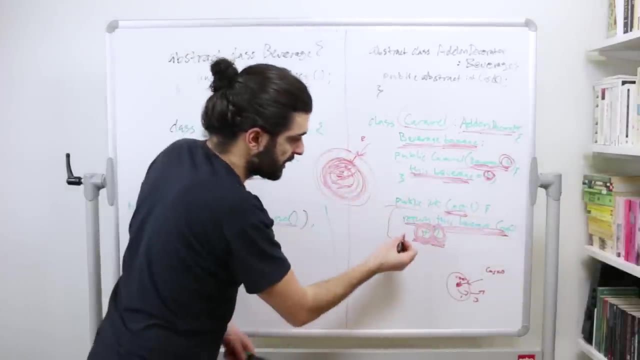 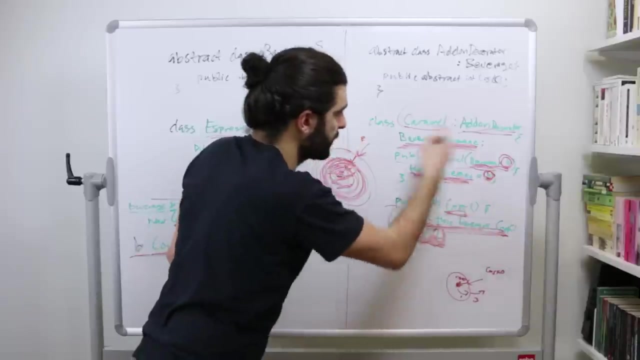 bcost. where we end up first is that because it's on the outer level, because it's a caramel class, because it's a caramel decorated, we end up here in the cost method. So when we call cost here, we get bcost. In other words, we can't do plus two first. We first need to look at the beverage. 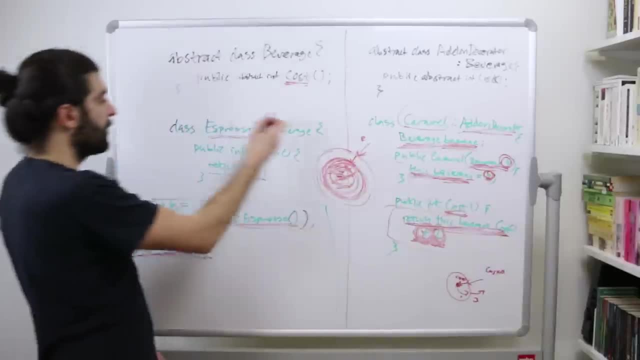 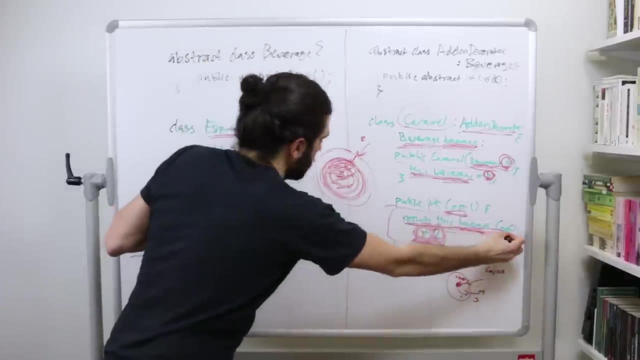 that I have as a decorator here, the beverage that I'm decorating. So we go into that beverage which happens to be an espresso, which happens to be this class, and we call the cost method here right, The beveragecost, We call this cost method, and then that cost method happens to return one. 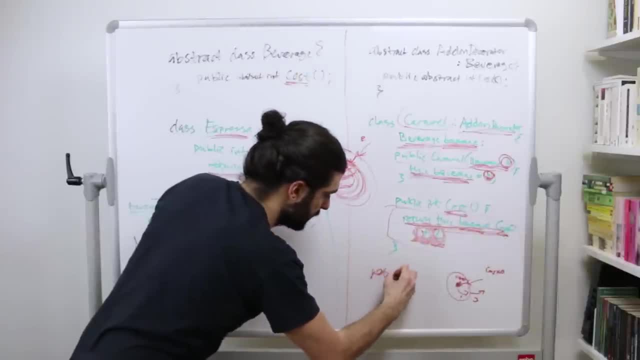 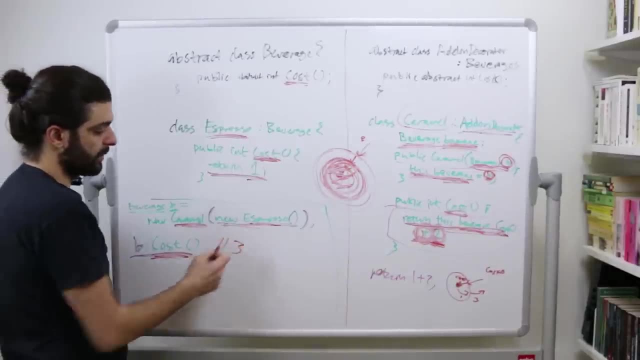 So here we'll get one, and then we add two to that, So we get in essence return one plus two, because we add two to it And then we're back here and then this line then essentially equates to three. And of course, if we had multiple decorators,